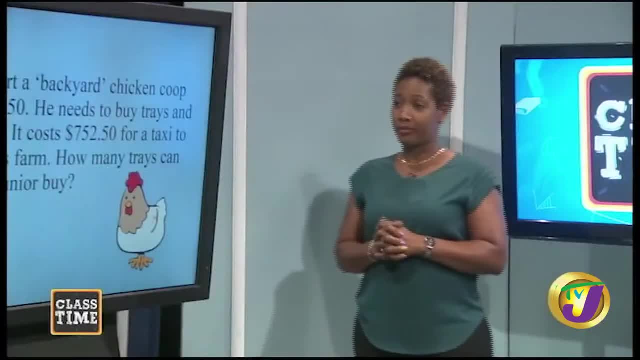 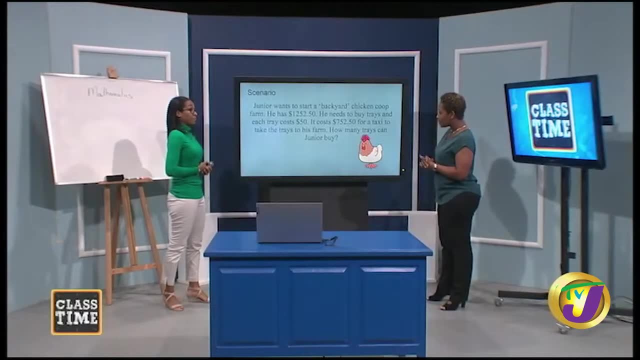 Well, at least him have some money. So let's see. But him still have a problem. because he has money. yes, Needs the trays because without the trays the farm not going to work. So he has to figure out what is we need to figure. 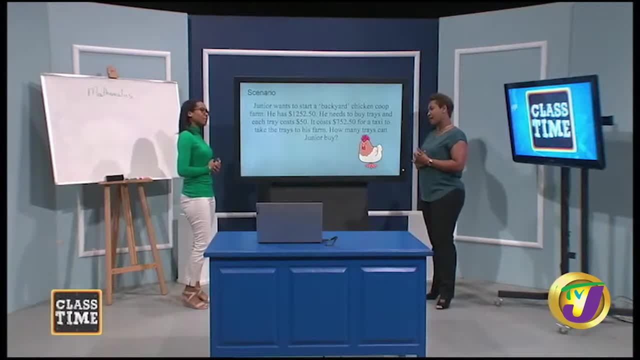 out how many trays he can buy. But in figuring, figuring out how many trays he can buy, don't we need to know some things? Well, they told us the cost of the tray. I know how much, how much money he has. That's all I need to know. No, man, but I think you know, we know he has a problem. We need 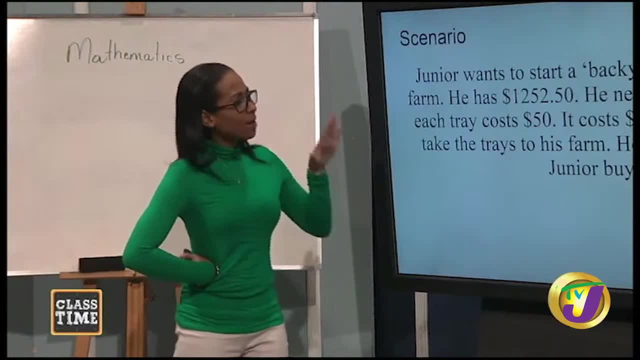 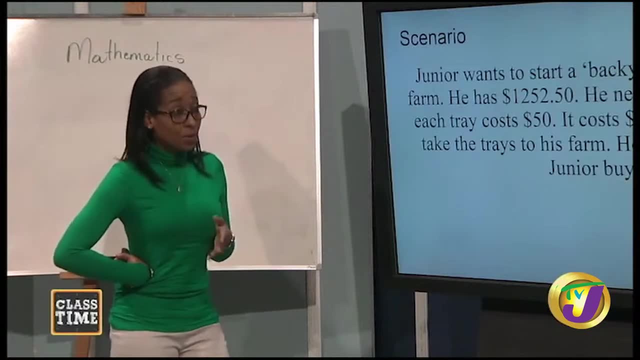 to understand what the problem is. So in understanding what the problem is here, you would have rightly said: he has some money, He has some money. So we know he has some money And he knows how much to buy, how much to pay for. 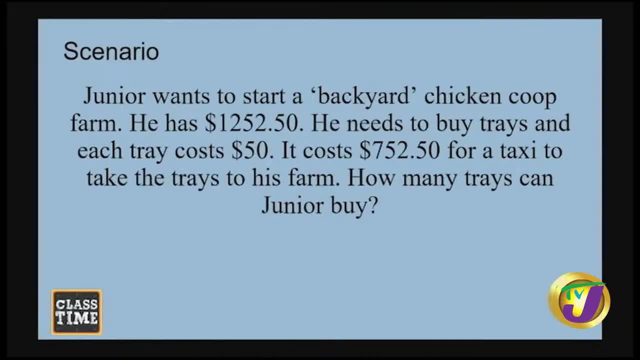 each tray Right. So he has some money. He needs to buy some trays And guess what? He knows how much. or he knows the cost of each tray, Most definitely What else he knows. Look again at the scenario. Well, you certainly need to understand- There's another figure in there- that 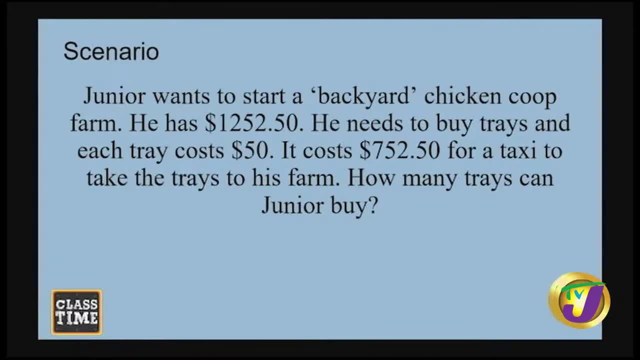 was introduced. You need to understand that man. he has to pay all of his debts, In fact the price of all his taxes. we all know that he has to pay $52.50 for a taxi to and $50.00 for a taxi He. 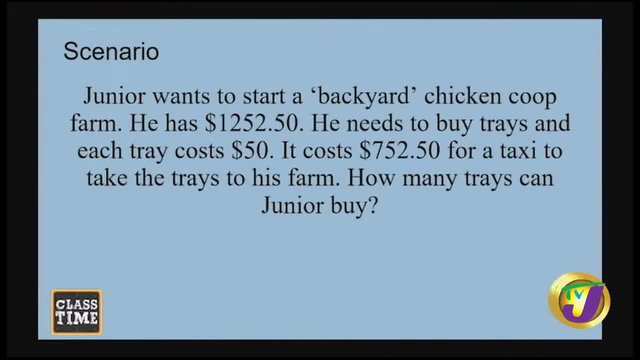 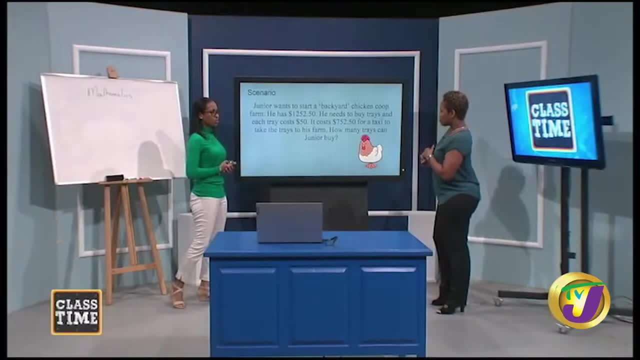 needs to pay all of his taxes. He needs to pay $52.50 for a taxi to Oh. he needs to get the trays to the farm. Gold, That has to be. that's a part of understanding his problem. Okay, So he has to. 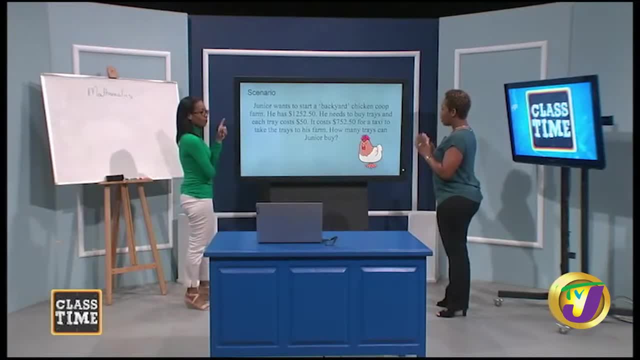 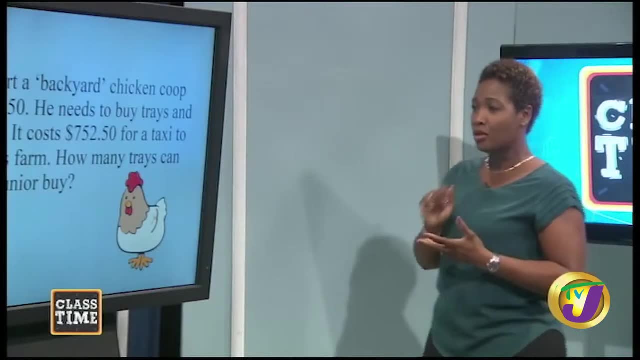 So he needs to figure it out, don't he? Yeah, man, he needs to make a plan to figure out how he's going to start the coop by getting these trays. So he needs to buy the trays and get them to the farm. 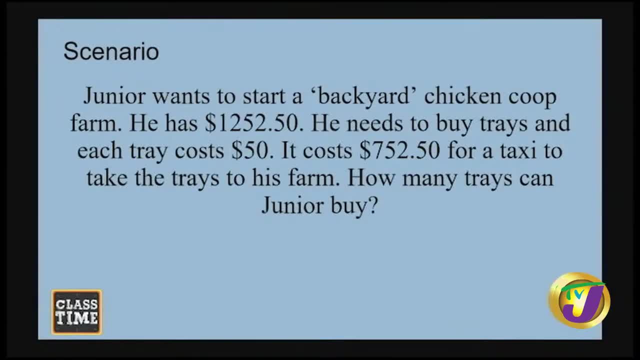 So he has to make a plan in order to figure this out And when he makes the plan, guess what is going to happen or what will take place. So he understands that he'll have a problem, he'll plan it. then He can work out this plan and end up with a solution. man. 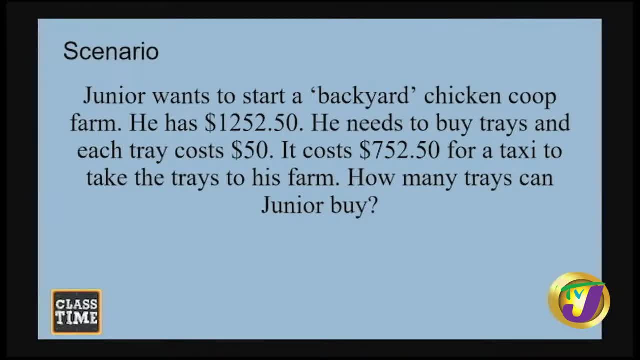 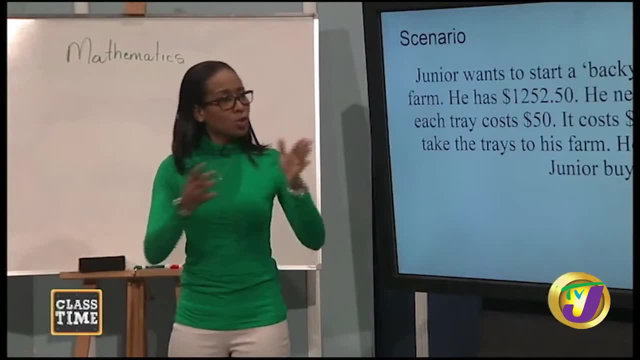 Good, so he's going to solve the problem, Of course, because after you plan, you can solve Great and in him solving the problem when he now knows that he needs so much trays to purchase Or he can afford so much trays. 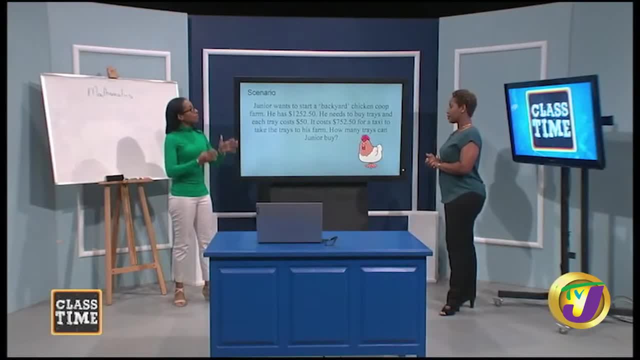 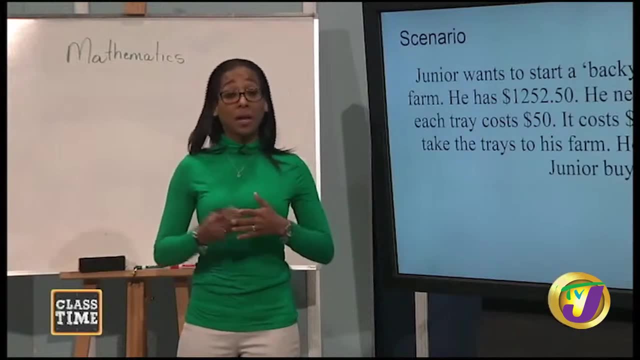 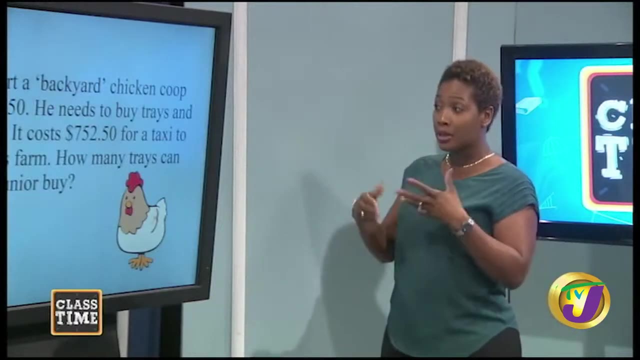 Right, based on how much money he has Right. So, based on how many trays he would have now ended up with, he would have realized: all right, as you rightly said, I can afford it, I can't afford it. But if he plans well, he can see the money, that he will realize that the money he has can pay for everything. 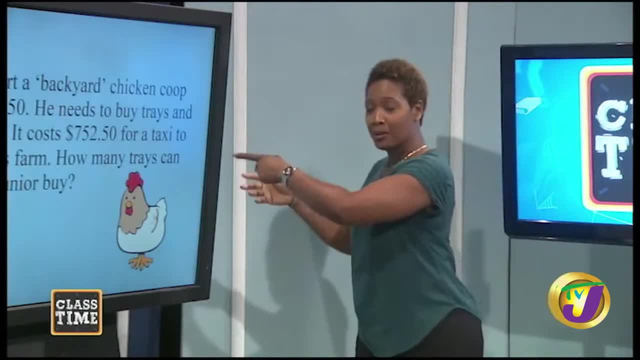 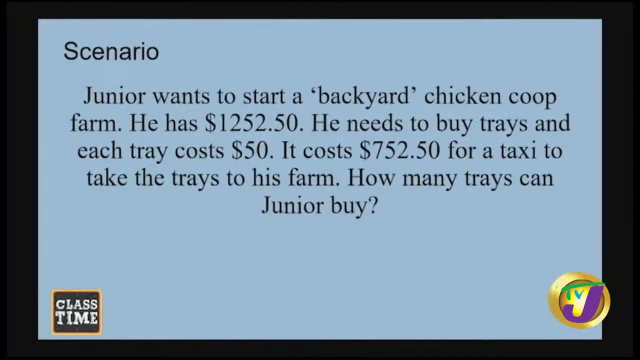 X amount of trays and also the transportation costs because he has to pay that taxi. So with understanding this problem, planning how he's going to use his money, planning how to solve this problem, he can come up with a viable solution. And then at the end, before he even executes everything or after he figures out the solution, 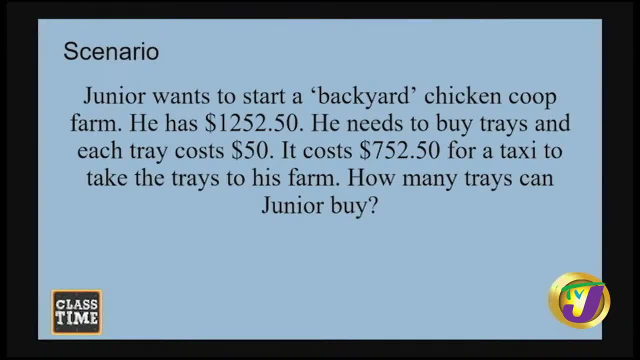 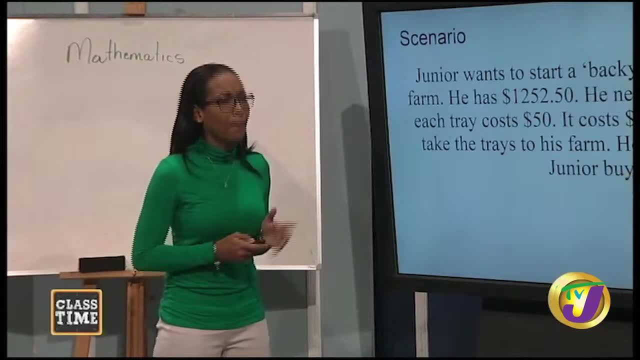 He can definitely check if everything works out. If everything works out, Yes, What do you think we really looked at here? Because we started out with Junior Junior having a what again? He had a problem. Great, So he had a problem. 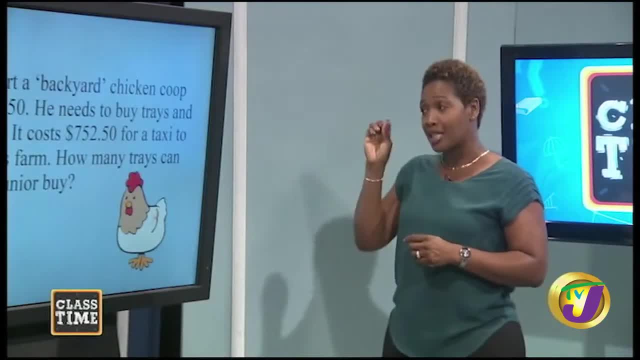 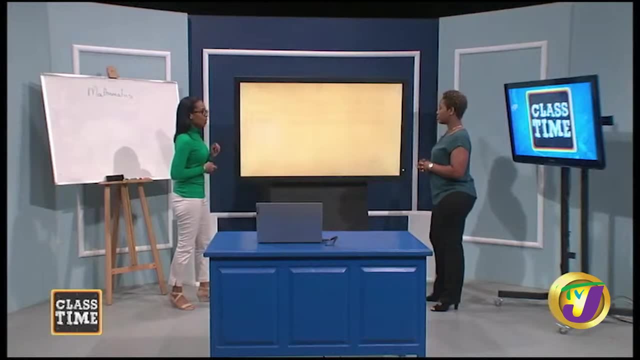 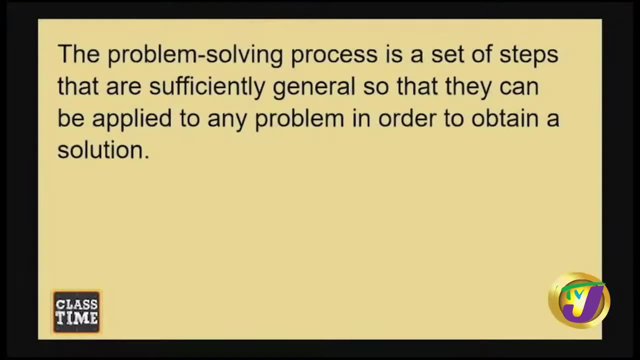 He wanted that chicken coop and he had X amount of money. He had a specific amount of money to get some trays. So we're just going to put it now in writing. So here we know that we're looking at problem solving And we would have spoken about a process that entails in Junior having a problem and such. 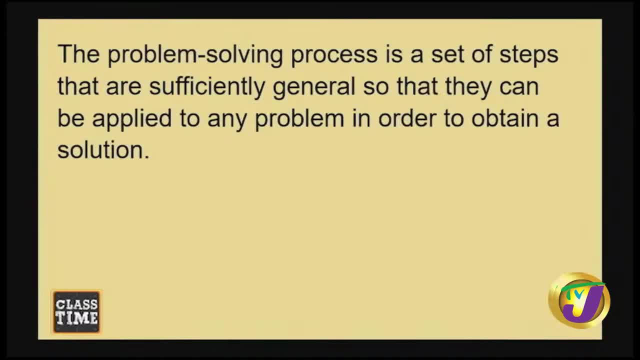 So here goes. So the problem solving process is a set of steps that are sufficiently general, Sufficiently general so that they can be applied to any problem in order to obtain a solution Before you even move on. when you say sufficiently general, what do you mean? 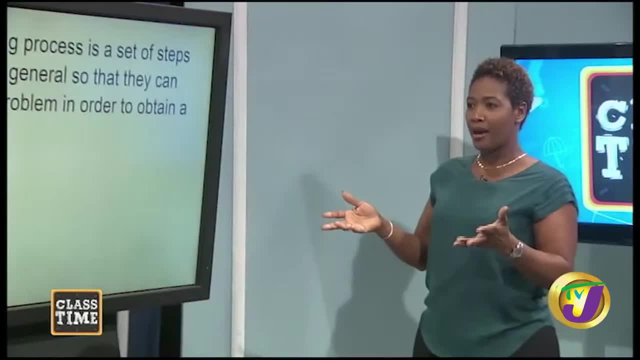 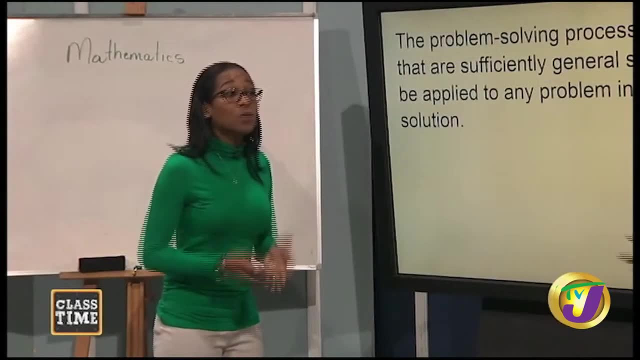 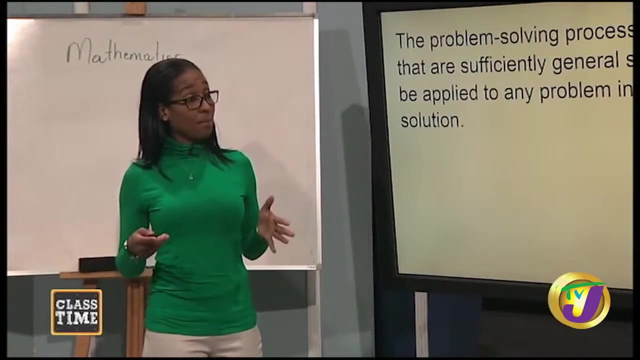 I can apply this not only to Junior's problem, but to any other problem I have Right. No, no, you're thinking So to any other problem, because guess what A problem is? a problem Got you. So in figuring out that problem, there's a process that takes place in really solving that problem. 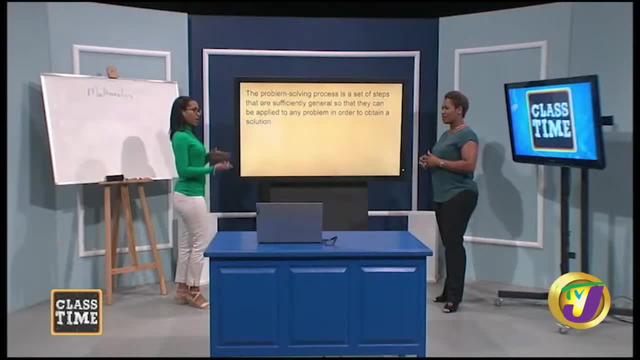 Well, that makes sense. Yes, and we would have spoken about the process, but we're just formalizing it Because one we realized that we had to understand the problem first. Of course, we had to look at all the information that was given. 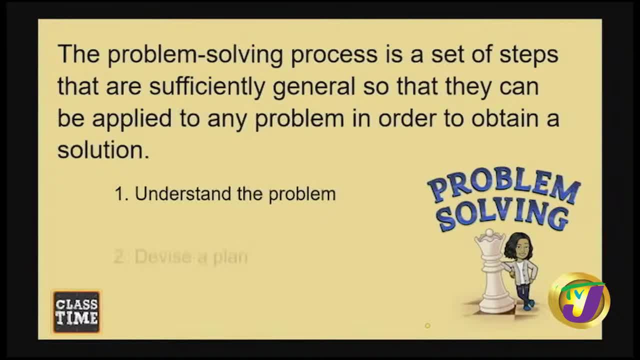 Great. And in understanding the problem, we had to devise a plan. We plan out something, We come up with some way to figure out how to solve that problem. So we made a plan- Great, And then what else we did? You implement the plan. 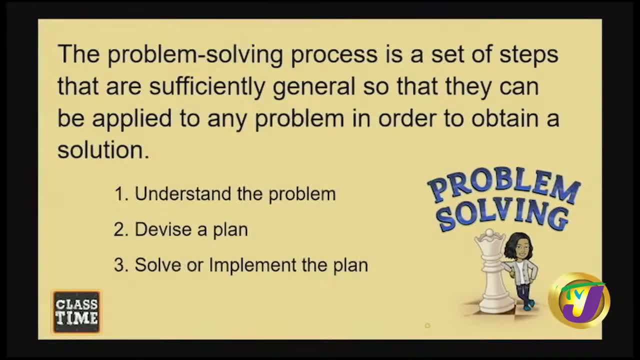 Good, And in implementing the plan, We know we have to solve it, don't it Right? We find a solution Any way you want, term it Right. And then guess what? We can now check to ensure that that plan that we came up with and we implemented that plan, that it does work. 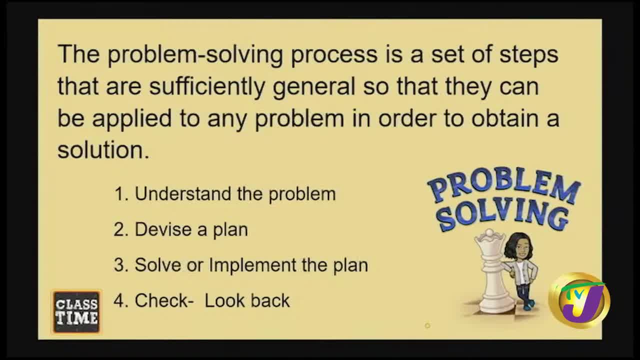 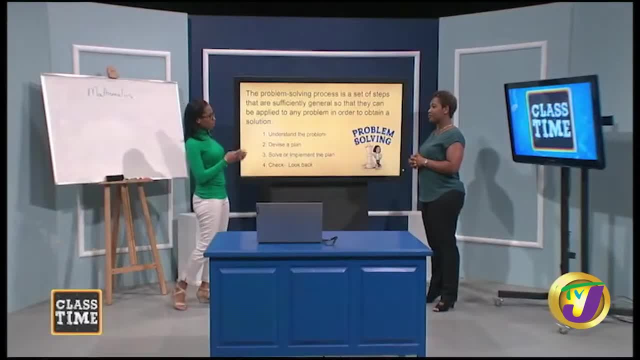 Because guess what happens? Sometimes the plan don't work, you know. So you really have to go back and check and look back where you made that error and make a new plan. All right, So since we would have spoken about Junior with his problem, we're now going to take a look. 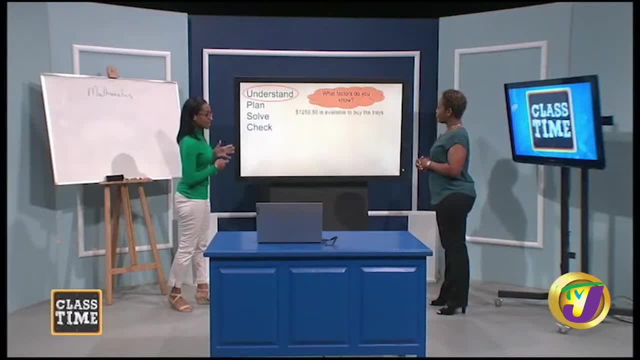 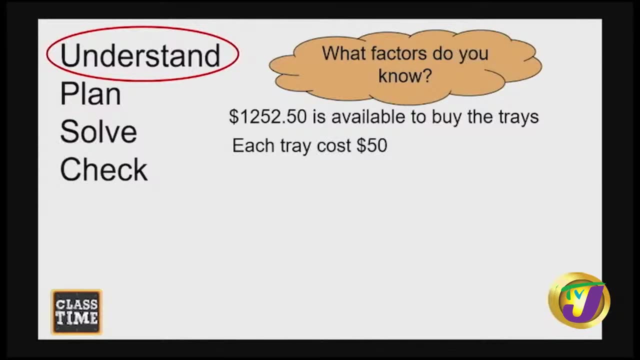 Take a look at everything. So we looked at the factors that he had. Right, We know he had $1,252.50 to buy the trays. What else we knew Each trays cost $50.. Great, What else That this little cost here? he definitely can't take the trays on his back. 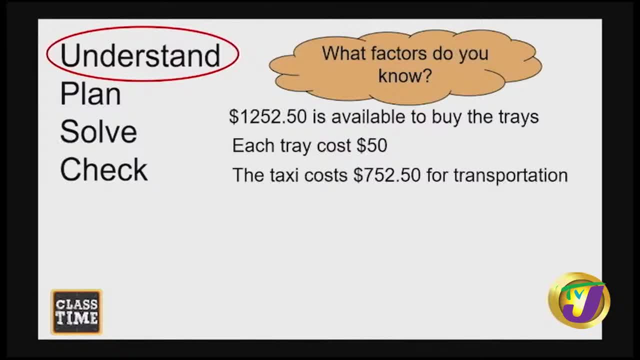 He needs a taxi which costs $752.50.. Great, So we have all of these factors that we know. So we know these factors from the problems. So what you're saying, in knowing these, we now understand Junior's problem. 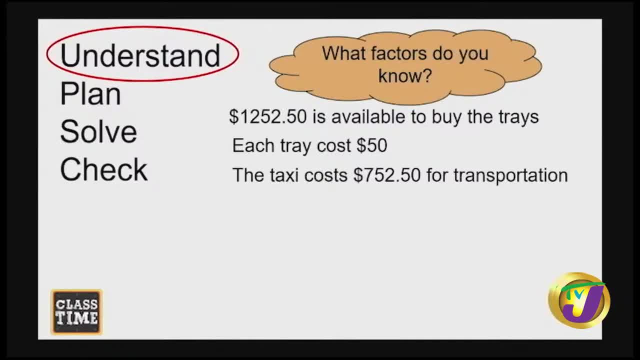 We need before saying that we definitely understand. so we know what he has, But guess what we need now to finalize that we understand the problem. Yeah, We need now to figure out what he needs, which we said already. Right, He needs to figure out how many trays. 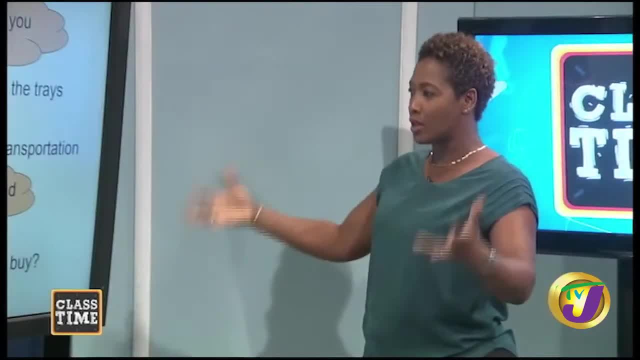 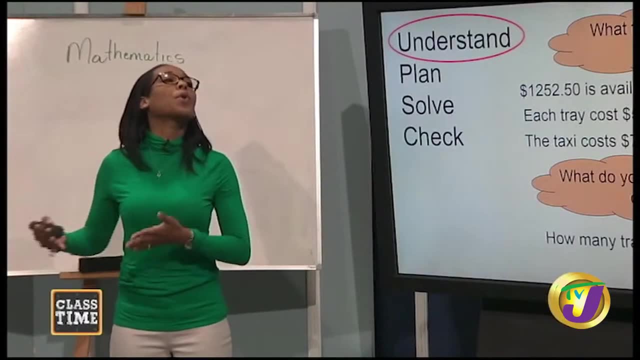 Right, Right. So we need to know what we are working towards. what is the problem that we have, Nice? So to understand the problem, we need to look at the factors that we have and we also need to know what we need to find out. 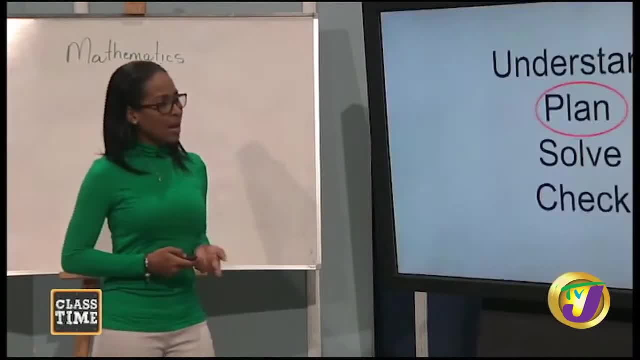 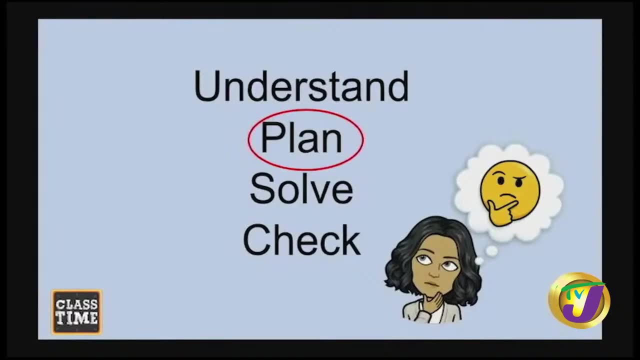 Right, What is required? Yes, That's in the understanding process, All right, And we would have spoken about our plan. After you understand, you can definitely plan. You know what I'm thinking though, about with the plan- The plan that I'm thinking, because if we know how much money he has, 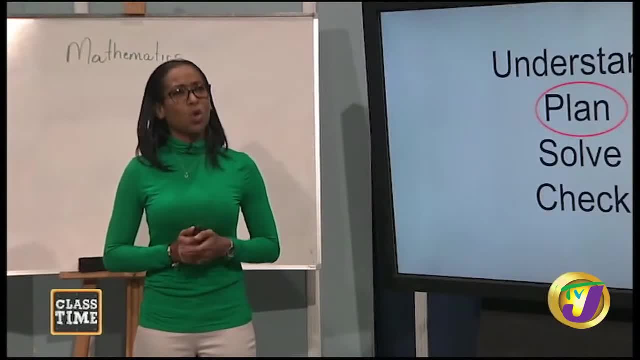 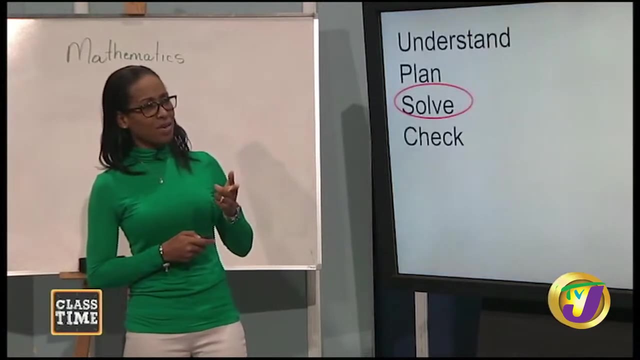 Right, We know that he needs some trays. We know that each tray costs $50.. We also know he needs transportation and there is money allotted for transportation Mm-hmm In this plan. I think maybe in solving it we can maybe work it backward. 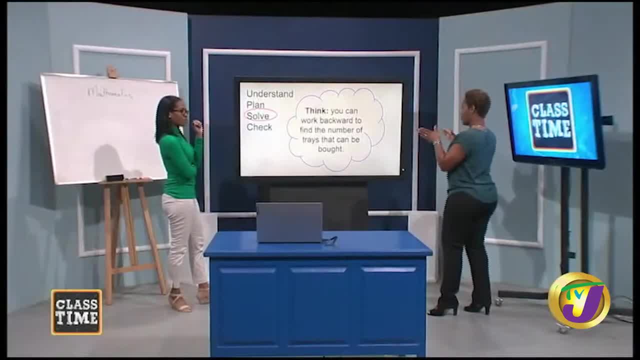 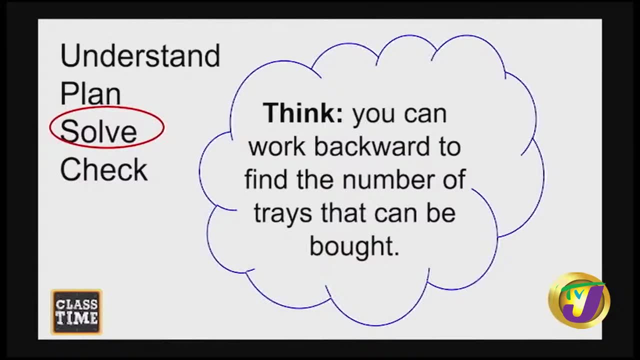 All right, All right, So you're going to solve this by working backward. You can work backward to find the number of trays that can be bought. Yeah, man, That's what I'm going to do. I'm going to work it backwards. 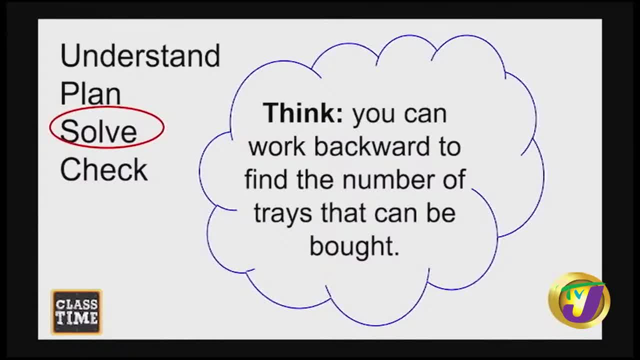 I'm going to use what we have. All right, We could discuss and see how that works then. no, Yeah, I'm going to show you. Okay, Don't stress it, man, I'm going to show you. So look here now. 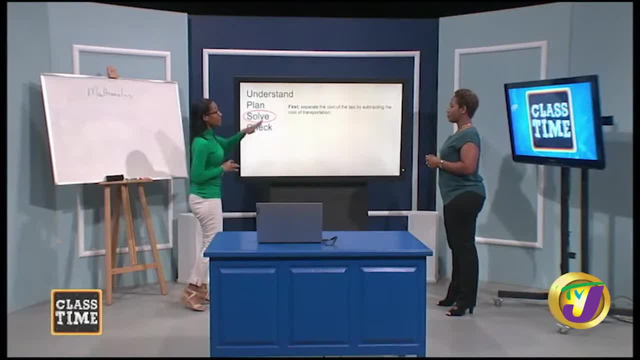 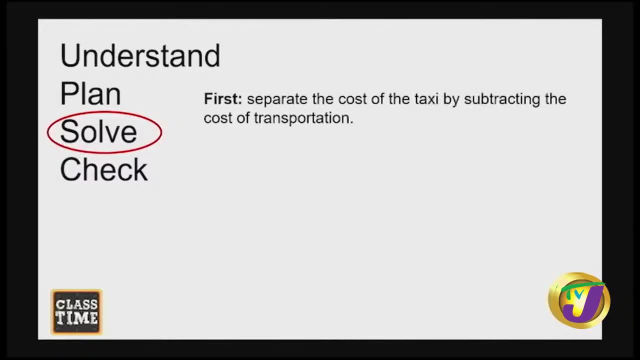 So the first thing that we're going to do, we're going to separate the cost of the taxi by subtracting the cost of transportation. Makes sense From the money that he has. So he can't order taxi till another time. Not at all. 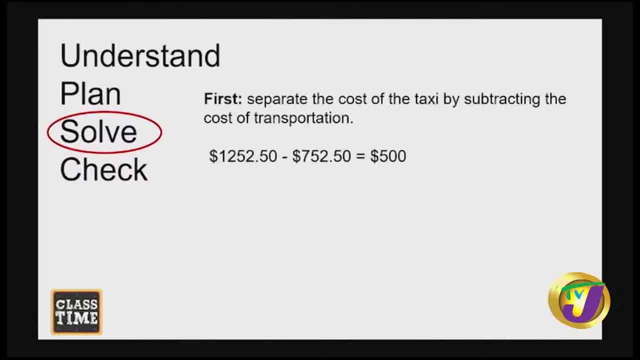 So right here, we would have done this. So we know that he originally had $1,252.50.. Right, right, We also know that the taxi is $750.. So we would have subtracted to know how much money we're working with now. 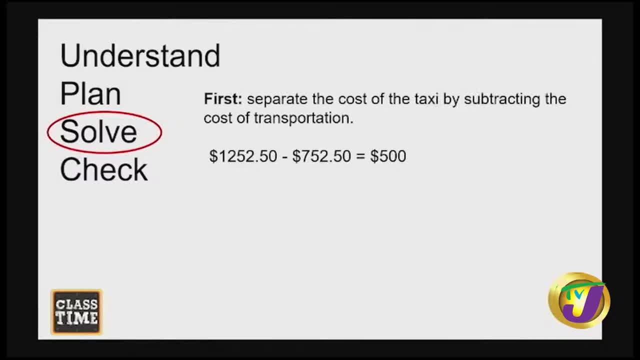 So we have $500 in all. $500 in all, And there I thought Juna could buy a whole heap of trays. No, That's why we need to understand the problem and that's why we need to figure out how we're. 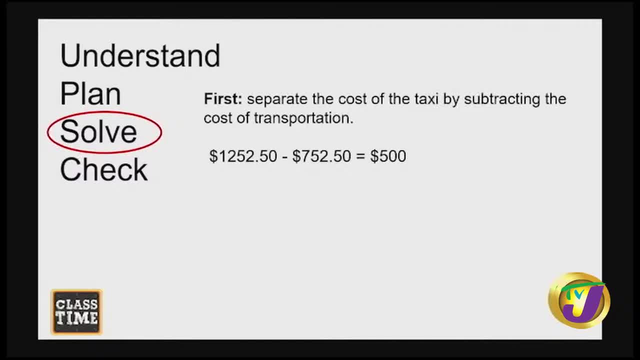 going to solve the problem, and then we implement this plan that we have. So we know we have $500 working with now, So now we need to calculate how many trays can be purchased From the money left Now. how would you calculate the cost of this? 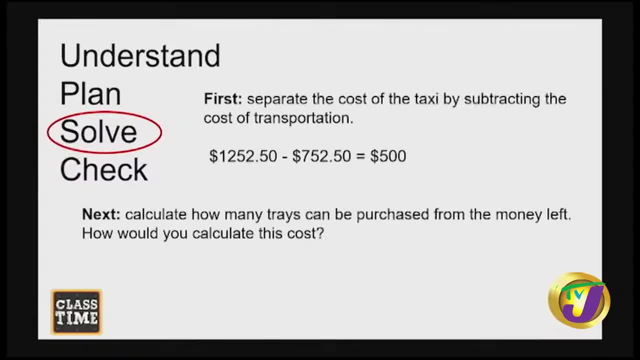 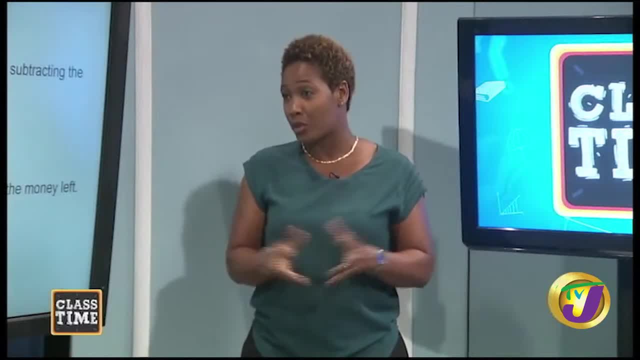 Tell me now: Well, definitely, If you have $500 and you know each tray costs $50.. It's simple, man: You divide $50 to $500. Or you can go on and add $50 to each $500. Whichever way you want to do it. 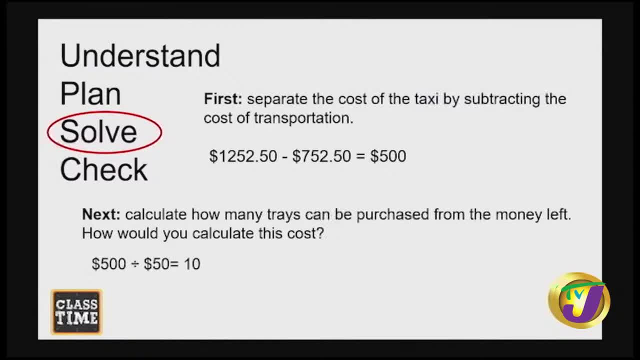 But efficiently, I would divide $50 to $500.. Great, Because we were told that each tray cost $50.. Right, So in dividing my $500 by the $50, we know that how many trays we have, So we know that how many trays Junior needs now. 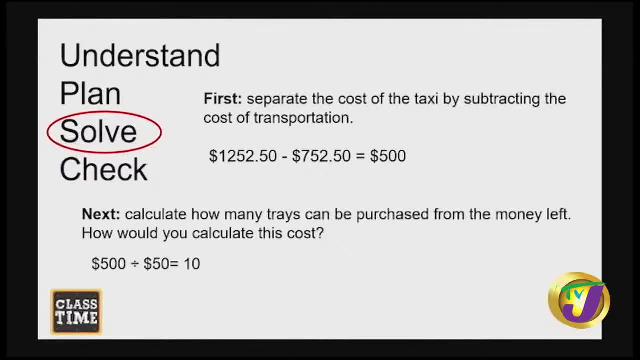 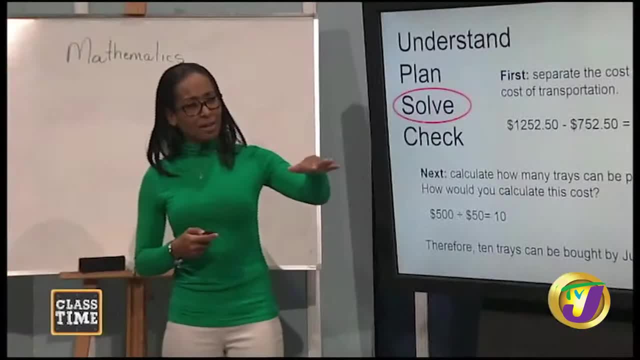 He can only purchase 10 trays. Great, Good job. 10 trays. I'm sorry Kind of small, but all right. 10 trays. So what we realize, you realize. I told you what's my plan, how we're going to figure. 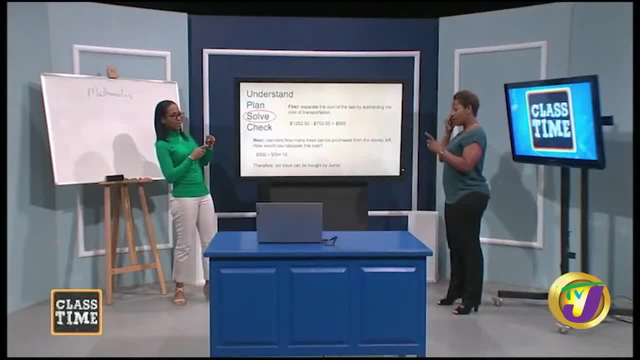 out how many trays he needed. You remember what I said I was using. You said you're using the backward method, The backward way. Yes, I want to work it backwards, Backwards, You want to work it backwards. You want to try and figure out what we need to find out. 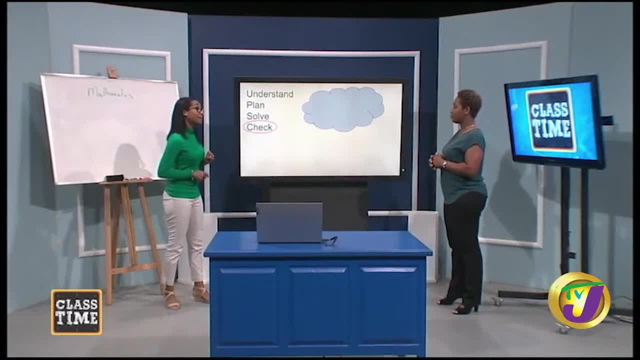 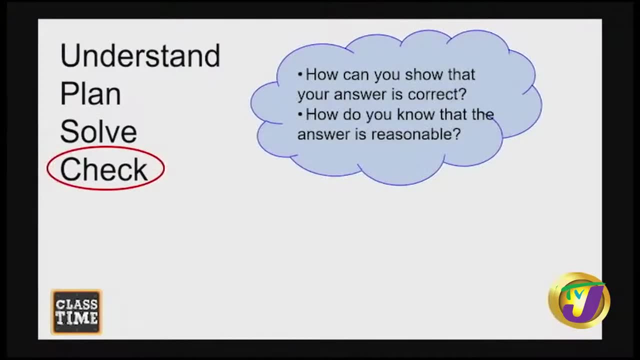 Right, All right, And now I'm going to check. All right. So I want to show you that our solution that we would have arrived at is correct. So here we have. how can you show that your answer is correct? We're going to check it. 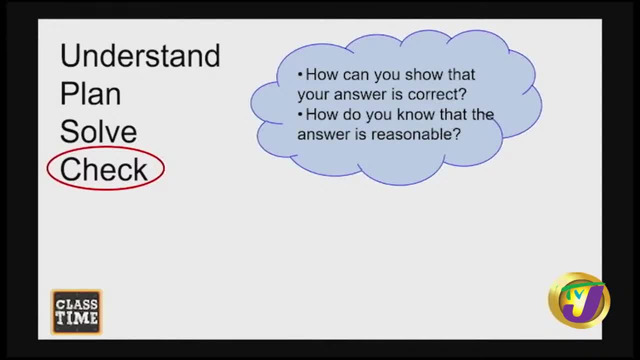 That's right, ma'am, And when checking it, we're going to know if our answer is reasonable as well. So let's take a look here. Okay, So we would have arrived at 10 trays, And we also know each tray $50.. 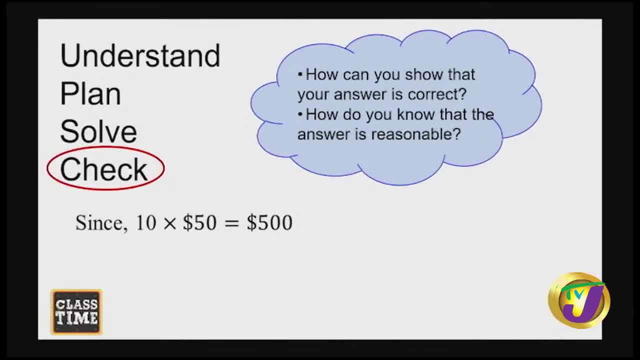 So when you multiply the 10 trays that we got by the $50 for each tray, what did we get? $500. $500.. And then let's look here now. So we know: $500 for all the trays. Now the 10 trays that he needs. 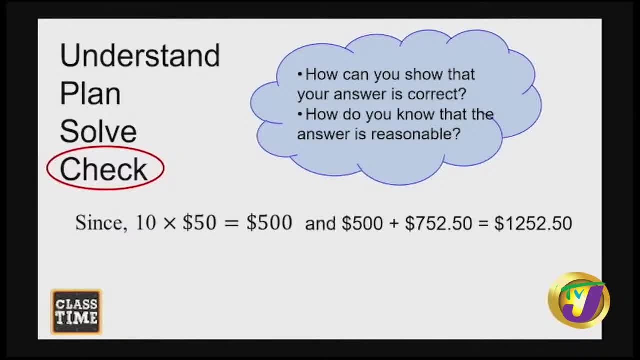 And the transportation cost would have been $752.50.. So when you add those two figures, you'd have gotten exactly what Juna started out with $1,252.50.. So you're right, Your answers are correct. Simple, simple something. 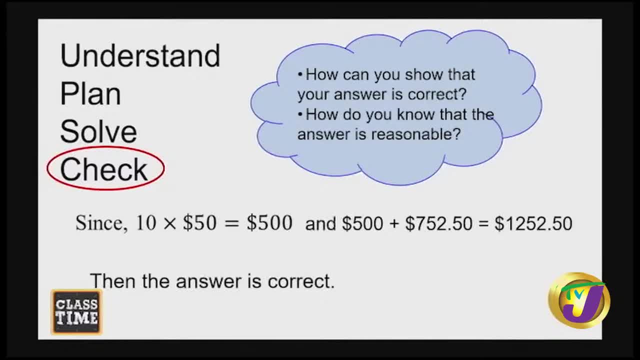 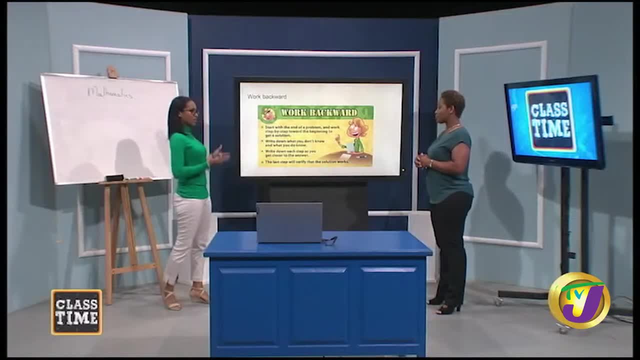 So we solved the problem. We solved Juna's problem. So now Juna can go to the farm store and buy him 10 trays- Simple, simple, something Just like that, Exactly. So in looking at this now and remember I would have shared that I was working it backward, 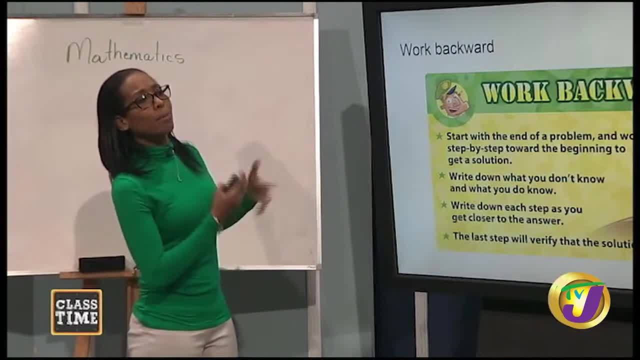 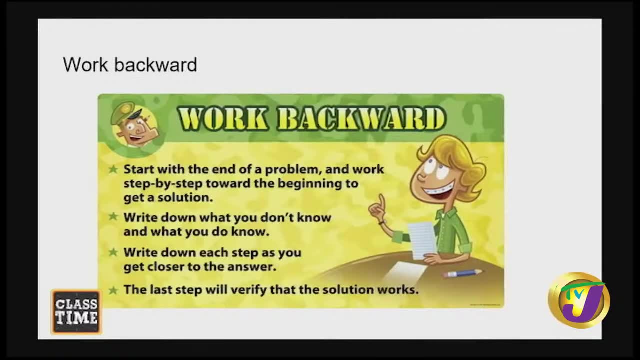 right. So now this is what is entailed in the working backward. Okay, So one start with the end, Start with the end of a problem And work step by step, which is what we did toward the beginning to get a solution. 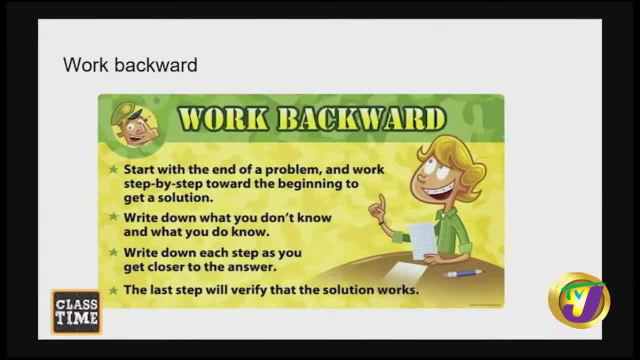 Right Two: write down what you don't know and what you do know Makes sense. Right Three: write down each step as you get closer to the answer. Okay, And four: the last step, which we did, will verify that the solution works. 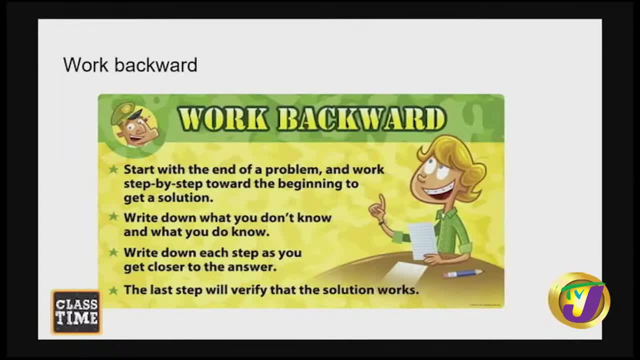 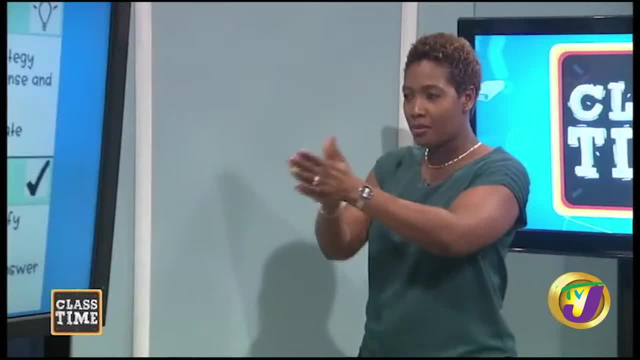 And we saw that it works. Everything added up And we're good to go. Yeah, We were okay, All right. So here we are. So what you said- planning, I mean problem solving. So when you are faced with a problem, we must first understand the problem. 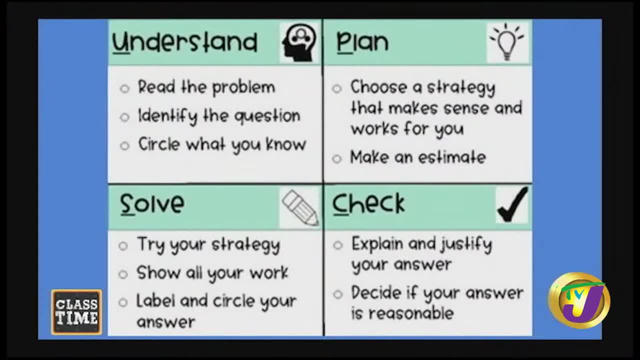 When we understand the problem. we may read the problem and maybe one twice identify the question or questions circle what you know. That's understanding the problem. Then next we plan, Choose a strategy that makes sense and works. Make sense and works for you. 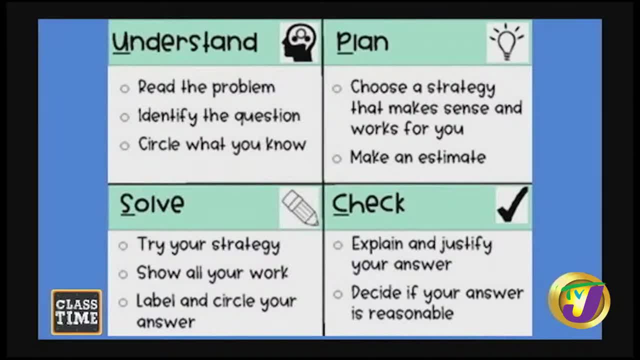 Now that first strategy. it worked for us this time, but it may not always work, So it's always okay to make another plan. Then make an estimate. what you think the answer may look like Might be yes, Right. 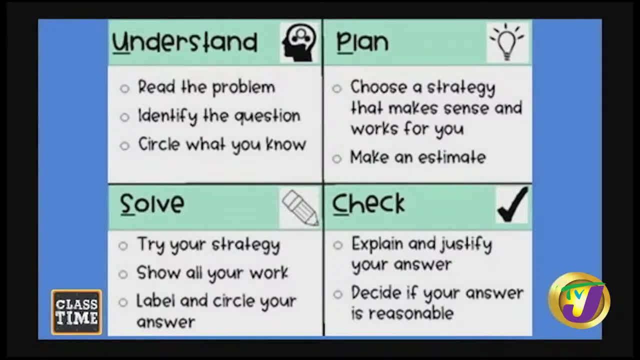 Solve, try your strategy, show all your work, label and circle your answer. And then, of course, the last thing is to check, Explain and justify your answer, Decide if your answer is reasonable, And we pretty much did all of that. 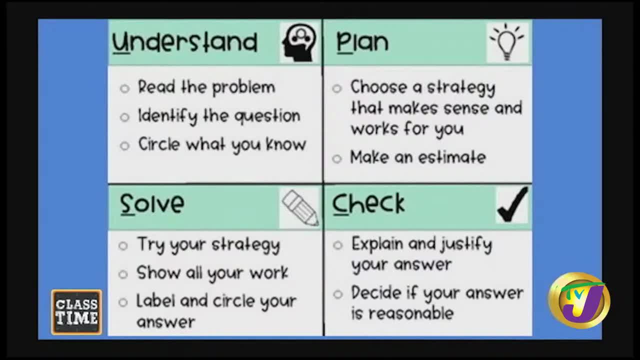 Come on, We did all that And when we're thinking about all this that we have here- understand, plan, solve, check- we are again looking at the problem-solving process. There you go. There's a process that we go through and we know we definitely have to understand the. 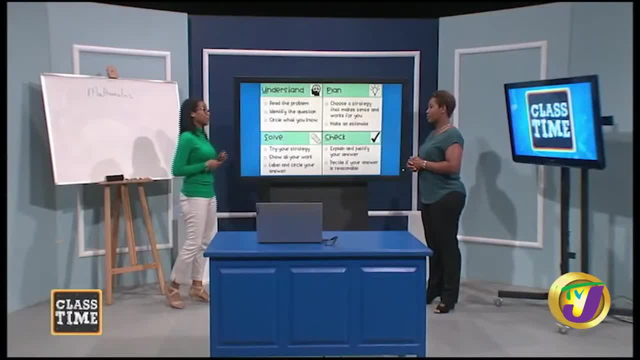 problem. So I want to know if you are paying attention. So guess what is going to happen now? I know you know You're going to just give me something else to do. Yeah, man, because I want to know how you're going to solve this problem. 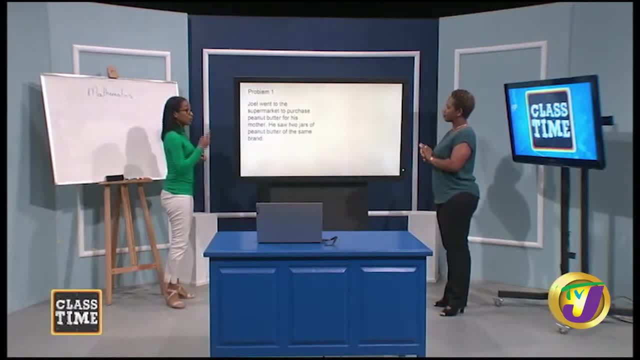 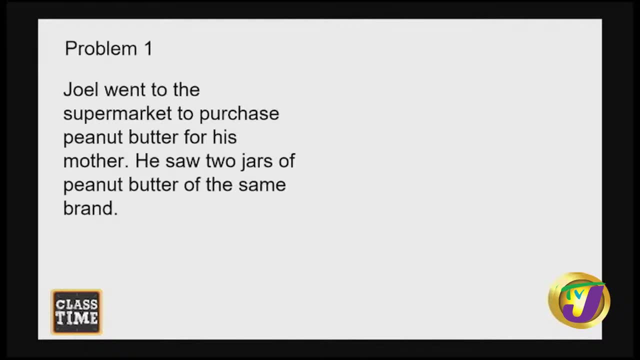 All right. So here's your problem. So Junior went to the supermarket, Oh, yes. So Joel went to the supermarket to purchase peanut butter for his mother. Okay, He saw two jars of peanut butter of the same brand. That's right. 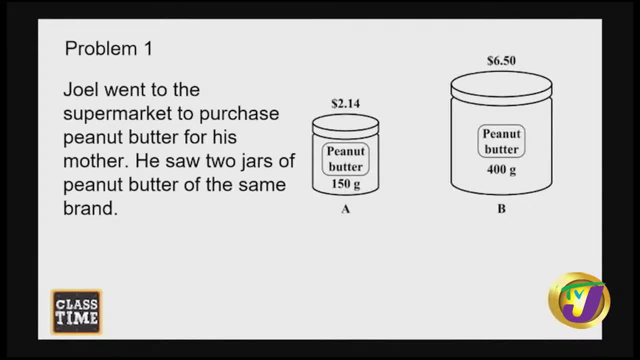 And there's your photo of the peanut butters, right? The brand is peanut butter, Right? This is what I want you to tell me now. He wants to know which of the jars Shawn is the better buy. Ah, All right. 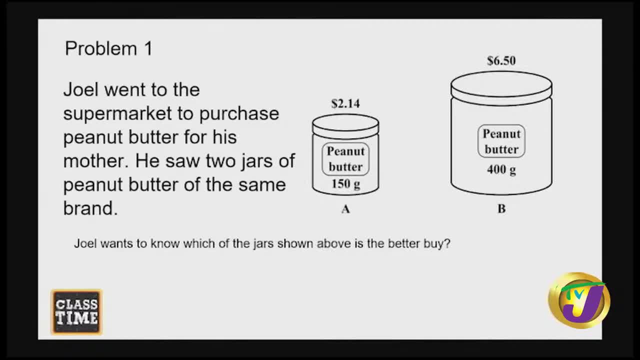 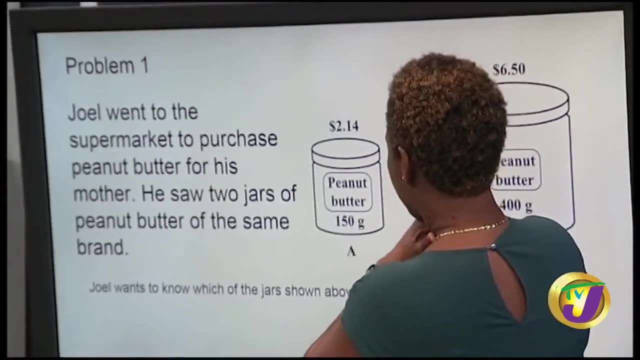 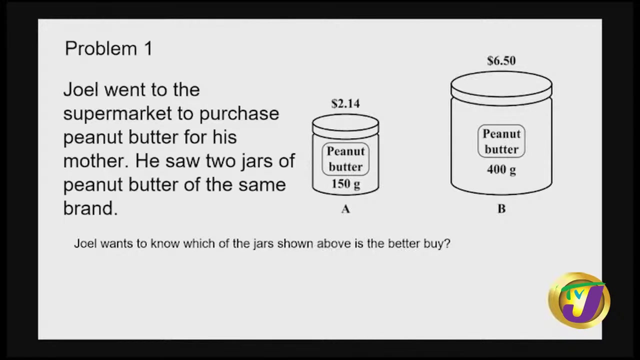 So we have a small jar there which is 150 grams of peanut butter for $2.14.. And we have a 400-gram jar for $6.50.. All right, What is the better buy? All right, He's going to have to figure out how much he's paying for a gram. 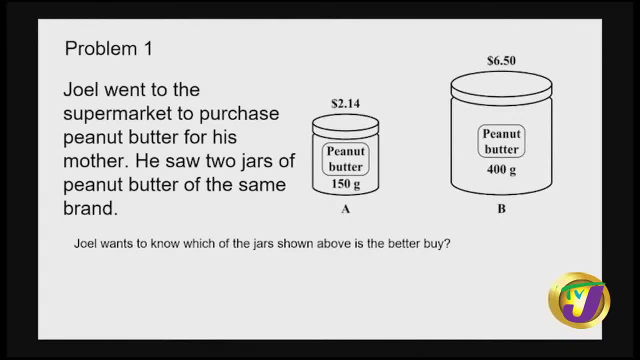 Or he can figure out. Can he ask himself how many of the small one can fit in the big one? Well, he can ask himself that question for real. But when he's going to the supermarket he can't go put each of the small ones, the 150. 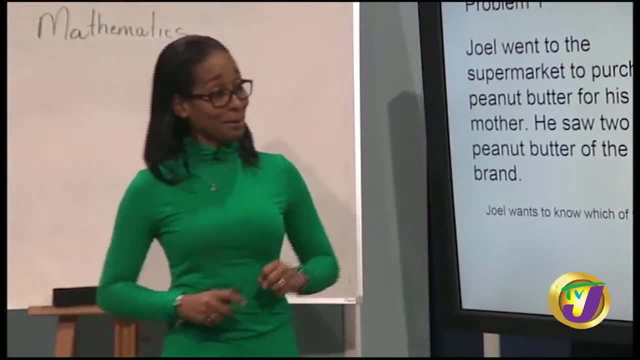 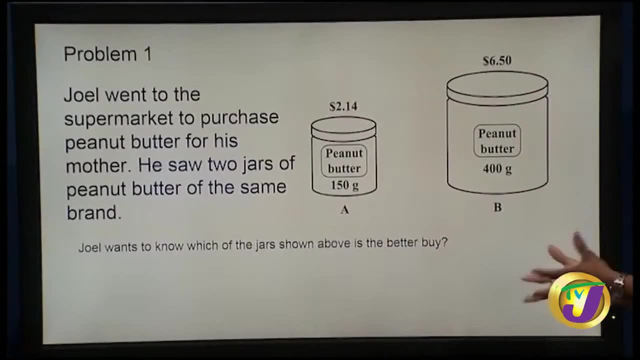 grams into the 400-gram jar. He's not going to do that, He's going to estimate, All right. So now you're talking. So he needs to understand what the cost and the cost in relation to the amount of peanut. 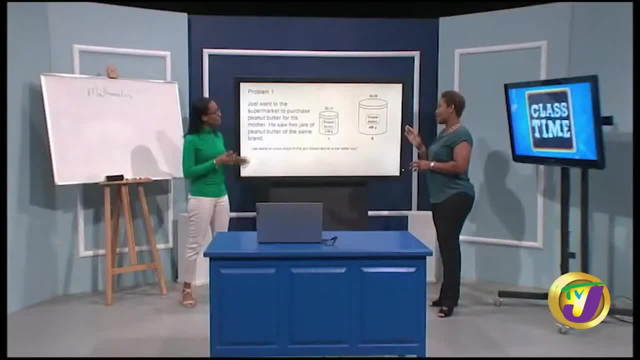 butter. All right. Now you're thinking: man, you're getting somewhere. good, Yeah, How much You know: 150 to two. You can't do the Croatia thing. You know 150 to $2.14 and 400 to $6.50.. 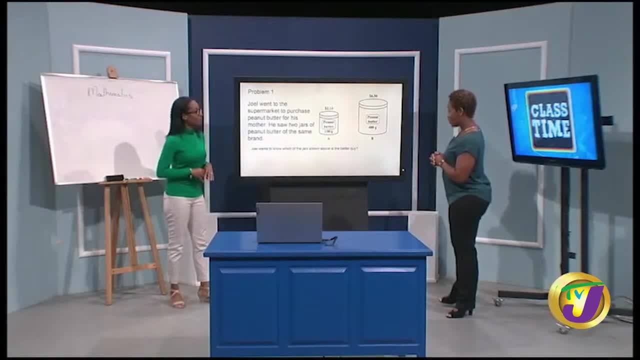 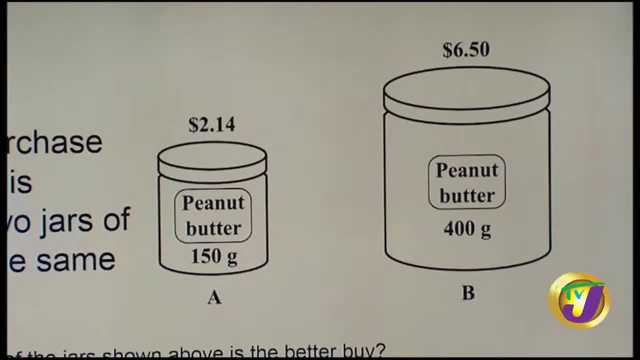 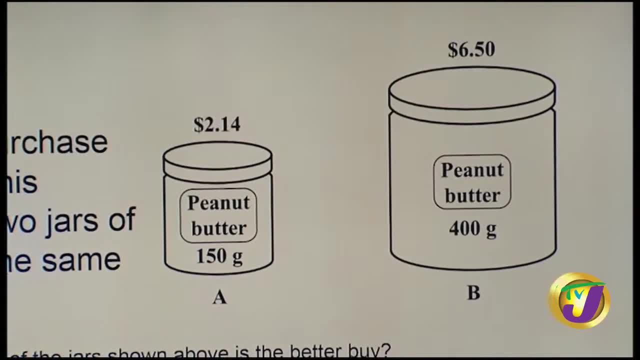 But one bigger. so we don't sell, You don't just buy the bigger one. You don't just buy the bigger one. Yeah, Mm-hmm, Well, that is what you just would do, But you wouldn't want to figure out which one is the better buyer. 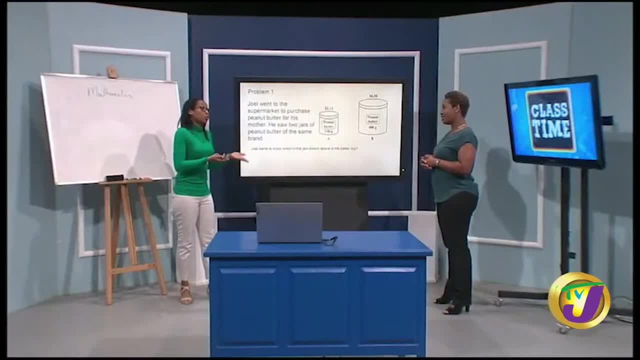 Which makes sense. Yes, It does make sense. So what you would have shared earlier about him trying to figure out how much for each gram Right in each of the peanut butter jars, we can try and take it from that angle. 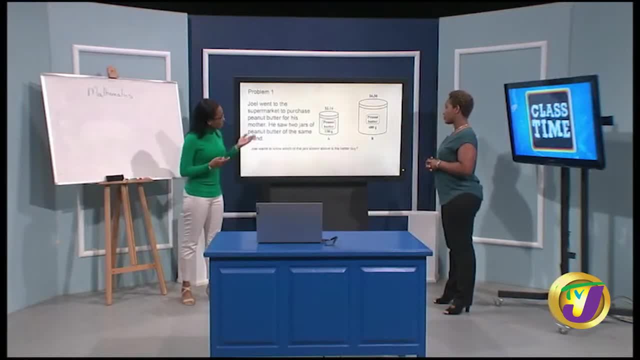 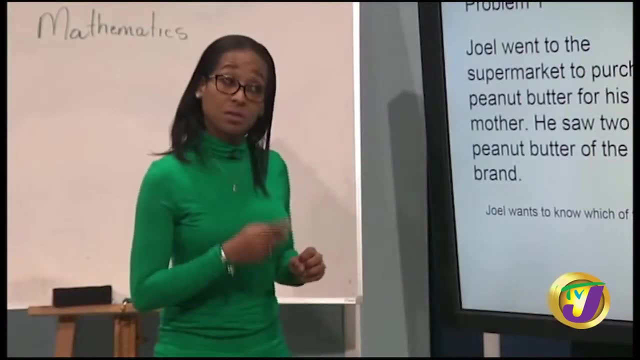 All right, Because it's the same brand. It's the same brand, It's the same brand, But it's just that. hey, one costs $2.14.. One costs $6.50.. But how much for each gram in each of the peanut butter jars? we can try and take it. 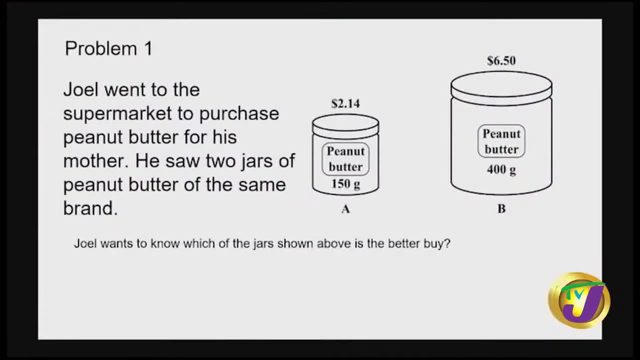 from that angle, All right, So we would look at how much is it for each gram in jar A, how much it is for each gram in jar B. So let's take a look here, because I had written it down. So let's look here. 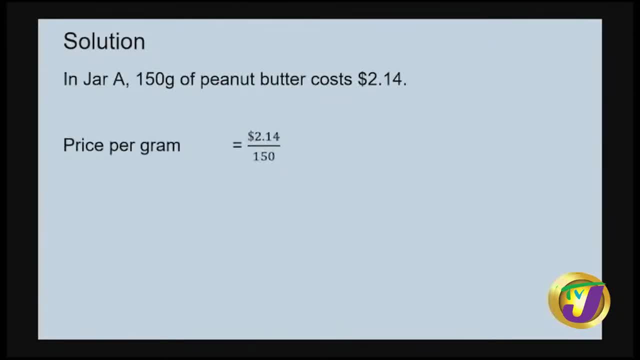 Right. So in jar A 150 gram- we know- of peanut butter cost $2.14.. Acceleration, Yeah. So here we have it. So we are now trying to figure out what's the price for one gram In the small jar. 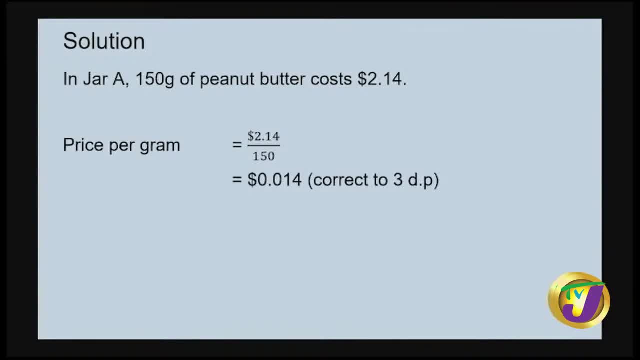 All right, Hear me about one gram. It's for one gram, One gram. So here we have it. So the cost now is $0.014,. correct to three decimal places. That's the price for one of the gram in the 150 gram jar. 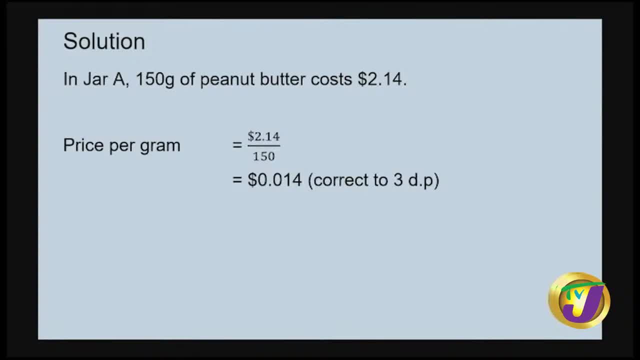 Cheap man. Wait a minute, Let's look again. Yeah, my friend, Let's talk about the jar B now. Okay, Which was the 400 gram Right, Which is a bigger jar Right, Right, Great, So we're doing the same process now. 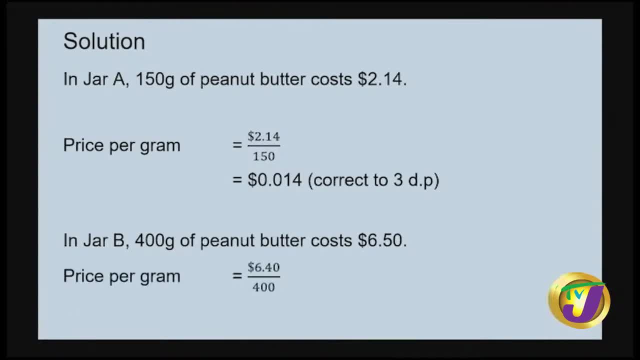 We need to figure out what's the price, How much per gram. Per gram of this one, Okay, Which is $0.016.. Look at that, I thought I'd be getting a deal Correct to three decimal places. So guess what. 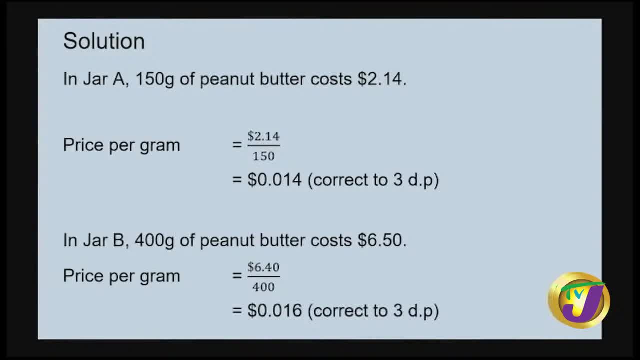 You're going to have to look closely now. Yes, To tell me now, because you would have shared all of this with us. So look closely now to tell us Which one would you work with, Jar A or jar B? Well, jar A. 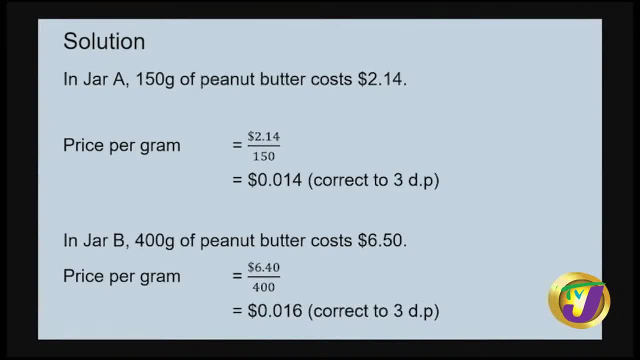 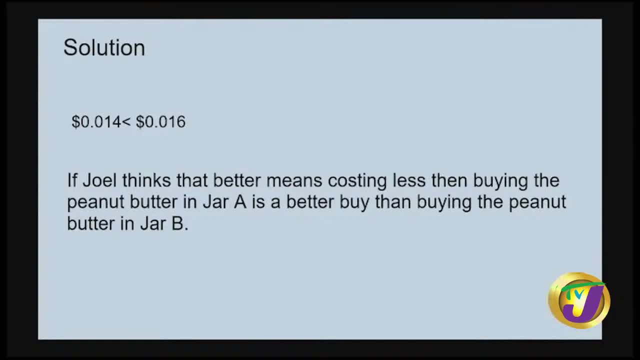 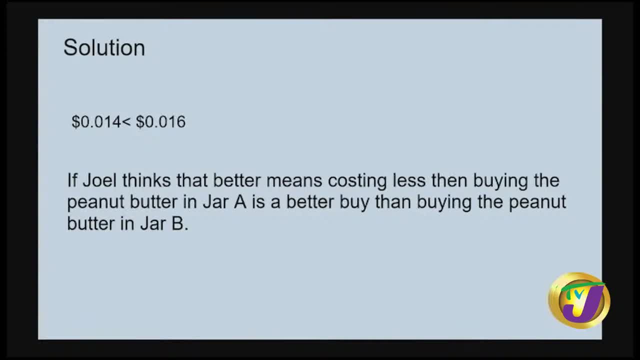 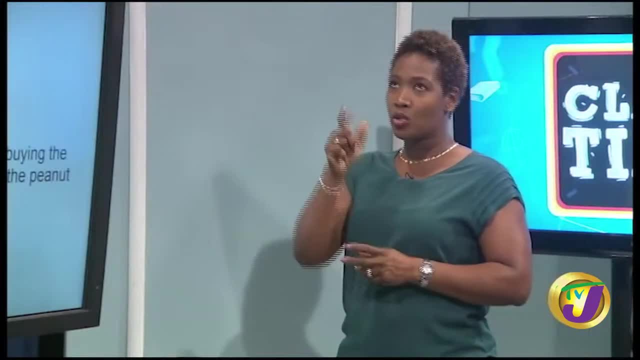 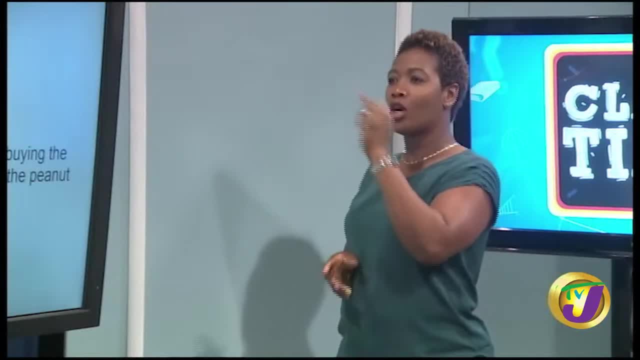 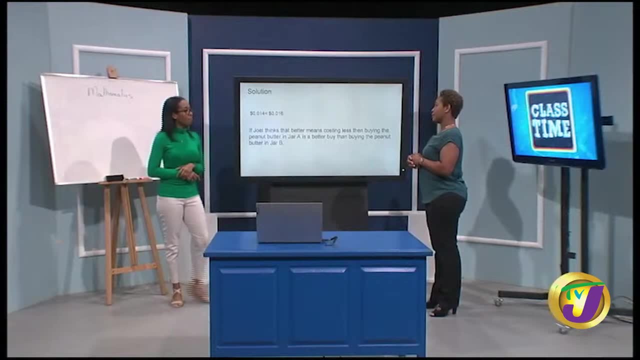 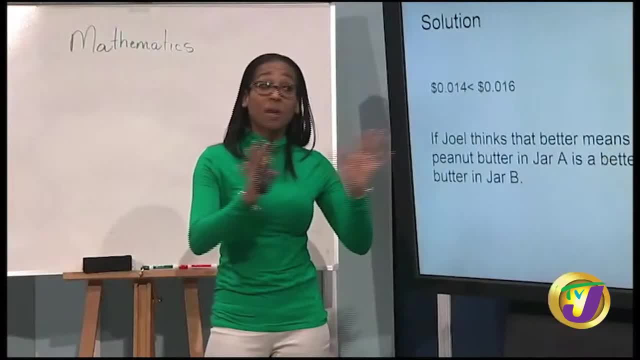 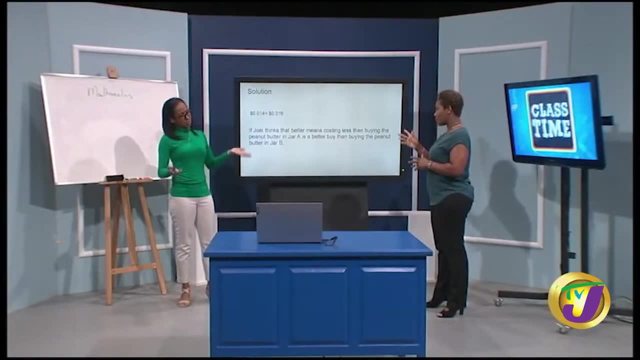 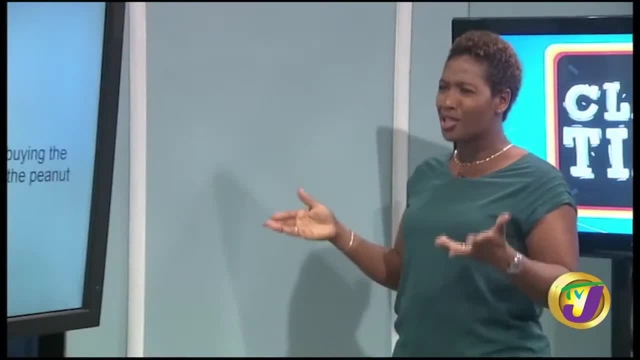 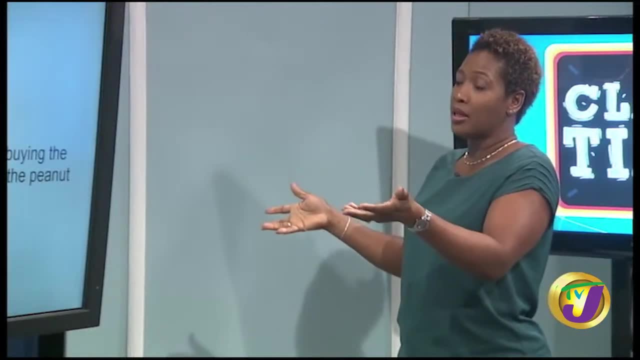 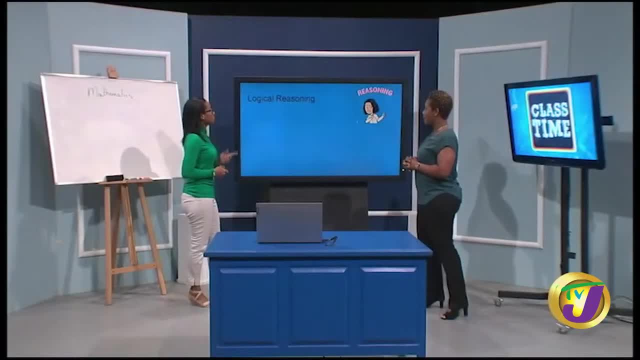 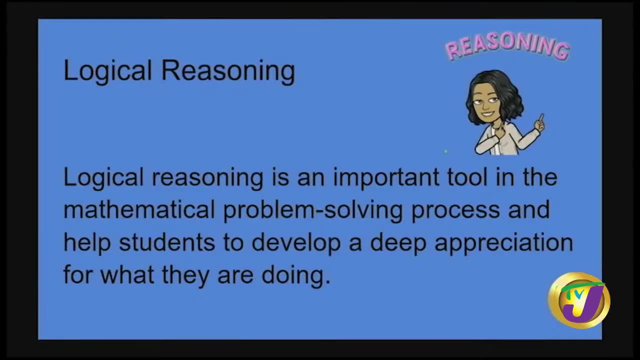 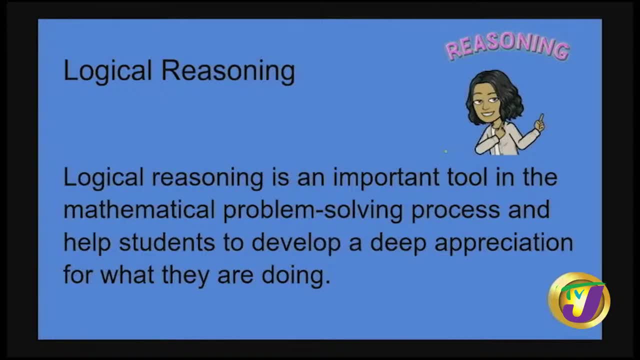 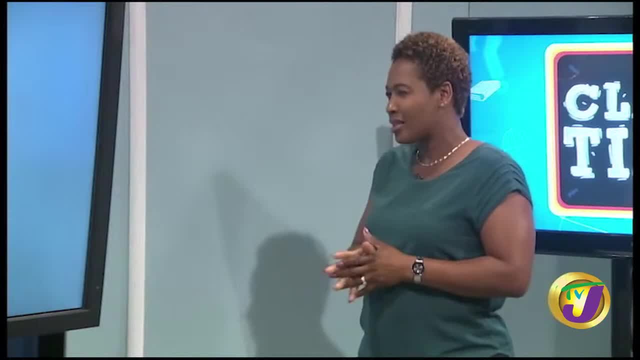 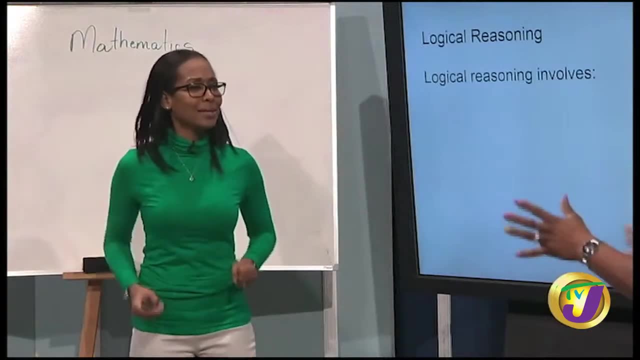 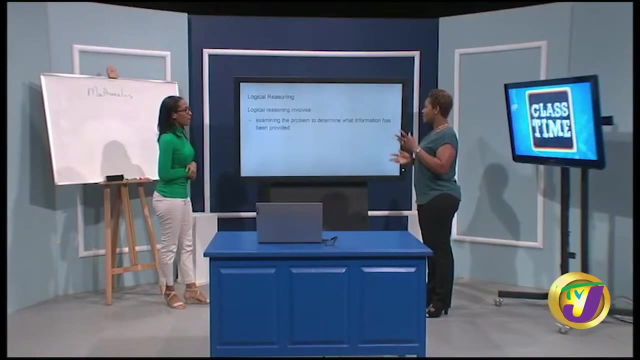 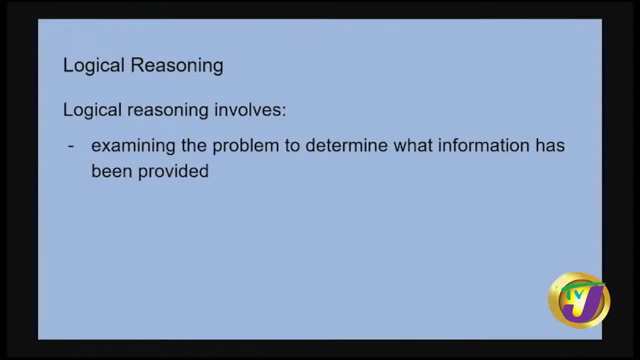 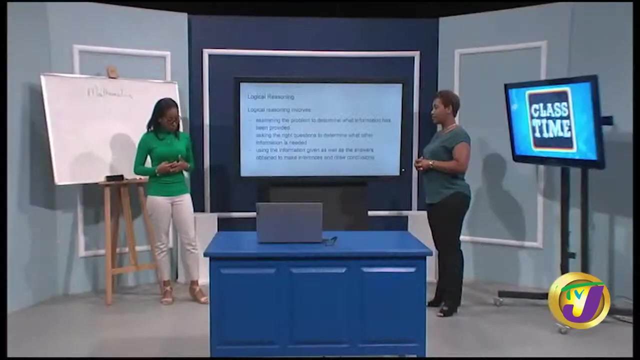 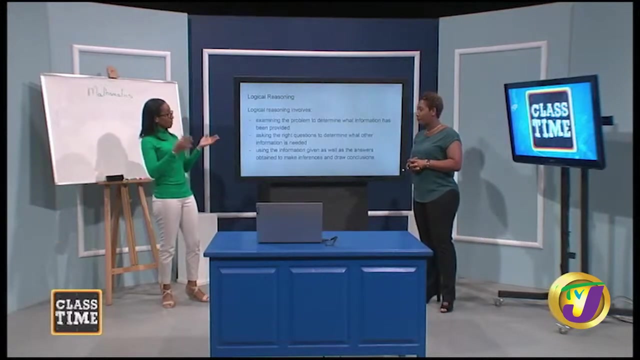 provided, asking, asking the right questions to determine what other information is needed and, last, using the information given, as well as the answers obtained, to make inferences and draw conclusions. so we would have, yes, logical reasoning. so we would have looked at working backwards in one of our problems, in june's problem, right during that farm. yes, and now joel have his. 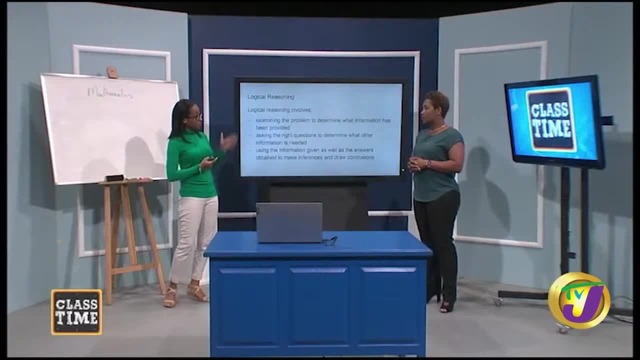 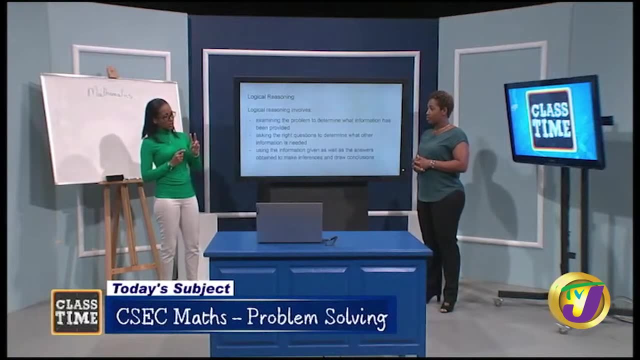 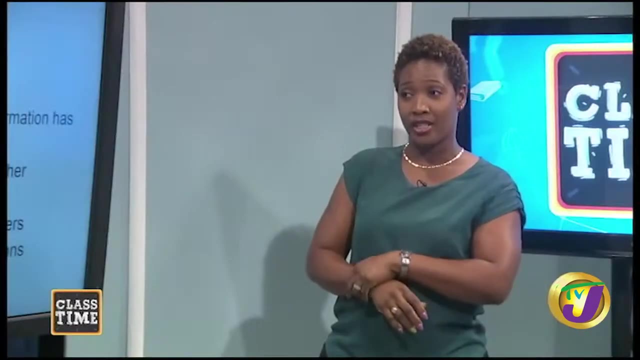 supermarket problems and we reasoned for june, for joel's supermarket problem. hmm, so we're going two strategies. i hope we're taking notes. you know we've gone two strategies, but we did say another, problem solving doesn't mean that you have that one plan. i see that you can try different. 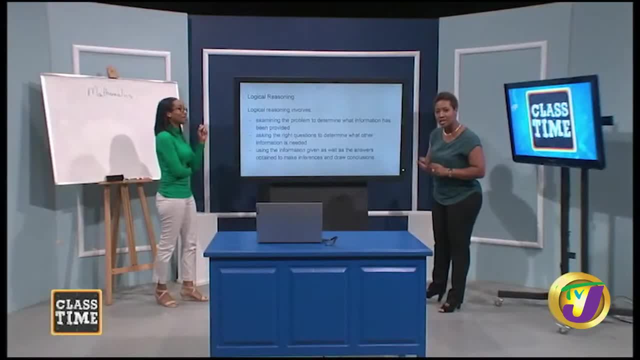 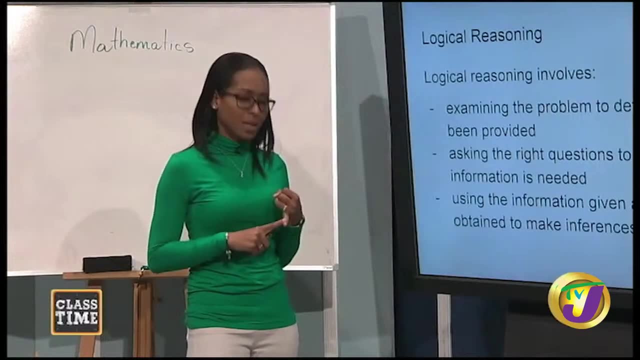 ideas, different strategies- right, use the correct term. different strategies can be applied and we're still linking it to our process. so we have to understand the problem. i have definitely have a plan. you have a plan, great, solve it, and then we check. that's right. so that's our problem solving. 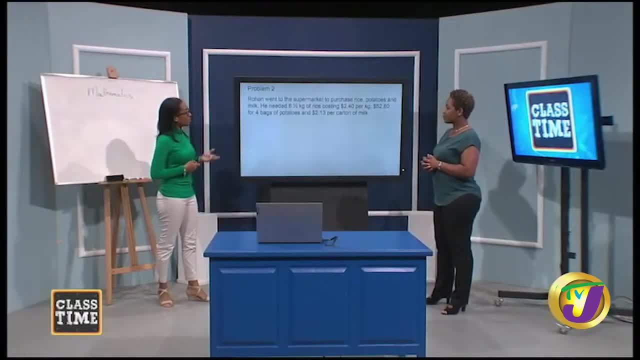 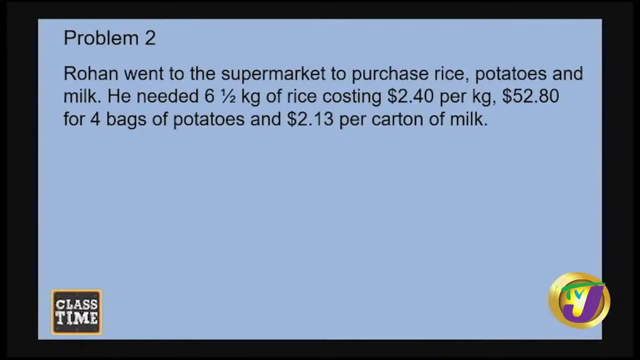 process. so here we have another problem. all right, so apart from joel going to the supermarket here, rowan is going to the supermarket too, and he wants to purchase rice, potatoes and milk. he needed six and a half kilograms of rice, costing two dollars 40 cents. 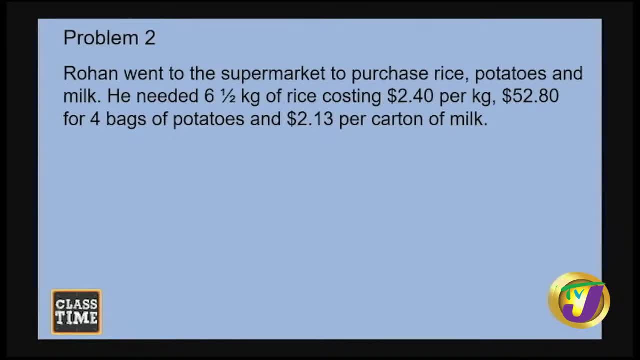 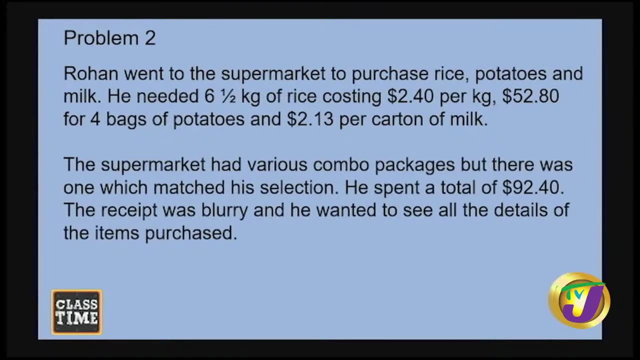 per kilogram right, 52 dollars and 80 cents for four bags of potatoes, and two dollars 13 cents per cart dollars per carton of milk. the supermarket had various combo packages and we cannot test it at the moment. many times have them packages going on. 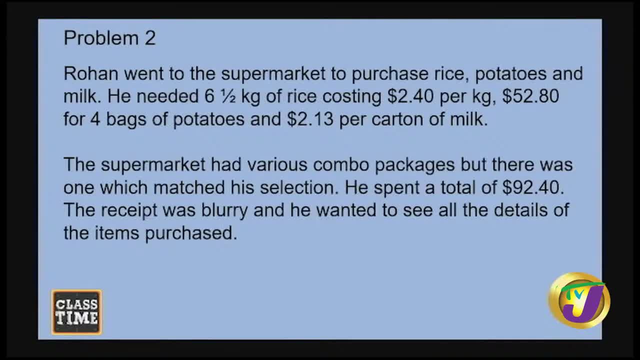 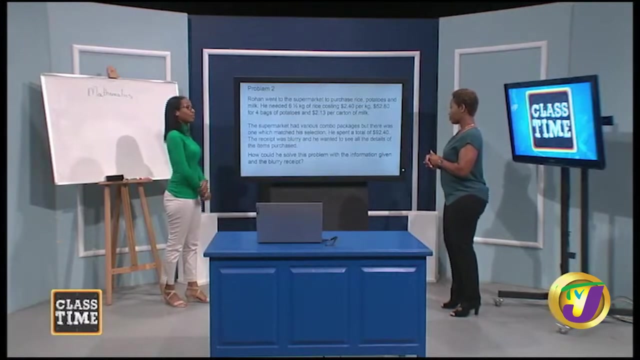 the deals, but there was one which matched his selection. he spent a total of 92 dollars and 40 cents. the receipt was blurry and he wanted to see all the details of the items he purchased. how could we help solve this problem? now, with the information given and the blurry receipt, all right? 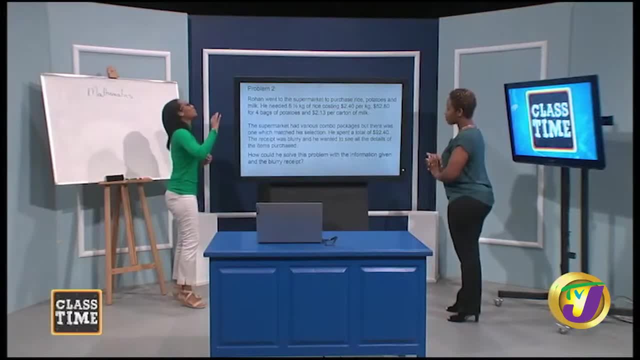 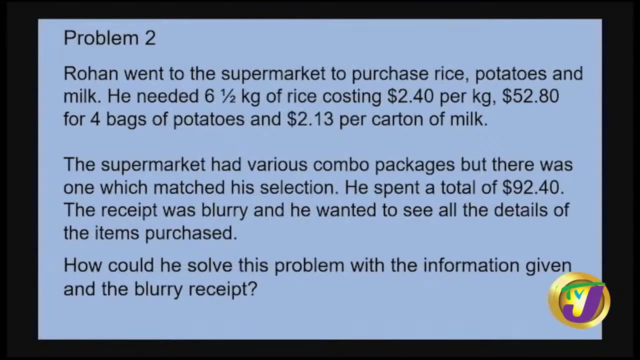 so let me read it again, because i need to understand this problem. good job, so really right there, and then you can realize, so that you don't necessarily have to read the problem one time and get it sometimes two, three, four times. you have to read it, right? so go ahead. so let me read. ruan went to supermarket. he purchased rice, potatoes and milk. 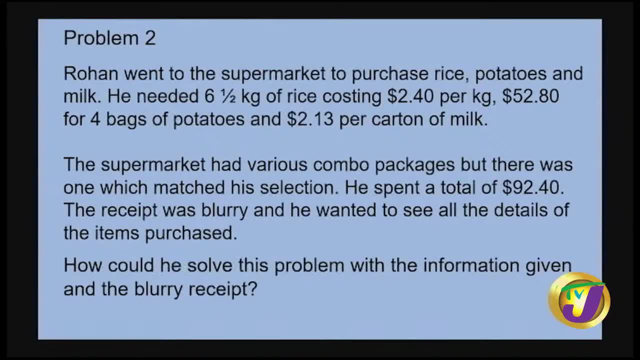 he needed six and a half kilograms of rice costing 2.40 cents per kilogram, 52, 70 cents for four bags of potatoes and two dollars thirteen cents per carton of milk. all right, so right away. i know he bought three things, three different items, yeah, and I know the cost of them. 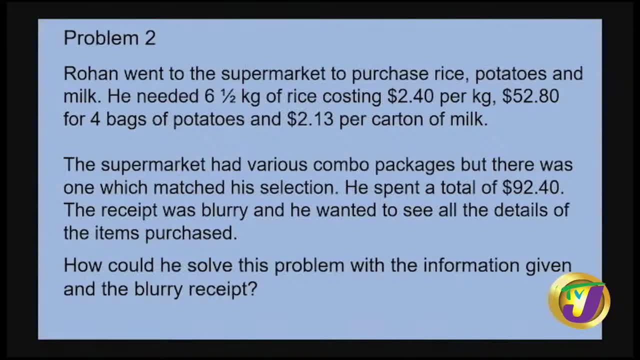 ish. yes, all right, so his combo know this combo thing. so he's he know his total was $92, 40 cents. that's his total. yes, so all right, all right, I get information, all right. what is being asked again: how could? Oh, remember the receipt was? 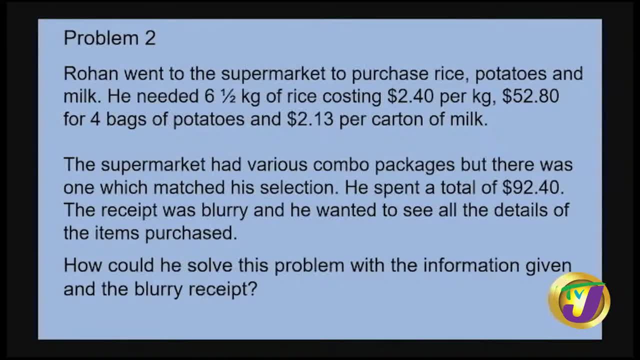 blurry and he wanted to see all the details of the purchase. I'm assuming that he realized the receipt by when he reached home. Camilla socks and back from printout. thank you very much done. that's why we need to pay attention to you. got he's at home now and the receipt blurry, okay, how? 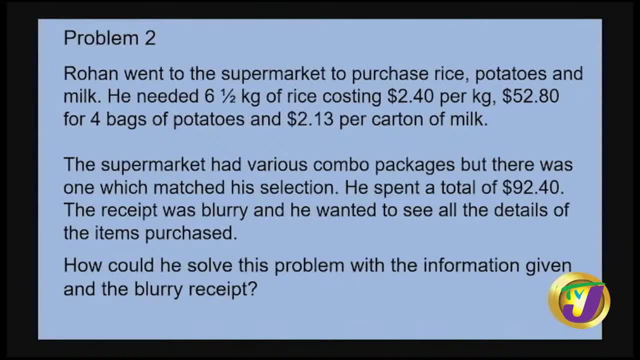 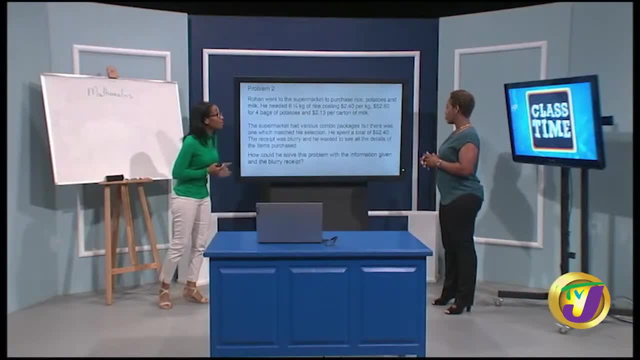 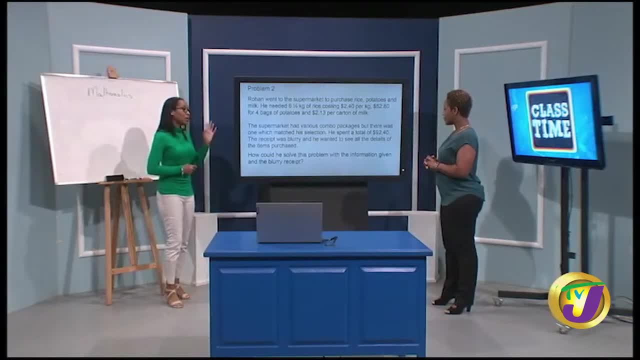 have a problem and he needs to fix the problem. so, based on what you would have just done, yes, so we understand the information given and what is required of us- we need to help Ruan figure out how he spent the money and you would have highlighted, you see, just like what we told him early and understanding. 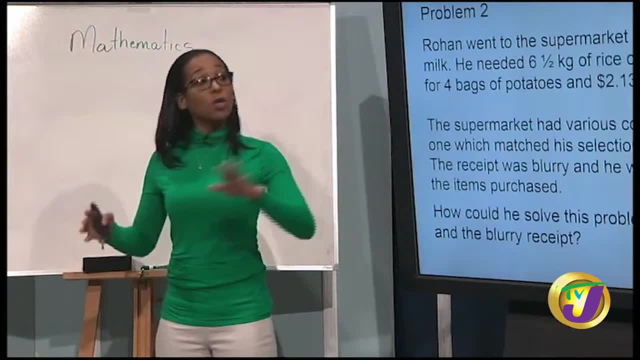 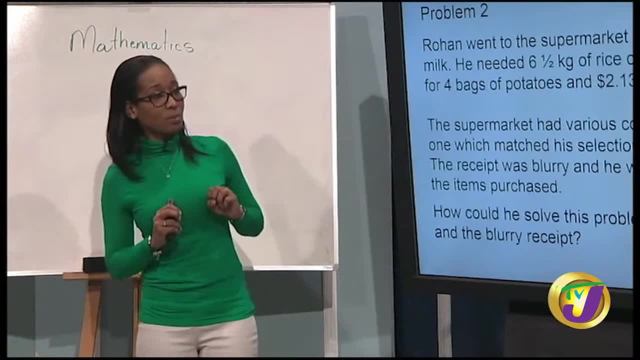 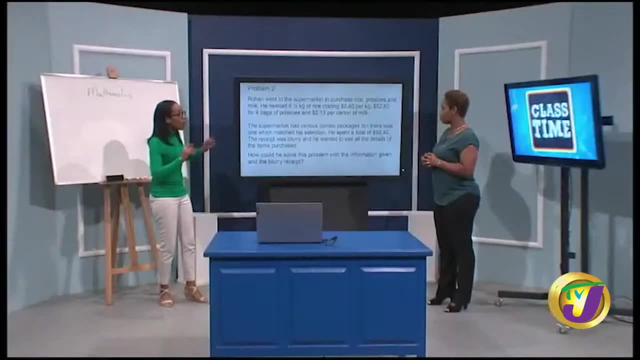 I need to fix this problem. I need to fix this problem. I need to fix this problem. so I know that he's needed six and a half. so I know that he's needed six and a half kilograms, underlined the milk, you know. and then you would have also said to us: hey, circle it to the total and we look. 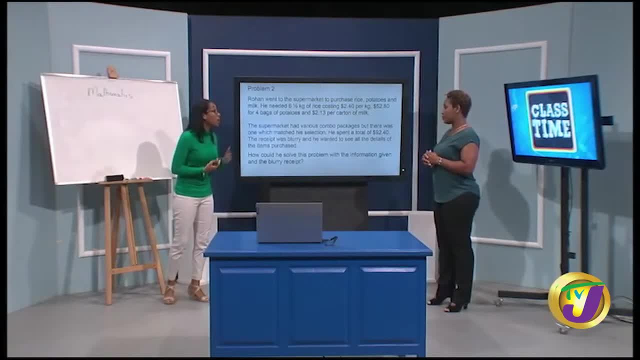 what the problem is, though. we need to know what we're trying to figure out right. we know what we have and we need to know what we are trying to. a call help him to replicate the receipt. yes, we're trying to help him to have a The receipt, then to be able to look at it to know exactly how much money he spent on, maybe, each item. 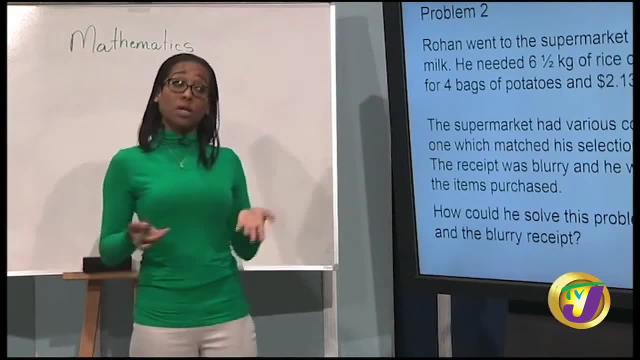 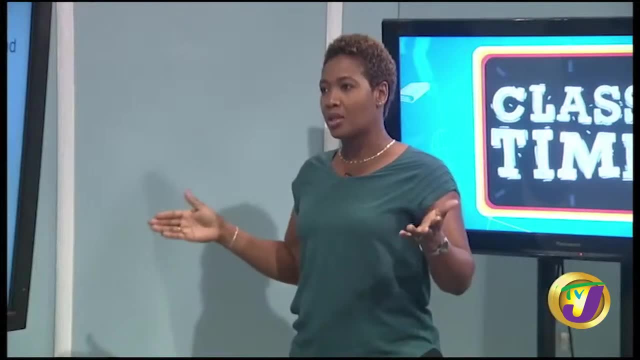 based on what we're going to be looking at too, on each item, the total cost for the item, differently from the unit price as well. Right, so we want him to pretty much be able to see what's on the receipt. 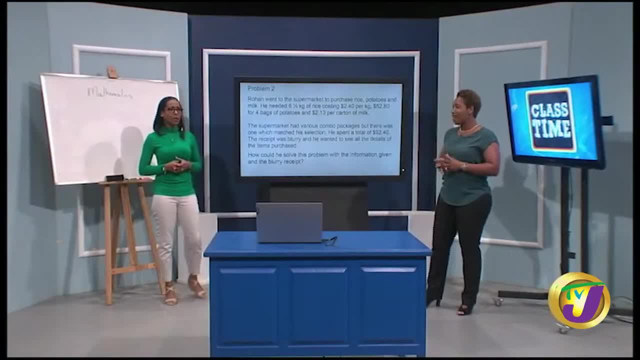 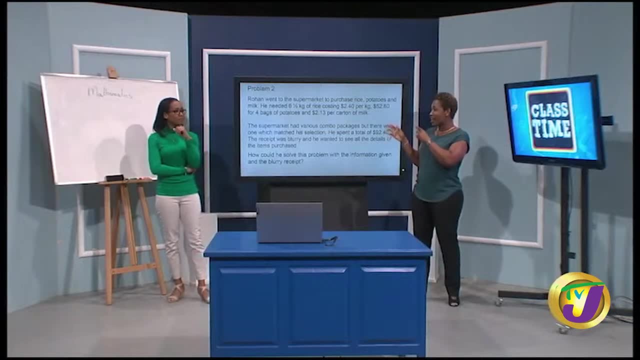 So how are we going to do that? Yes, how are we going to do that? I would love for our audience to work on this right, because this is important. I want them to get a chance to think about this before we even solve it here. 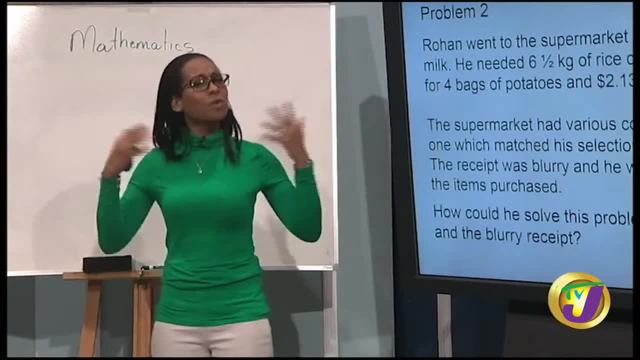 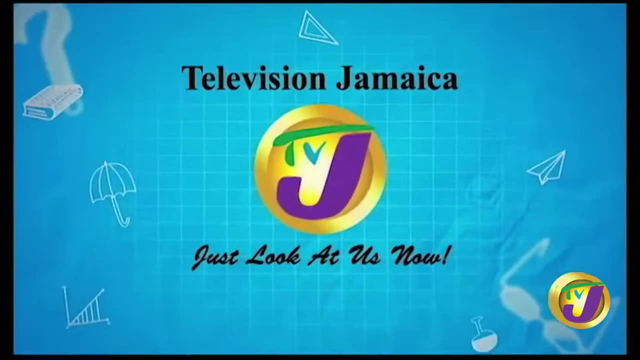 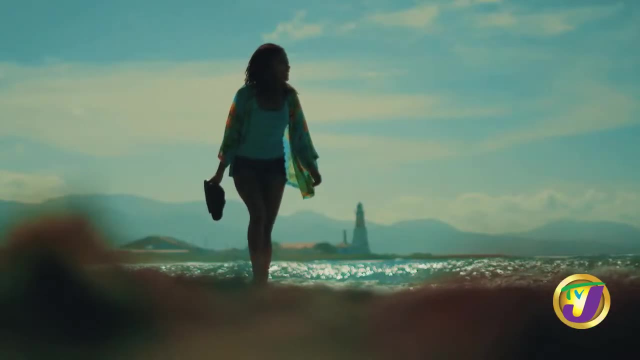 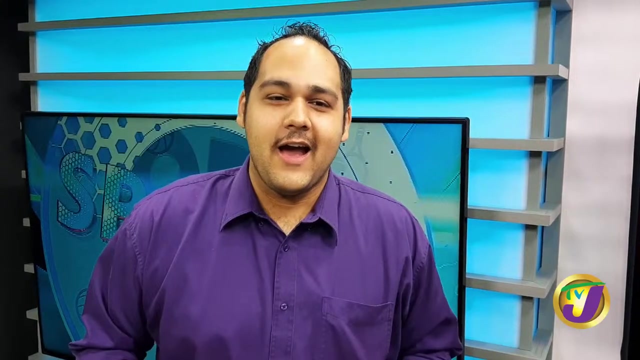 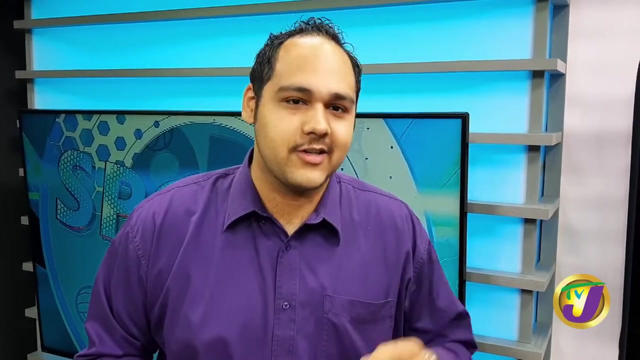 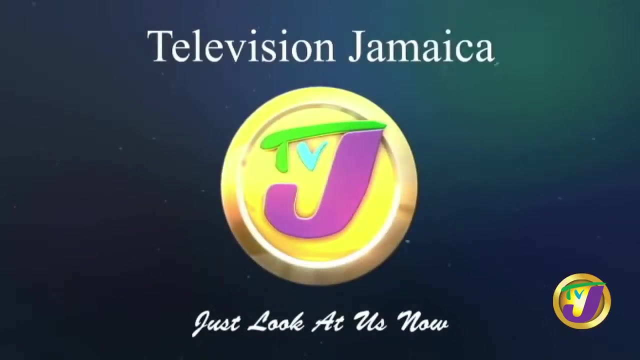 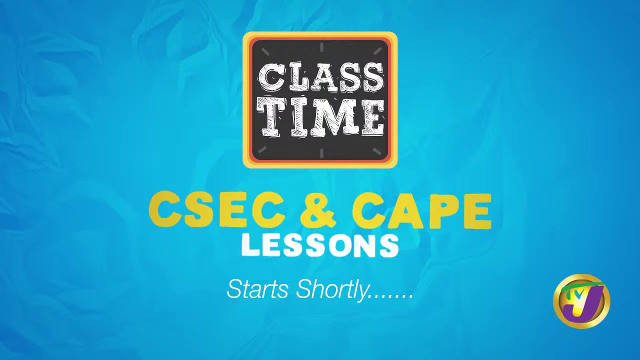 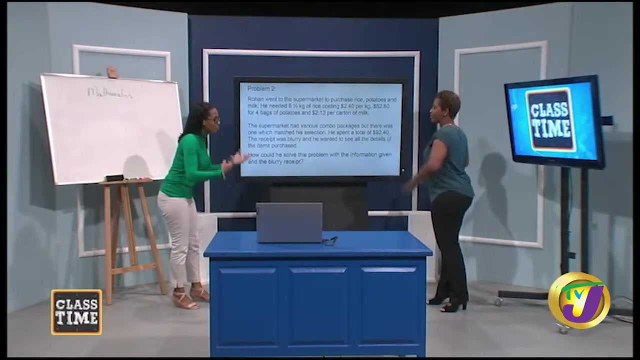 Right, so we'll pause here to give way to a few messages. We'll be back in just a bit. We have it: Live Days. We have it: Live Days. Right, man, and we went through it. We read the problem a second time. 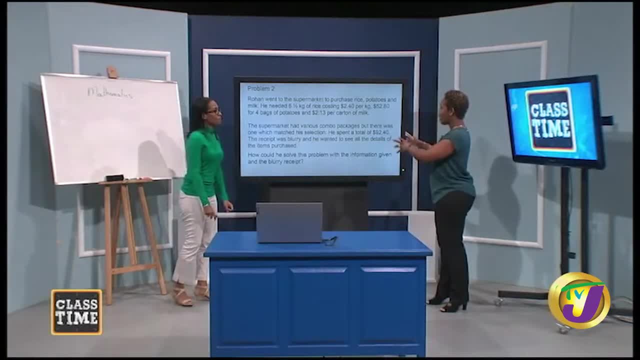 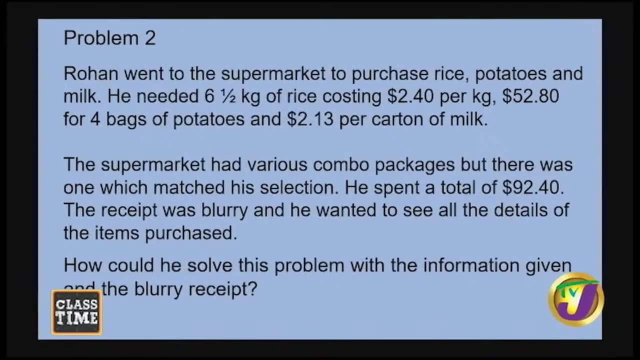 We understood all that he bought and what he paid per kilogram for each thing that he bought. Well, except for the milk, it's per carton, Yes, and the potatoes his bags Right. so we looked at the information that was given in the problem and how much the total that he had spent. 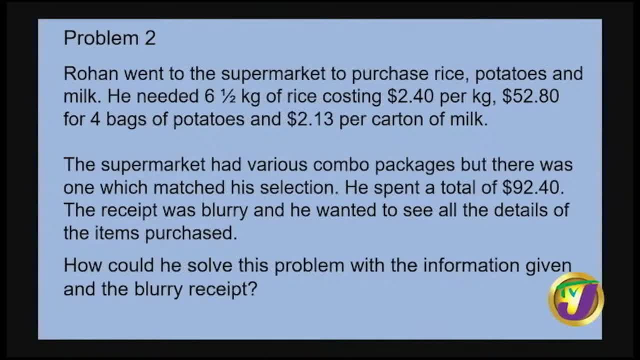 All right. so we are now faced with helping him to pretty much put back that receipt together. So I think maybe we could put this information on the table man. We can put it in a table. yes, Yes, ma'am. 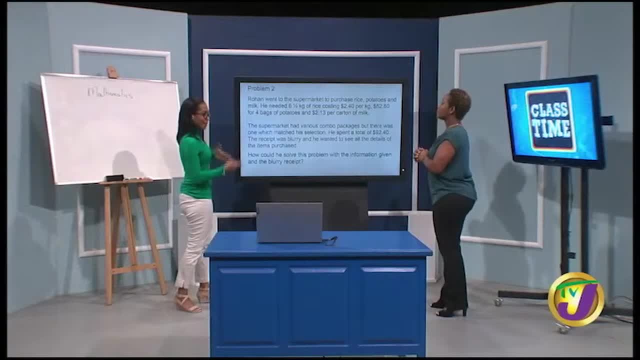 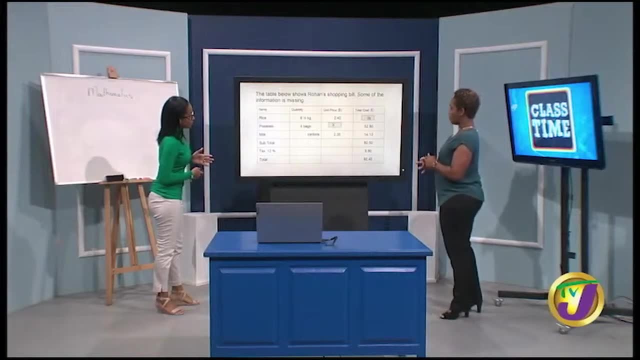 All right, let's try and put the information that we have now in a table. Most definitely So let's see what it would look like. All right, So we have the items, the quantity, the unit price, the total cost, all the information this time. 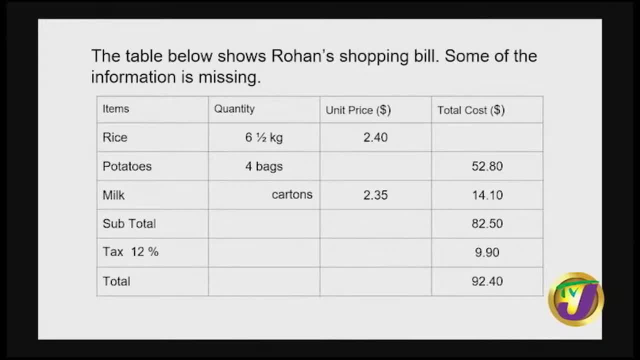 No, but this is what we would have looked at with his problem because he bought. Well, I guess the receipts would not really have on all of this. Yes, remember, you know he bought rice potatoes, milk, and the quantity: 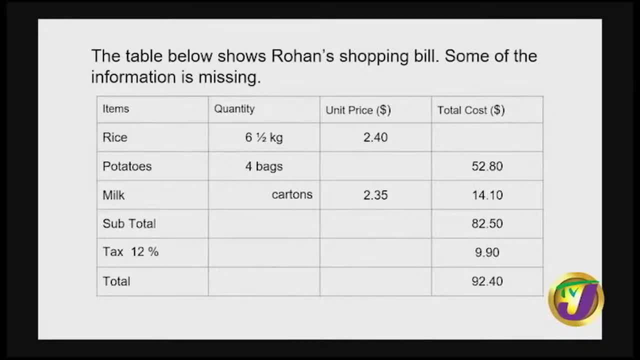 Right and you know we have Pay tax. so tax Right, tax, the subtotal, tax, the total, and we have our total cost on the other column as well. These are the things he doesn't know, these things. 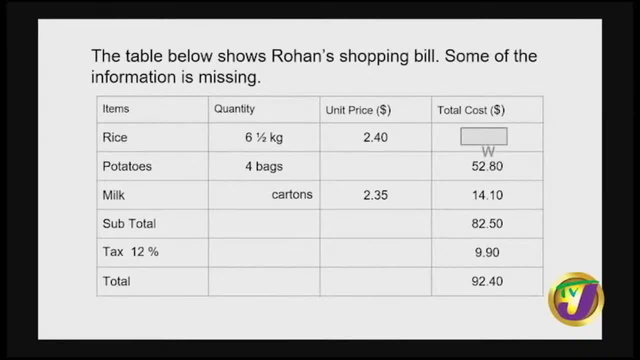 Also, we need to find W, X and Y. Yes, these are the things that are missing, and if him don't figure this out, and if we can't help him to figure this out, He might have to go back to the supermarket. 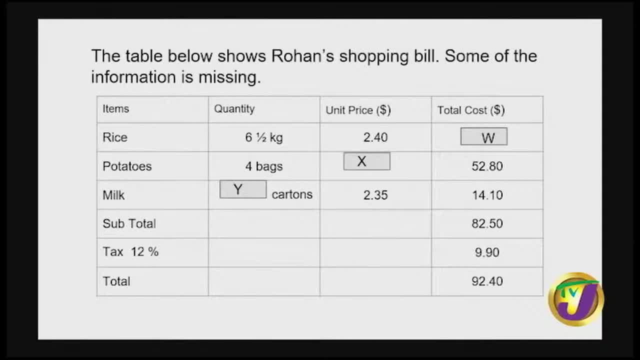 Well, I am sorry for that condition. All right, so where do we go? Okay, so for the rice, We definitely. we have the quantity and we have the unit cost, So we can figure out the total cost for the rice ma'am. 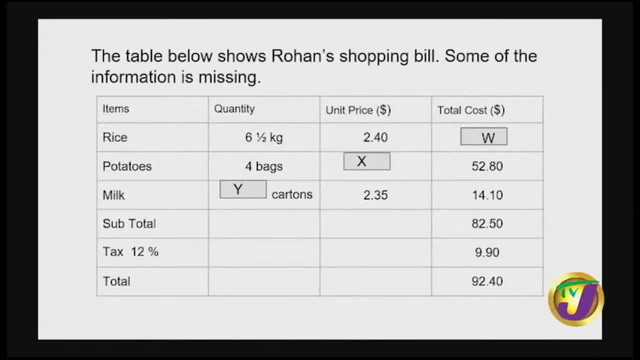 You're sure? Yeah, ma'am, we can figure it out. ma'am, Oh, wait, wait, wait. how are we going to figure that out now? Listen, ma'am, if you need six kilograms, six and a half- even if I don't know how to multiply this- I could add $2.40 six times. 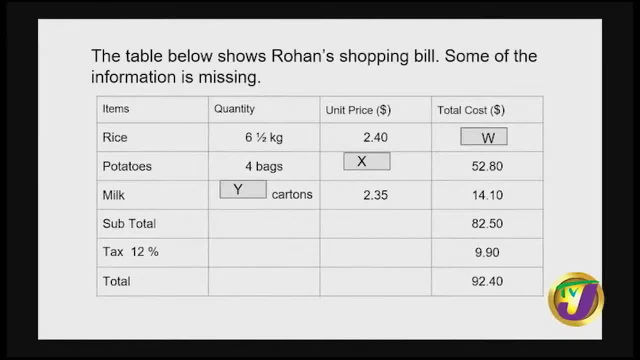 What about the half? I would half it, I would half it and add it to it too. And add it to it too. All right, Because it's half. So we can multiply the quantity there by the unit. So we can do the repeated addition. yes, 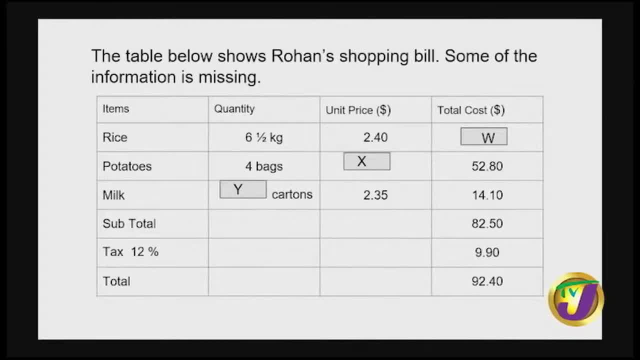 But we can go ahead then to do our six and a half multiplied by our $2.40.. All right, What about the potatoes? All right, so four bags of potato cost $52.80.. Simple something, that, ma'am. We divide $52.80 by four. 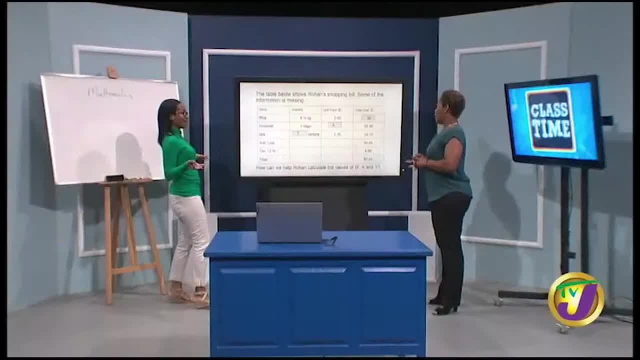 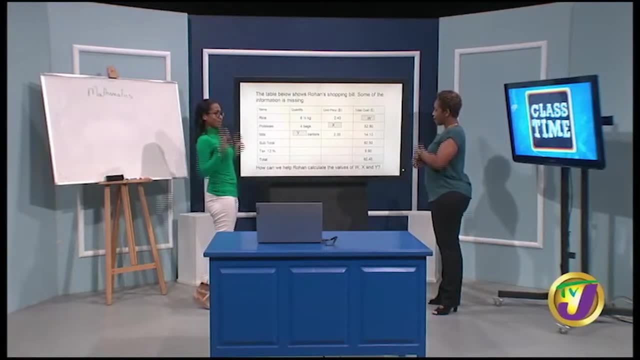 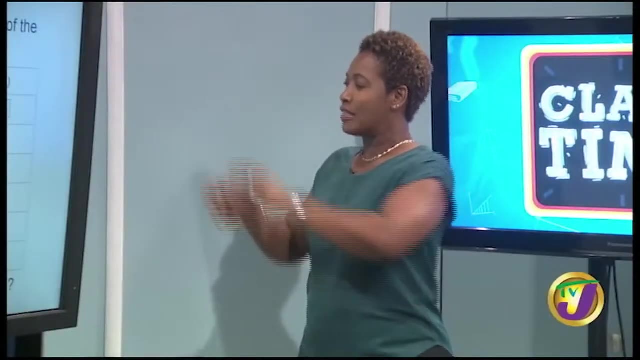 No, sir, Just know. you told us that we're going to multiply the quantity by the unit. We're going to multiply it by the unit price. so how are you going to divide? Because I don't know how much for it, so I can't take it away from it, so I have to figure out how much one bag costs. 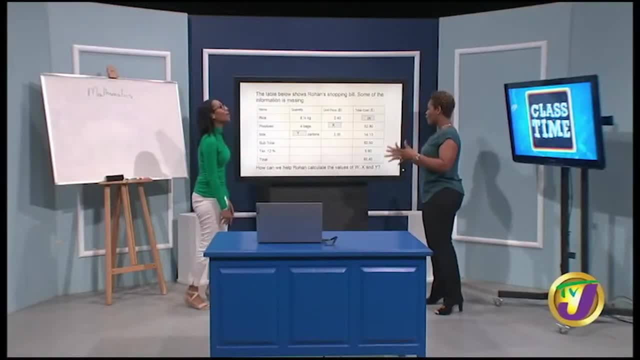 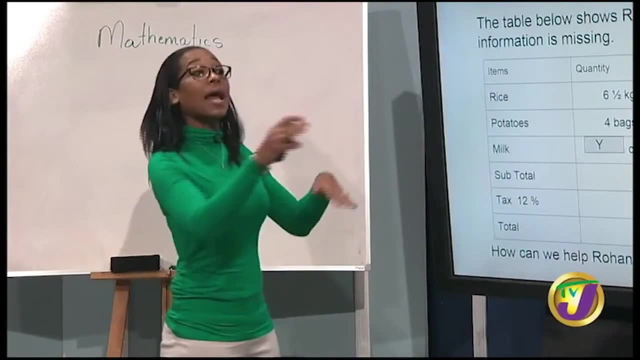 Okay, so it's, four bags cost that, so I have to divide it up into four equal parts. Oh, I get it, I get it. So for the potatoes, I get it, I get it, I just have to divide. 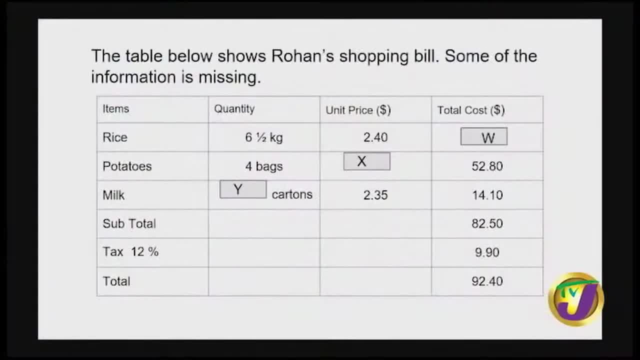 All right, And I can do this milk one. so watch me now for the milk one. Sure, Tsk Boom. I multiply. so I just say: all right, my unit price is $2.35.. My total cost is $14.10,. so I just multiply and I get how much cartons I'm buying. 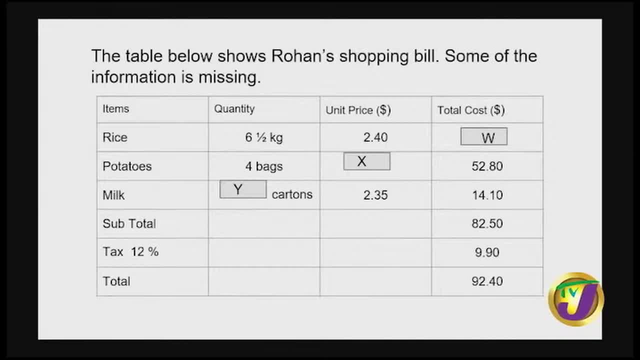 Just like that. Where are you going to multiply? What are you going to multiply again? I'm looking what you're doing in the first one. When you look at the rice, you multiply and then you're going to divide. so now I must multiply. 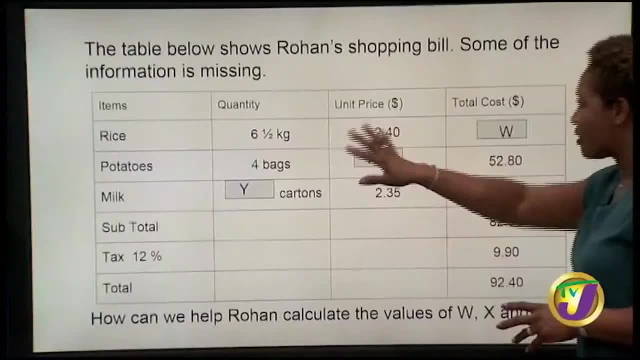 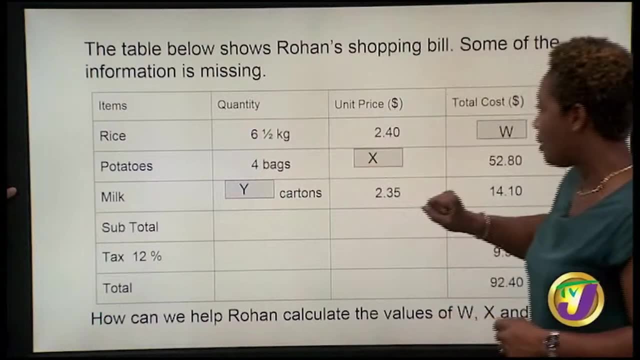 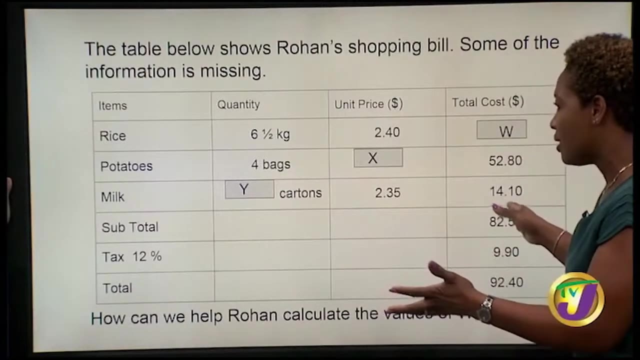 All right, all right, Good attempt, but let's look at the first column, The first. this is column the first row. I have information in this column and this column. Look at yours. Even the information layout is different, Oh. 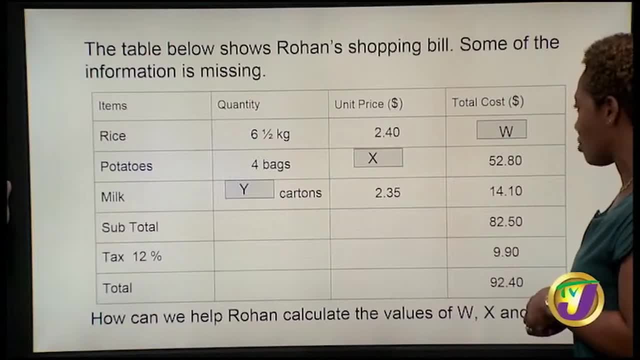 So I can't use that same method that I used for the first row. Okay, so for the milk, we have how much you actually spend. So this is your total. Oh, so the total two, And this is for each carton. 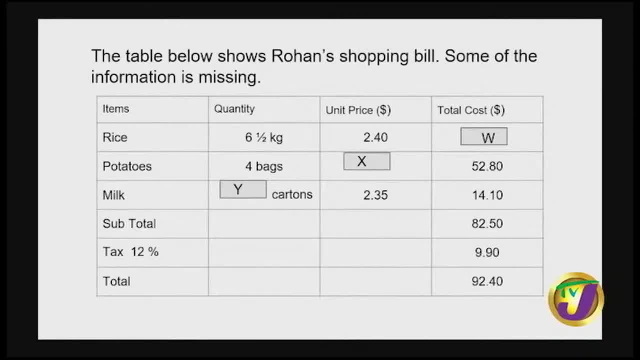 Oh, okay. So So now that you should understand: mama, Mama you have this, ma'am You have this, So wait there, wait there. So if I cannot multiply because I don't have a carton, Okay. 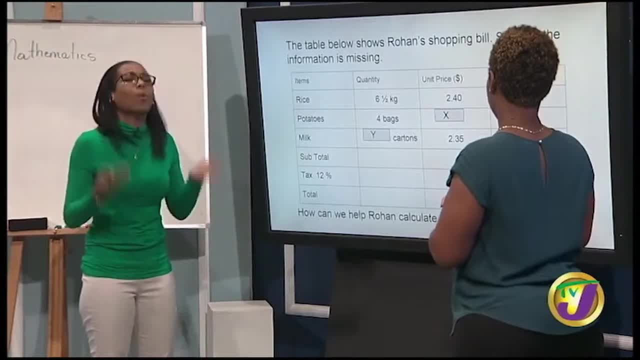 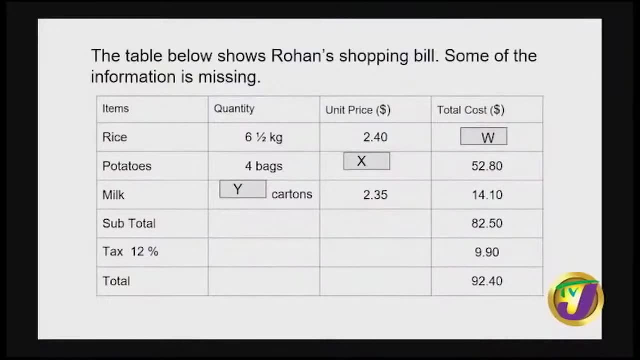 So I can't multiply? Oh, okay, because I don't know the quantity, and the quantity is what I need to know. but I know the unit price and I know the total cost. All right, I'm going to divide, I'm going to share it, I'm going to split it up then. 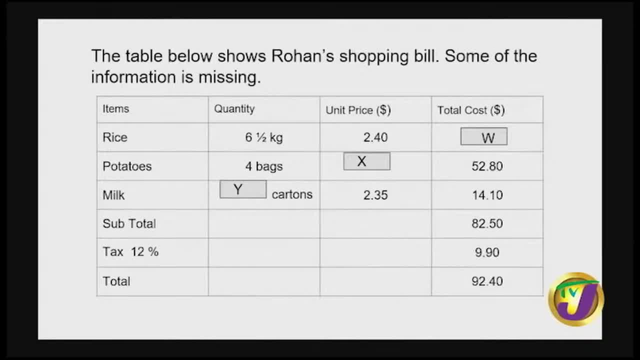 That's correct. So if you divide your $14.10 by $2.35,, you definitely will get how many cartons you would have bought, And we can help Rowan to figure out what W, which is the total cost of the rice. 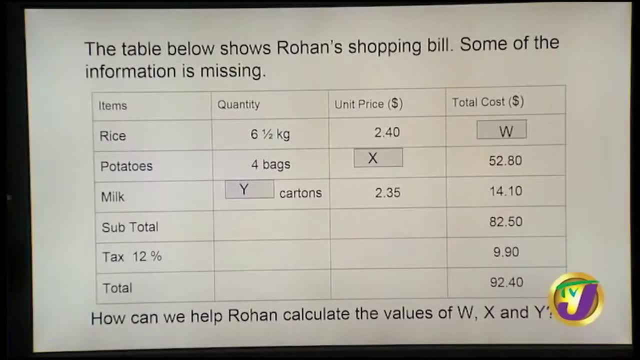 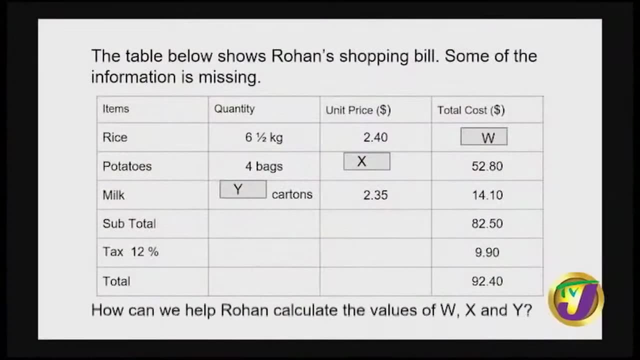 what X, which is the unit price of the potatoes, and what Y, which is how much cartons of milk he bought. So let's take a look, because we had helped him. so let's look what we did. So we multiplied $15.60. 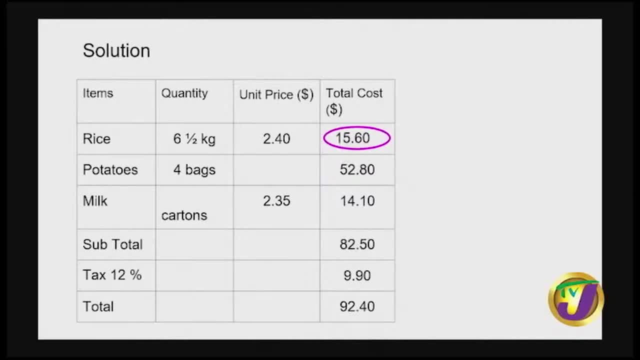 Great. so that would have been our total cost for our rice, which again is W Correct, Right, and then here for our potatoes. We would divide $52.80 by 4, giving us $13.. Yes, and $20.. 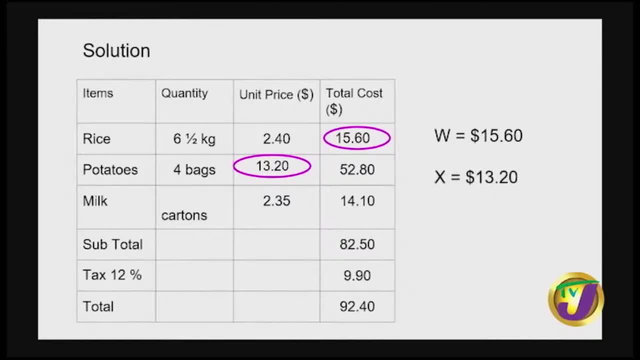 There you go. Great, which is X And 6.. So if you divide $2.35 into $14.10,, you would get 6 cartons of milk, And when Rowan looks at this, him can stay home now. 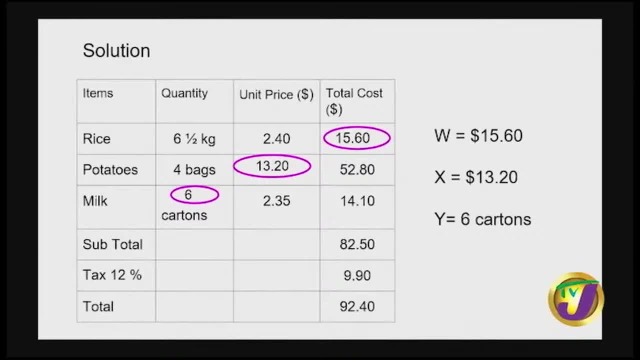 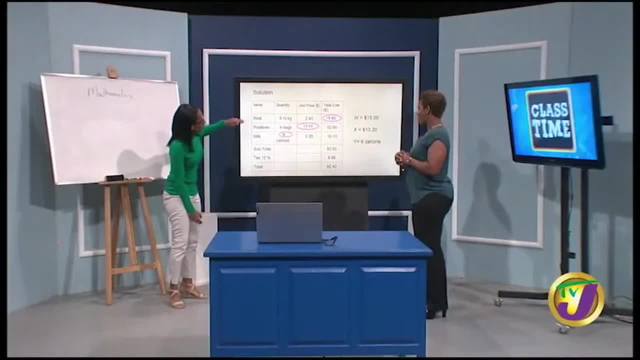 And him can add it up on him own. now Him can check it to see if everything worked out. Yes, I remember we spoke about checking it. There you go. Good, so right here we have the Because, Right, He adds up and see if all things come up to $92.. 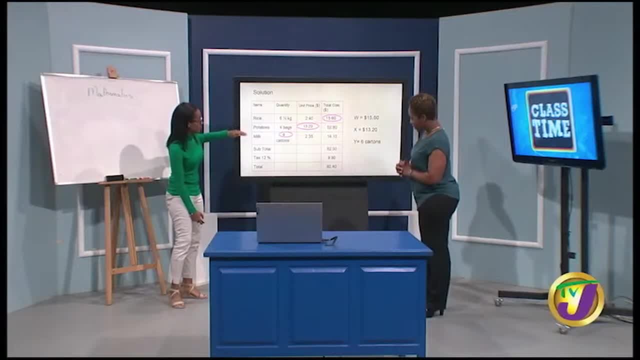 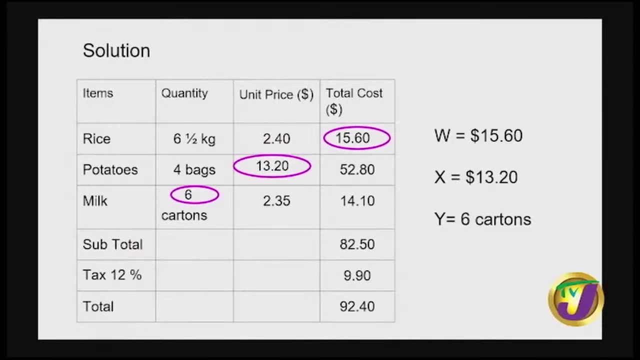 $92, go the rice, the potatoes, the milk And then of course add in tax Right to the subtotal, Of course, To get the total Most definitely, And he can check if him tax right to him, can check if 12% of $82.50 is $9.90. 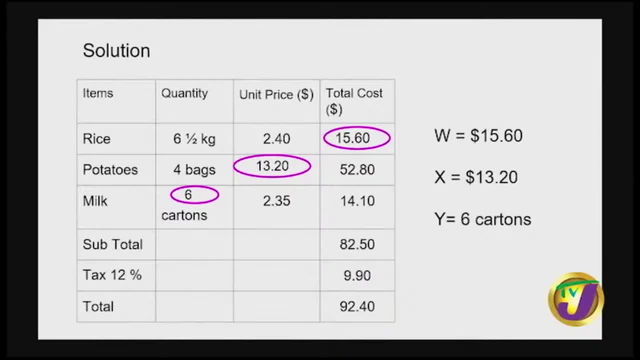 To see: all right, it's really 12% tax, I paid, All right, so Joel's wife- $98.. It's not Joel's wife, man. this one is Rowan's wife. Oh geez, Joel loves peanut butter. 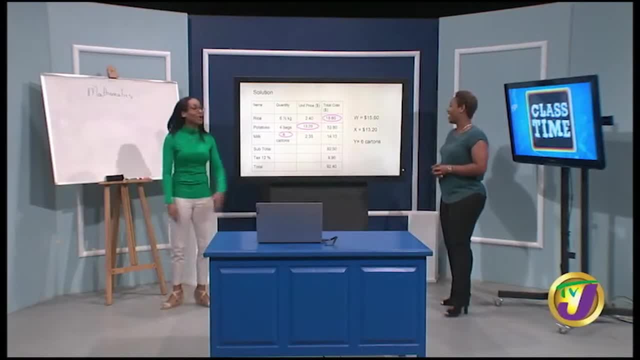 Boy, these people just crossing over. Yes, man, Them full of problem, I'm telling you, They just crossing over. Joel have problem, Joel have problem and now Rowan have problem. Them full of problem. Rowan problem solved now do. 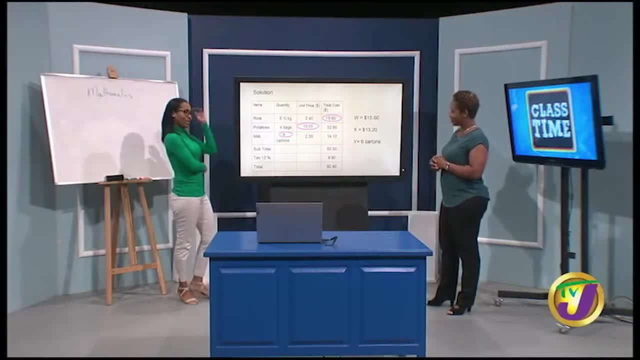 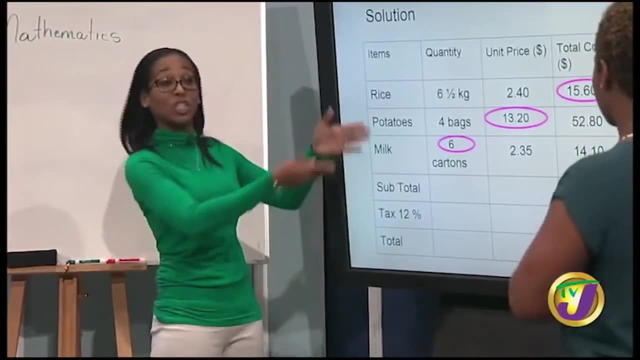 We help. yeah, we're helping them to solve their problems. But what do you think we use to help Rowan to solve his problem- his blurry receipt problem now, Because he had a problem and we help him solve the problem and we check it. 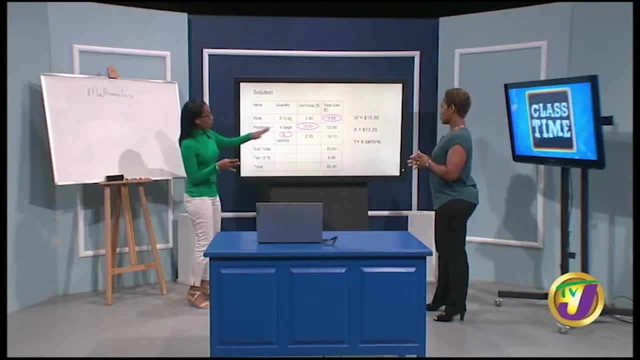 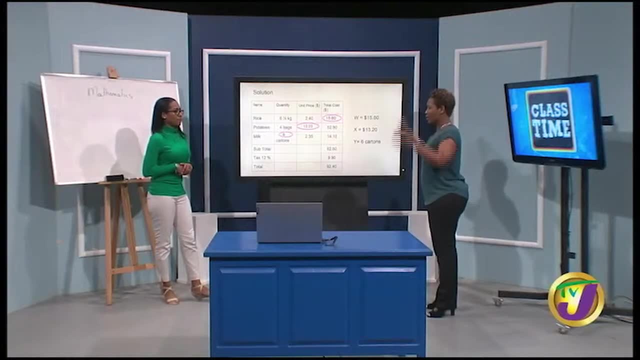 We help him now to know how to check, to see if- all right, what you would have figured out. if it's right, Well, when you know, when we first looked at, When we first looked at the problem, when it was written out like that, it wasn't so easy to see how they are linked. 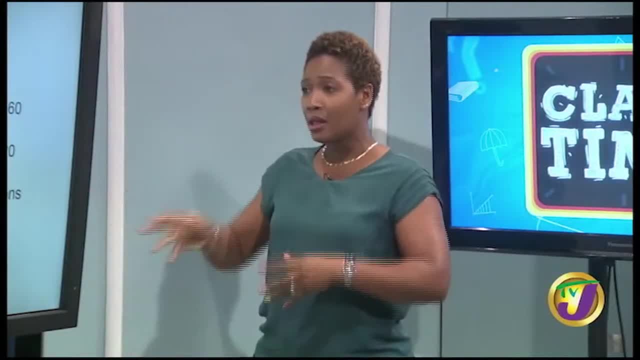 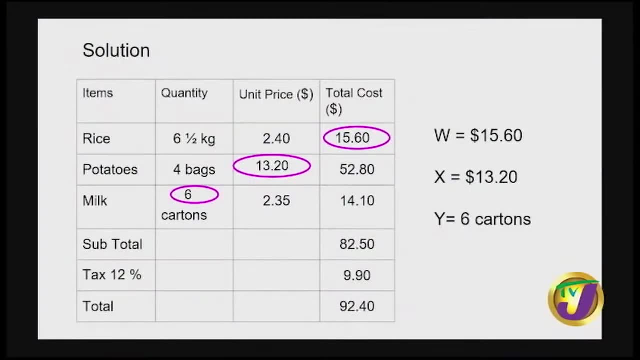 But as soon as we dropped all that information in this table, it was so much easier to access the problem and solve And simpler to work it out, don't it? Much better, Much better. So we made a table. We did make a table. 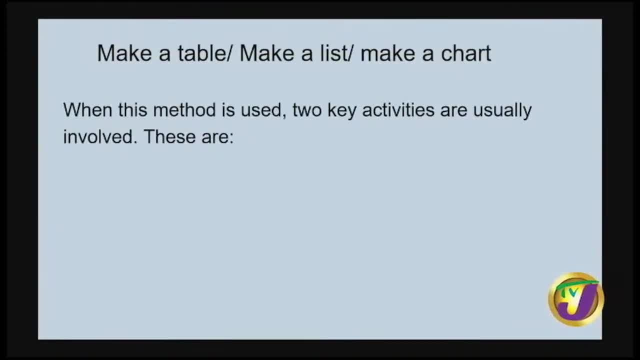 And sometimes I guess we can make a list. We can make a list and we can also make a chart too, But in this case we looked at creating our table. That's right, And when this method is used, two key: 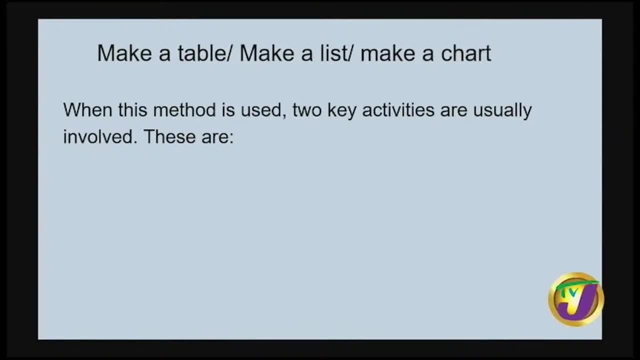 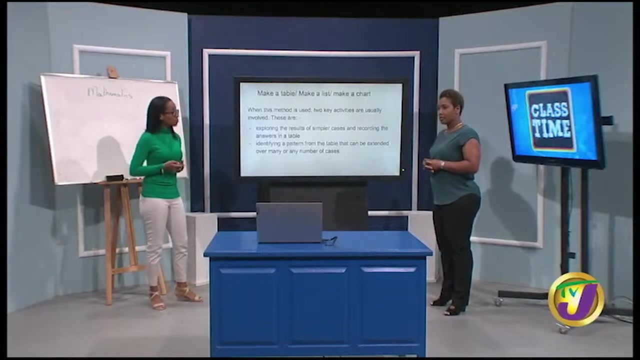 Activities are usually involved. These are: one: exploring the results of simpler cases and recording the answers in a table. Two, identifying a pattern from the table that can be extended over many or any number of cases. All right, So far. again, we're looking at problem-solving strategies. 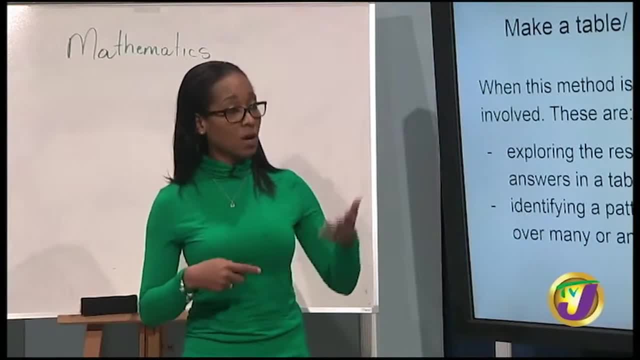 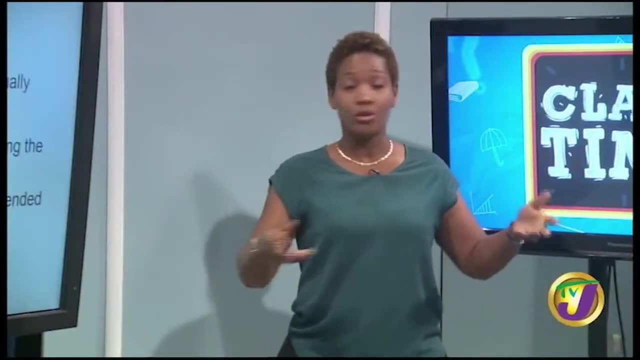 and we're looking at the process in understanding, planning, solving, checking. I'm hoping that they understand fully by the time we finish. So just to remind for those who are just joining us or for those who were there and probably a little bit distracted. 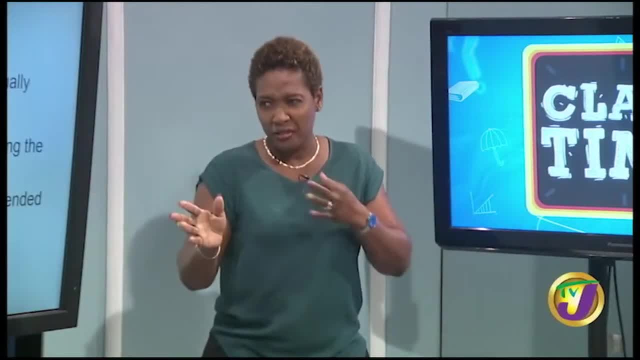 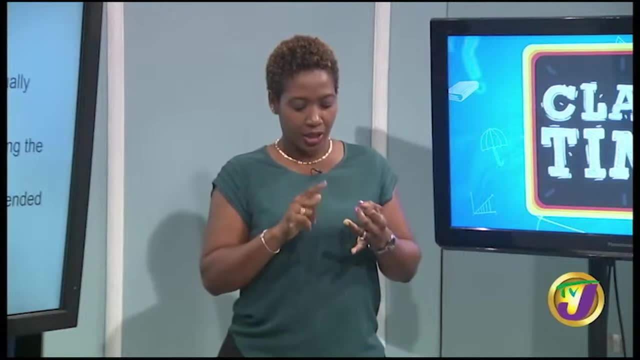 just remind us how we went through three problems, three different scenarios, and we helped everyone. So we had Juno with a farm coop. We did what We worked backwards to arrive, All right. And then you had Joe with the peanut butter supermarket. 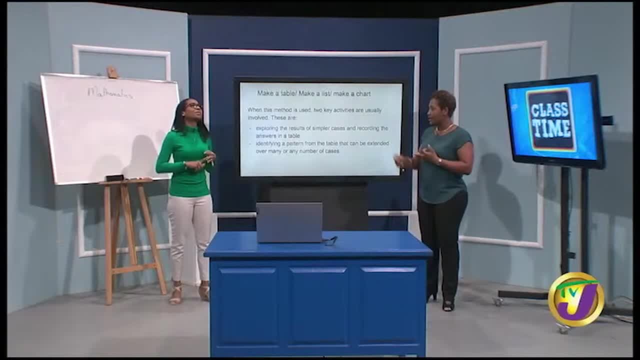 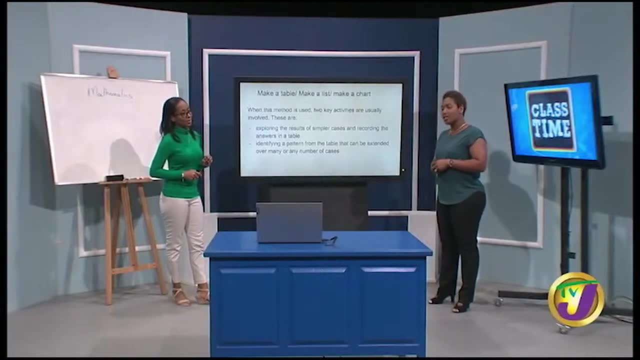 We did logical reasoning- Excellent. And Rohan and his wife We did making a table. There you go So far. So far, We gave them three different strategies, Problem-solving strategies. So you know we're good to go, man. 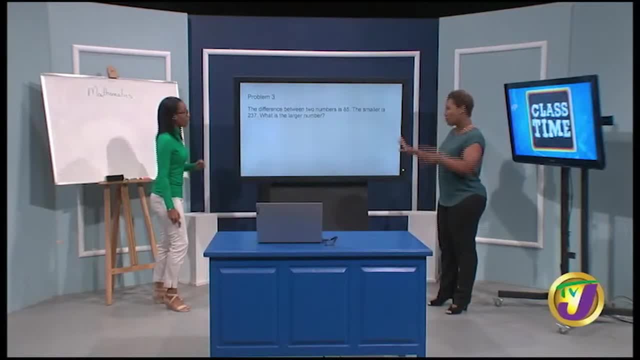 It's all, Lord, another problem. Today's just the day full of problems. Come on, you don't look so bad, though, because it was two lines. All right, Let's see. The difference between two numbers is 85.. 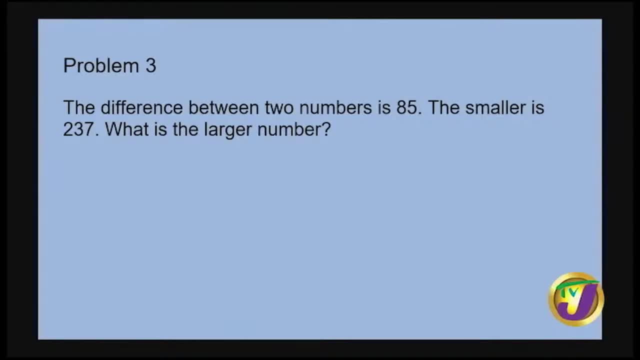 The smaller is 237.. What is the larger number? So we're given three options: A 152.. B 312.. C 322.. All right, So just before we even touch this, there are problems. Several problems may exist, but some problems may be easier for depending on your age and 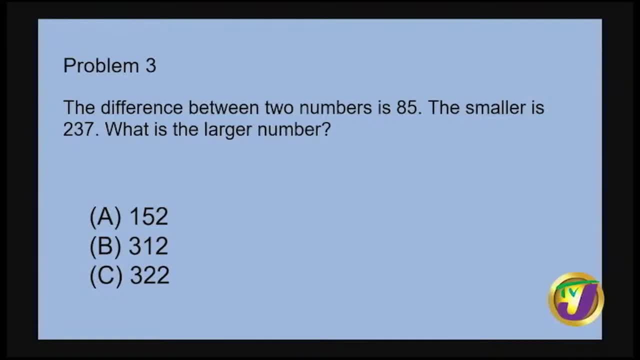 experience to look at and solve. But let's say we gave this to a 10-year-old. It probably be a little a little difficult for them to, and maybe not, you know. you never know- because it depends on their experience again. 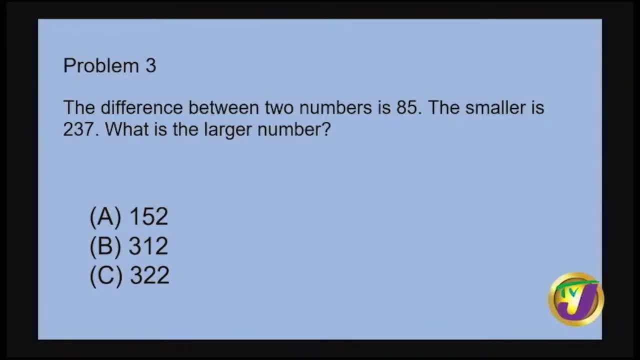 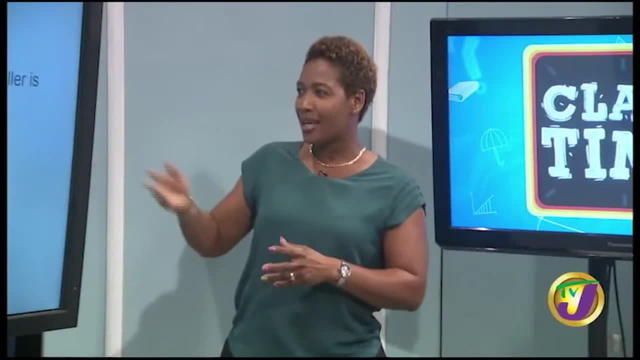 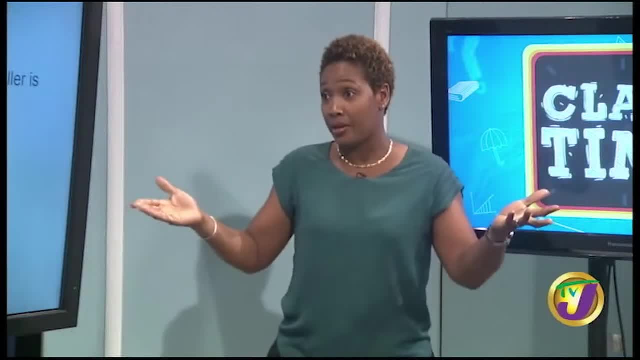 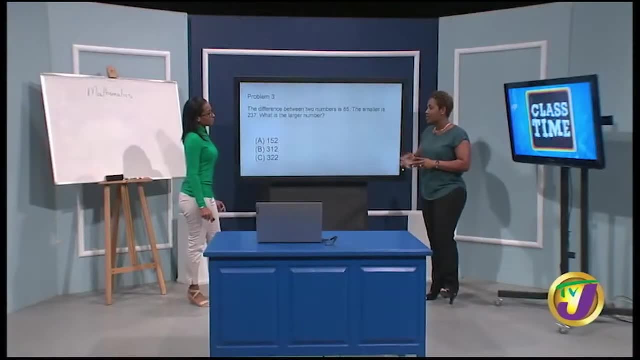 never know, because it depends on their experience. again, Yes, But let's look. There are some words that I think I'd have to understand in order to get to it. For instance, the difference, Great Difference. What is the? what am I talking about? 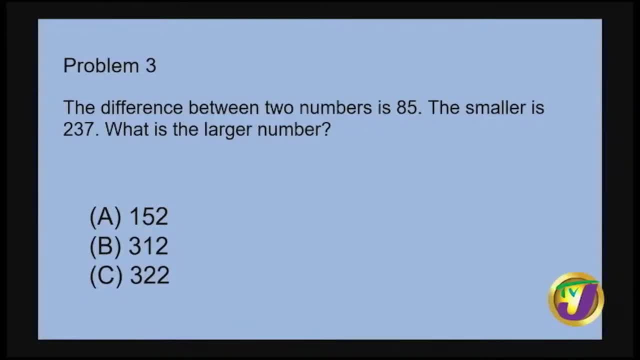 Um, difference. I'm different, You're different. Oh, yeah, Yeah, that's what you're going with. Yeah, Math, difference, Math. Oh, oh, oh, Math, All right, in math now, and we're looking at the operation, we're looking at, you know, subtraction. oh, thank. 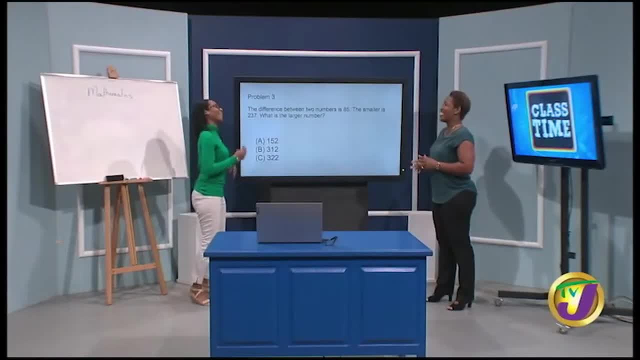 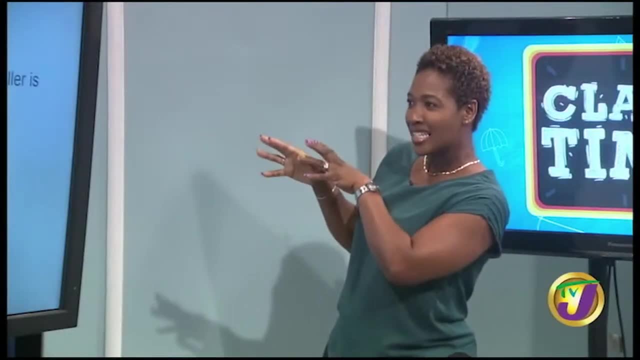 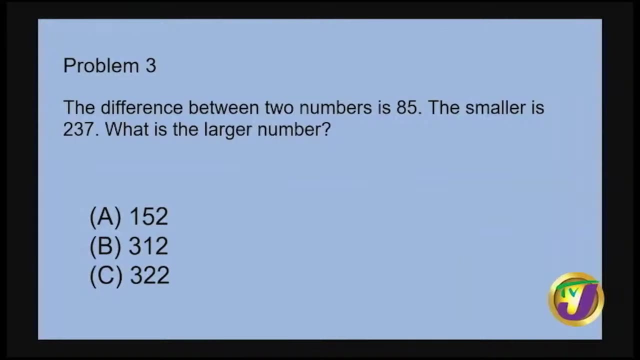 you, you different, i different, yeah, right, so difference in math. we talk about subtraction. right, that's the operation. the smaller is the smaller number here. yeah, this is 237.. so that means a cannot be an option. all right, a can be an option. 152 is not smaller than 237. 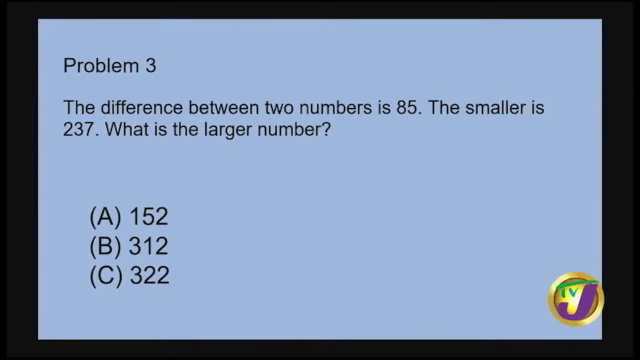 i realize that you're using, you understand the problem and you're using what you know and you're guessing, but continue, that's what i'm doing, man. so what is the larger number? so clearly, if them just give me two options for things. so since 322 is larger, let's try that 322 is larger. 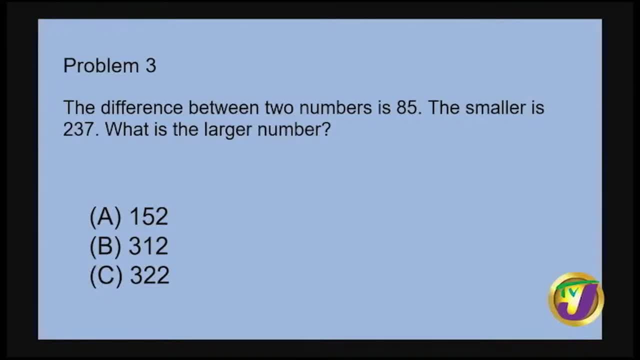 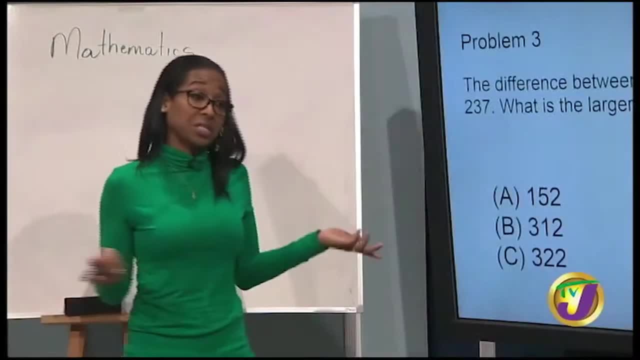 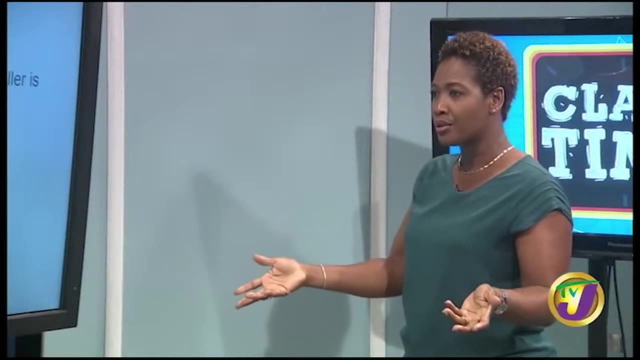 yeah, so you're guessing, of course. so how you're gonna check if you're right. so your guess how you're going to check, because i, i want to guess and i want to say b 312.. you're saying it's c. how can we figure out? i'm going to subtract 237 from the 322.. so not that you should say a long. 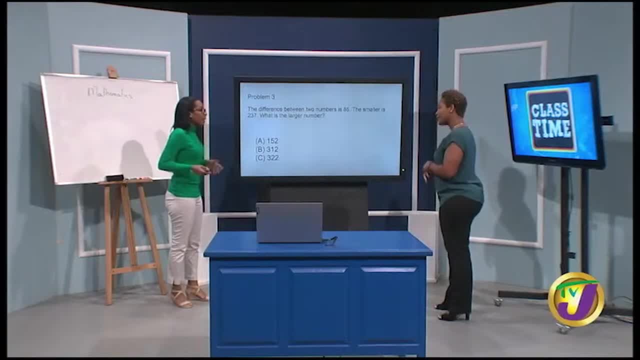 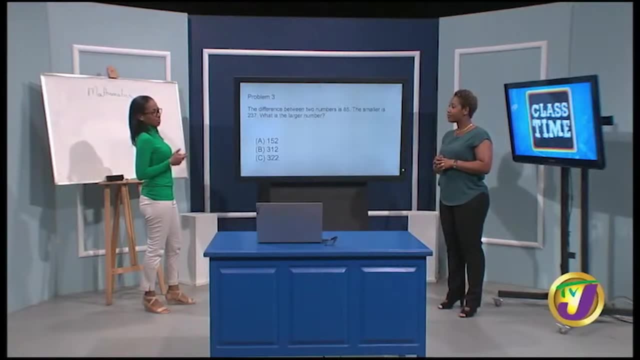 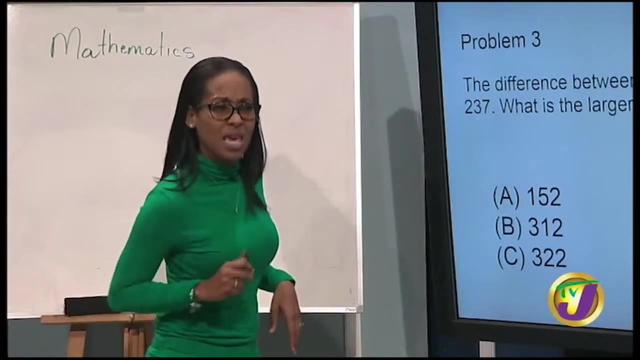 time, how else was i going to get 85.. that's why i need to know something. but what if a child then wants to subtract, still guessing, but wants to check if they're right? so you're guessing, you say c, the circle c, i guess, and say b- i certainly want me to check it first. you're checking it. 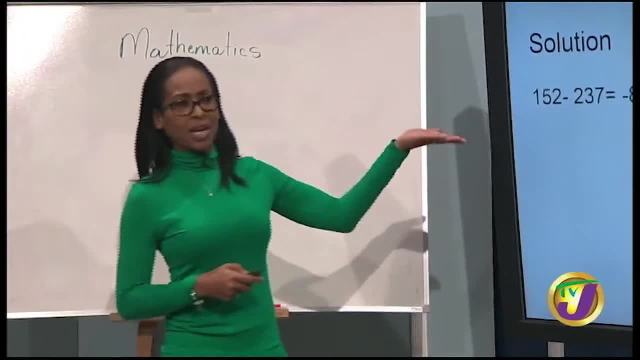 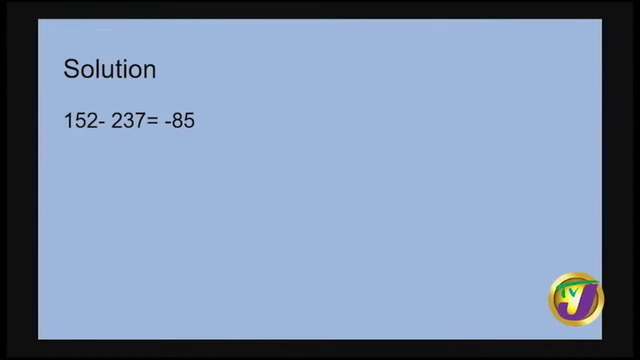 so let's check it, okay, so we wouldn't get, we definitely. well, i didn't. don't say 152 can't work, right, so the 152, i would not have it. i would not have guessed that. whoops, he's out of here. that's right. all right, let's look at the 300. oh lord, so my answer wrong. so the 312 can't work. well, i'll. 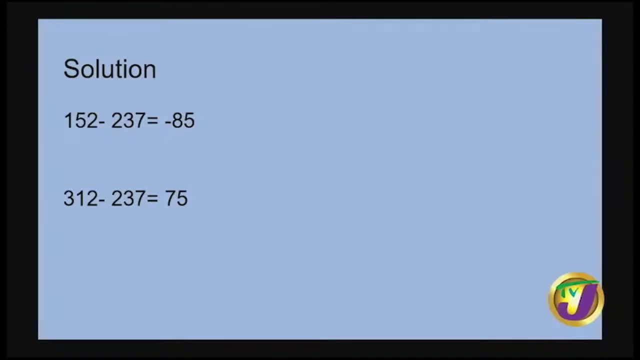 just go with the bigger number because it's a. it had a bigger number, oh well, all right, fine, you get it. you get it. so our answer is definitely 322.. and it's obvious what we had used to figure out this one guess and check. you just checked it, yep. 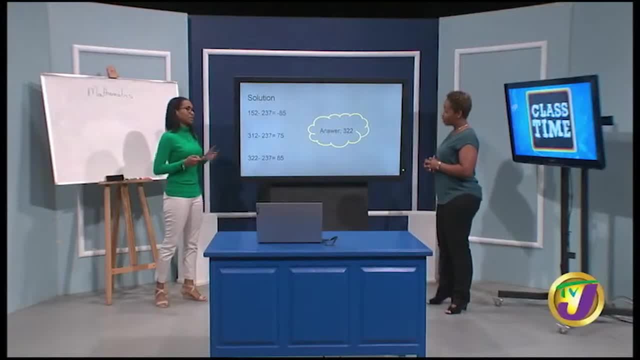 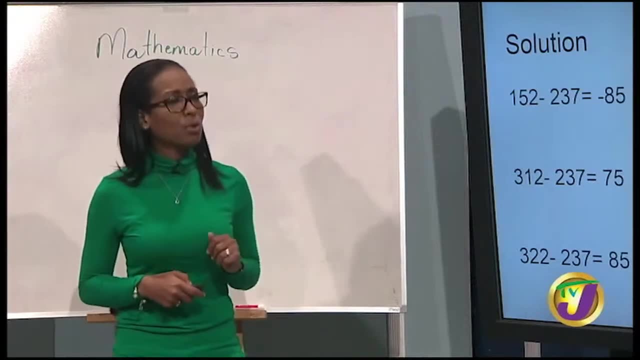 and we guess and we definitely checked it. so that's another method and you know this method. they can use it too with when they're doing the multiple choice. most definitely, yeah, man, they can use it when they're doing multiple choice questions, but let's not always use guess and check though. 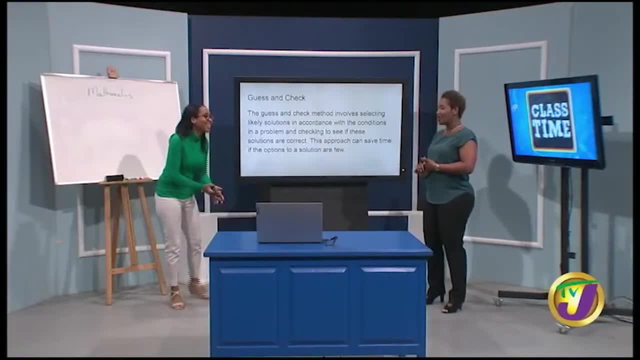 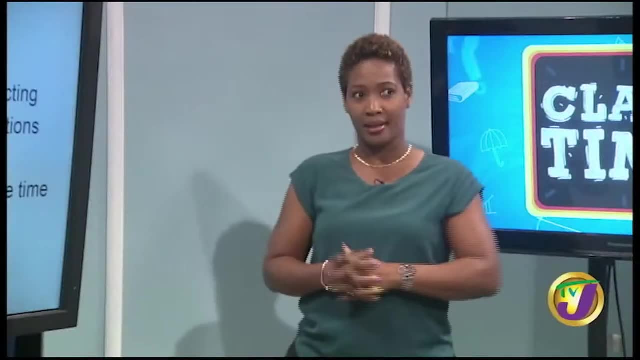 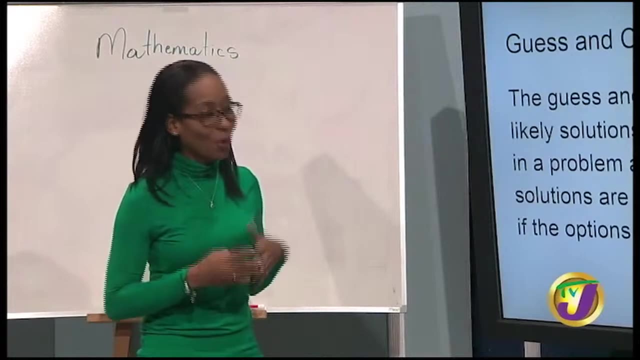 which is true, stuck, or you. you have a little clue, you know, you give out, you you have a idea of what and you're down to like two. you may want to guess and check, but let's not guess and check all four options. no, not at all, not not going to work. so we're formalizing the guess and check method now. 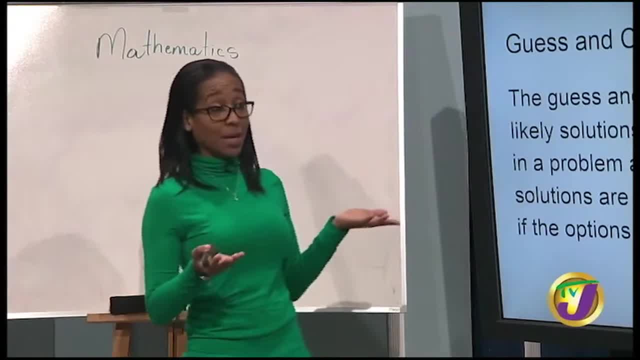 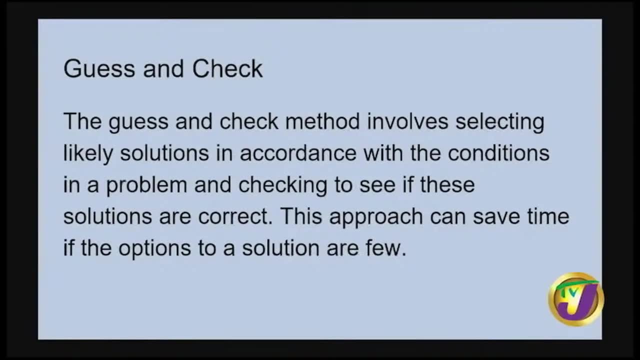 and it involves selecting likely solutions, which we did with the conditions in a problem, and we checked to see if these solutions are correct. and we did all of that and this approach can save time if the options to a solution are few, there you go, you realize that keyword and few and 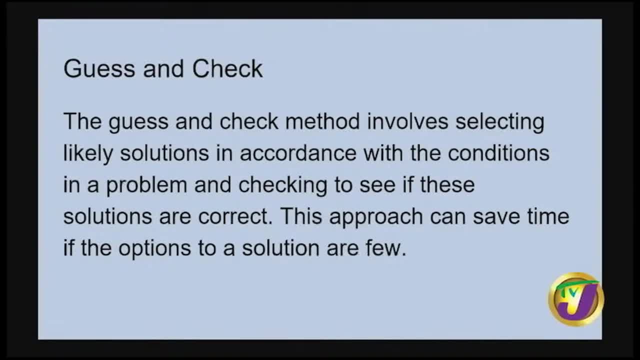 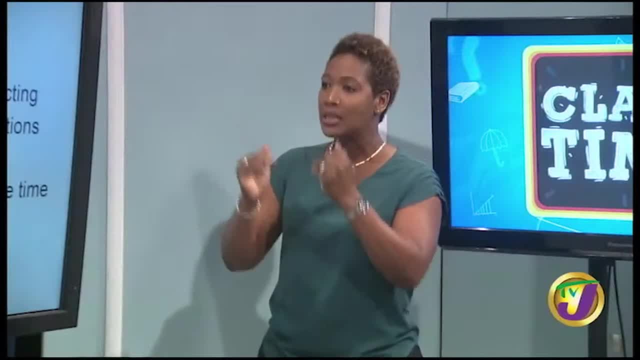 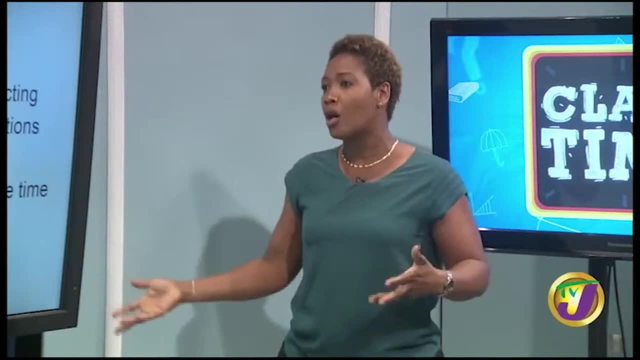 and checking. really we did all three options, but we would not have chosen 152 because they did state the problem. this did state that 237 was a smaller value. great, so to save on time, you would not have chosen the 152 because it is not smaller. it is not larger than the two cents- 237, right and 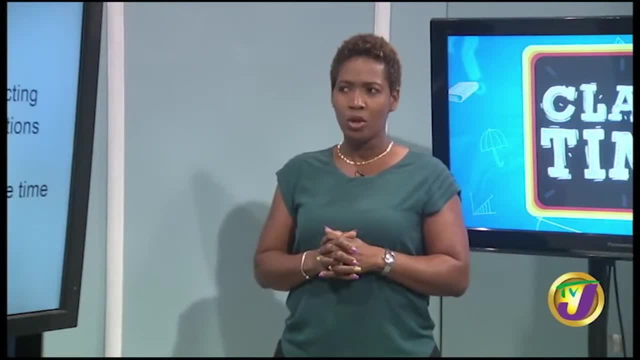 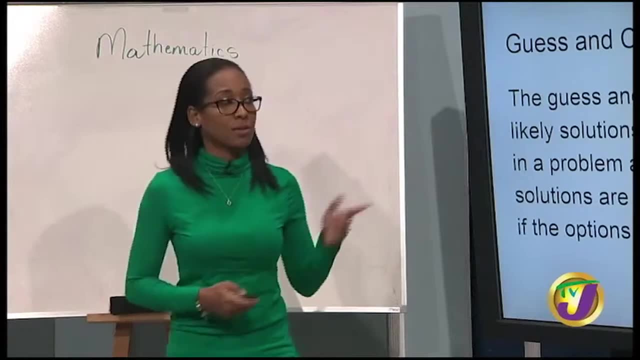 you realize too that you have understood the problem most definitely. so that is very important. The understanding part we have to definitely understand before we can do anything else. So let's take a look here at the problem. So Kenny equals squaring numbers ending in 5.. 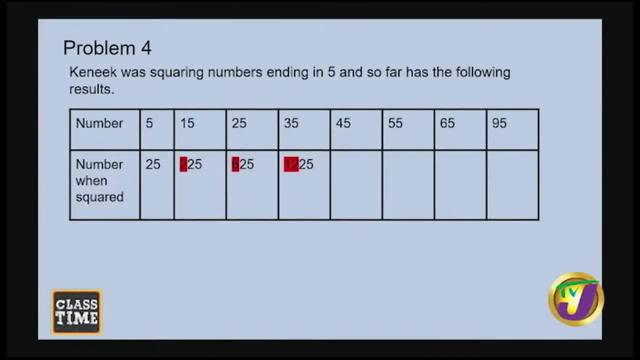 And so far he has the following results: So we realize row 1, number. So we have 5,, 15,, 25,, 35,, 45,, 55,, 65. And we end at 95.. All right, 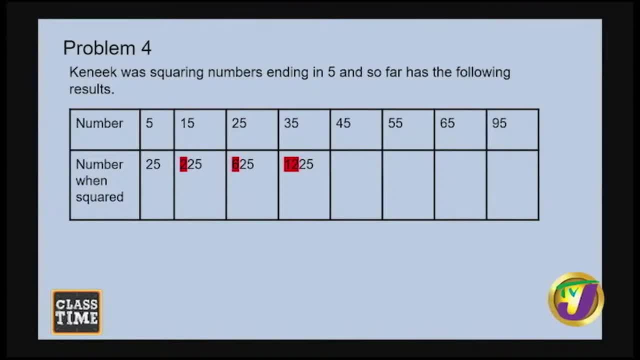 And we realize number when squared. So 25.. 5, 5 is 25.. 15,, 15.. 2, 25. 25,, 25.. 6, 25.. 35 times 35 gives us 1,225.. 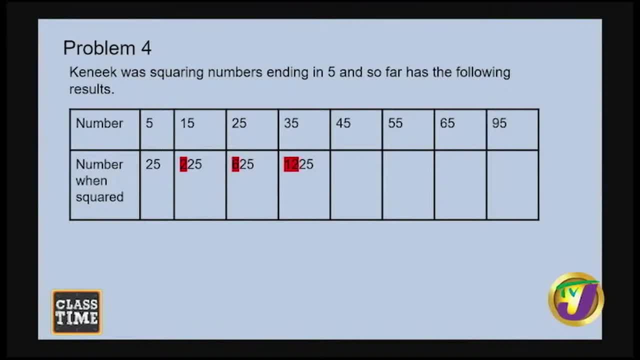 All right, I can't help you with numbers. I get what you mean because you're reading what is in the row. You're telling us That's fine. Look how smart I am. I'm happy that you're reading it with understanding. 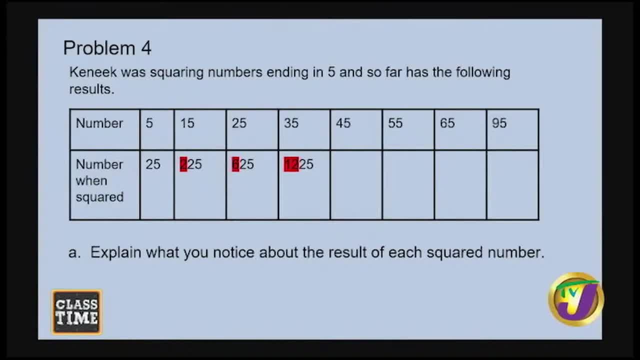 So let's look at A. Explain what you notice about the result of each number squared. I don't want you to tell me that when you multiply, or you multiply the number by itself, you get that answer below. Oh, you don't want me to tell you that. 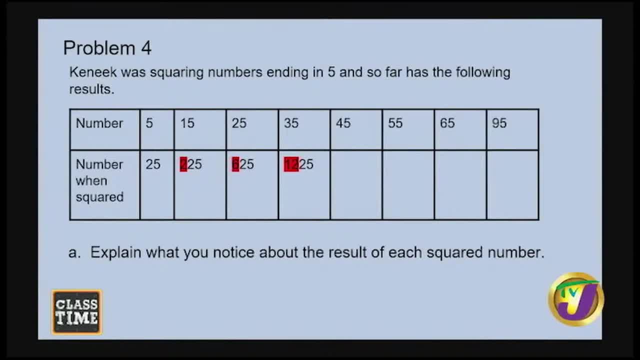 No, no, no, no, no. Look again, man, and tell me what you notice, And hold on. Before you do that, I'm giving you two more Okay For you to think about. So the next one is: you're going to describe a relationship. 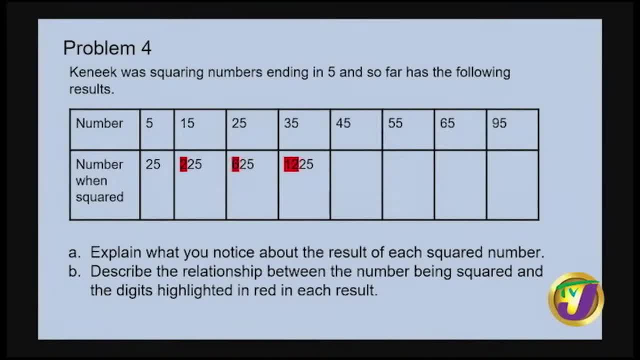 between the number being squared, or your face changed, And the digits highlighted in red in each result: The number being squared. So you're talking about the 15 and the 2.. The number being squared Right, which is the 15, the 25, all of those numbers being squared right. 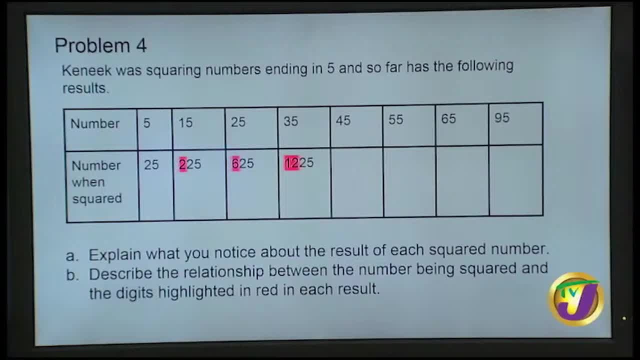 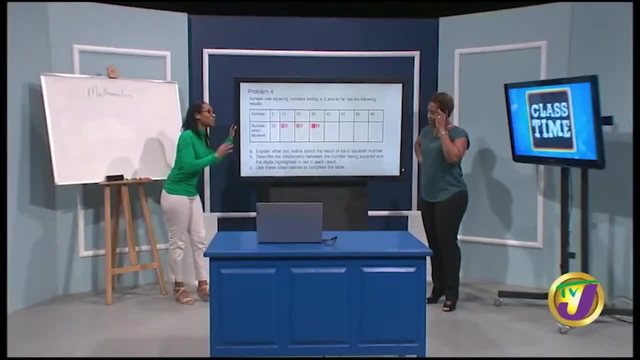 And the digits highlighted in red. Great, No problem, man. And this one, though- And I want you to after you figure it- I wish the viewers were able to see your face to wonder what's happening. Now, when you figure out A and B, you're going to use it to complete the table. 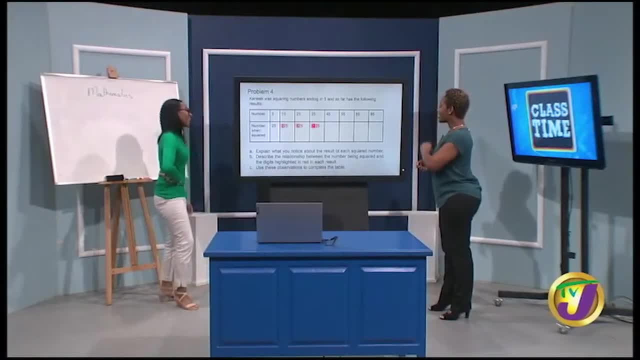 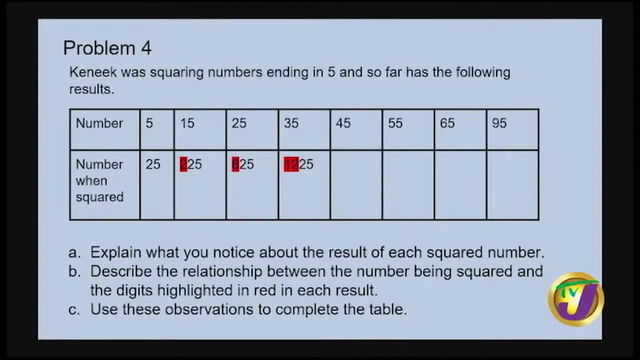 Let me figure out. B must figure out, Okay, Okay, Explain what you notice about the results of each squared number. All right, This easy. you know It. easy, man, but I'll even you. I'll even you. 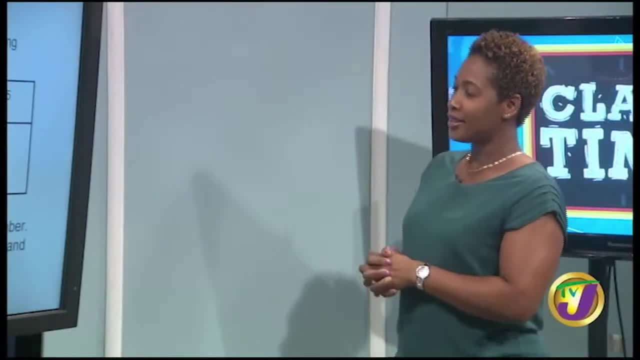 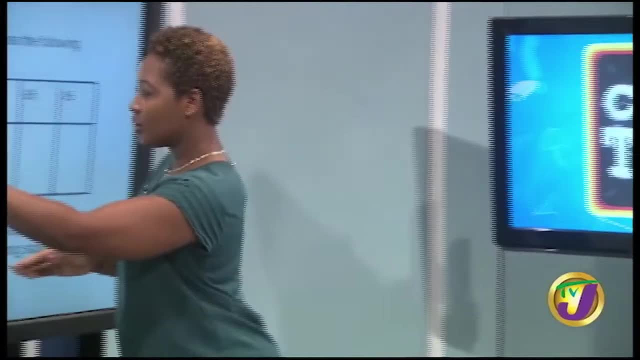 Try and figure it out. Explain what you notice about the results of each squared number. All right, We're giving you time, Hurry up. no, Okay, they all have 2 and 5.. All right, They all have a 5.. 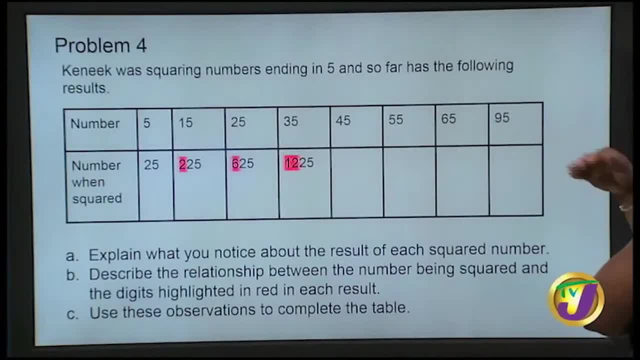 But they all have 2 and a 5.. So they're all ending. They all have 2.. 2, 5., 25.. 2, 5.. All right, One. So you're picking up something happening. 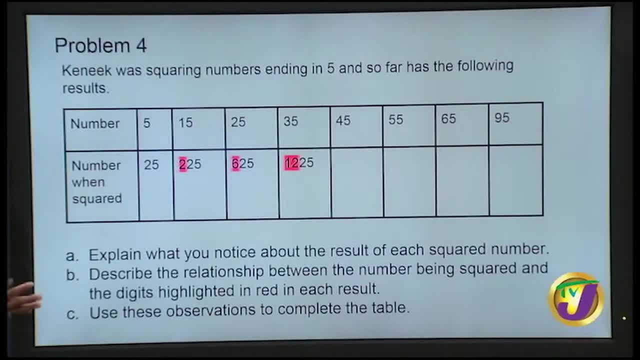 All right. So the next one going to have 2, 5 at the end. So all of the others, 2, 5.. 25. Oh, you're definitely sure that they will have 25.. They'll have a 2 and they'll have a 5.. 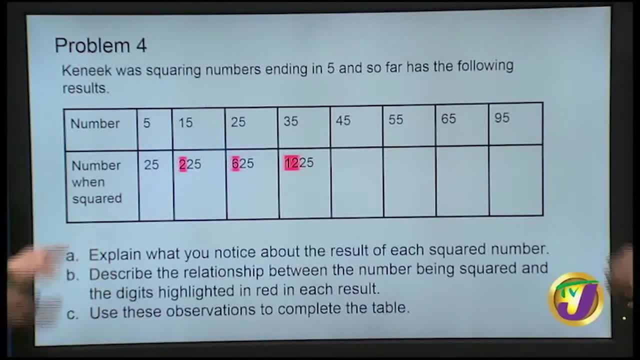 25.. I don't know What do you mean? You don't know, but you are able to tell us They all have 5. Isn't it? All the numbers have 5. So clearly we're squaring the 5.. 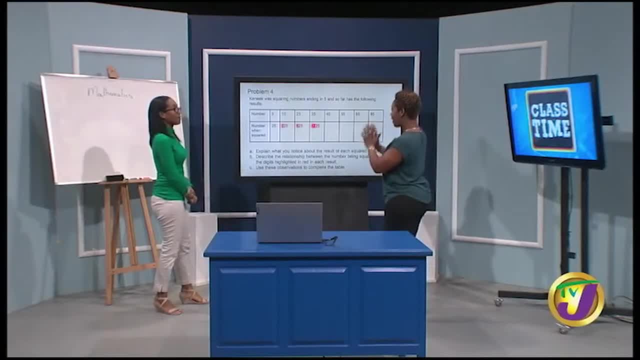 Great. So what you're picking up, then I'm going to give you a little hint, I'm going to give you a little hint, I'm going to give you a little hint, Nothing else. You're not picking up anything, No, 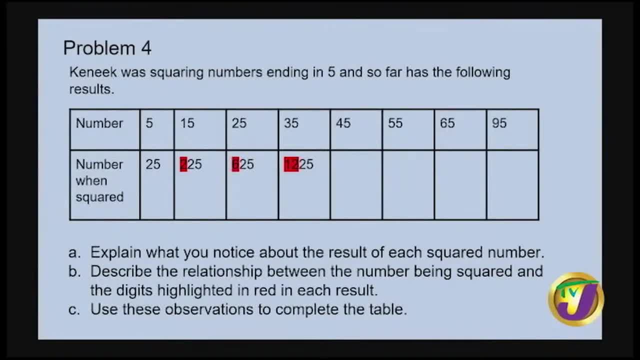 All right, Not a problem. No, I want you to use You're going to look This relationship you're talking about. Yeah, man, You need to tell me the relationship. I need to hurry up and tell me the relationship too, because I give you too much time. 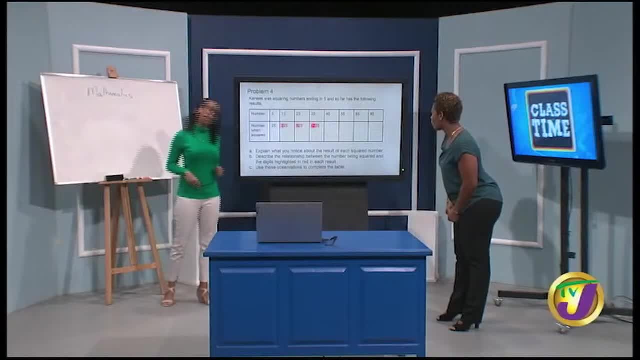 Come on, Figure it out, Figure it out, Come on, I'm sure the grade 10 student are told: no, Figure this out. I don't see no relationship. You have 1 and 5 up there, You have 15.. 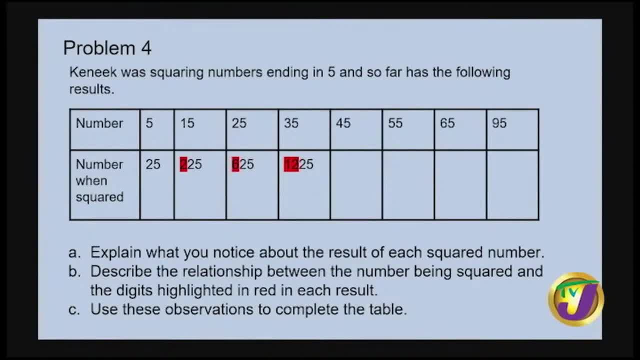 And then you have 25. And then you have 25. And then you have 26. And then you have 27. And then you have 28. And then you have 29. And then you have 30. And then you have 24.. 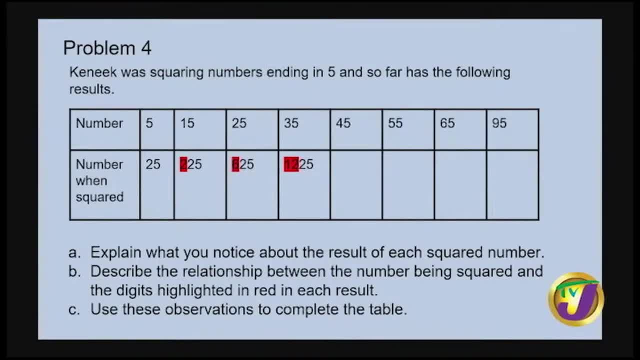 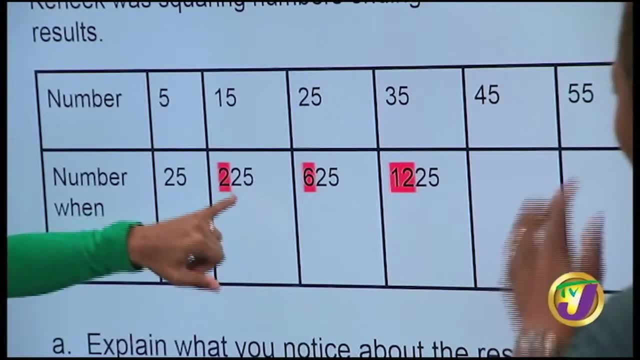 You have 15.. And then you have 2.. All right, So watch this now. So you would have said the last two digits when you're looking at each number: Yes, Would have ended in 2 and 5.. Uh-huh. 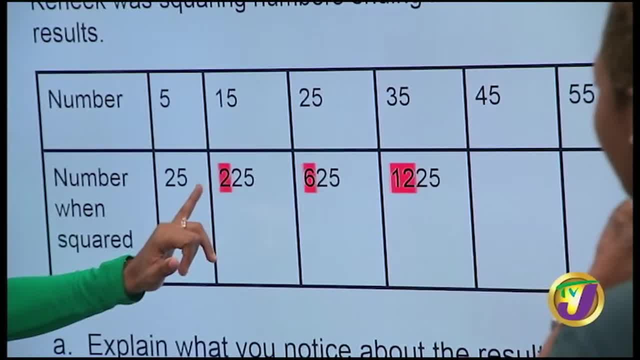 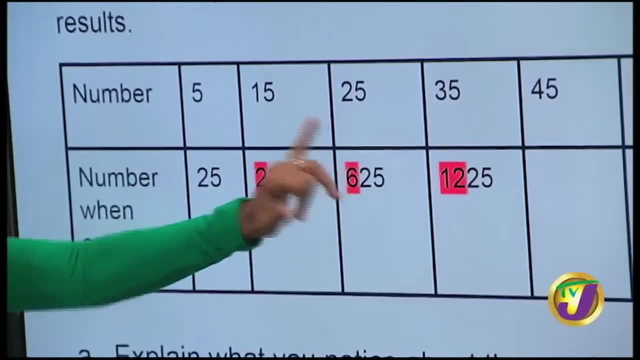 25- right here, Right, Right, Right. But now you're looking at the 2. Uh-huh- Right here. But then, when you're looking at the number up top, Uh-huh To be squared And the number following: 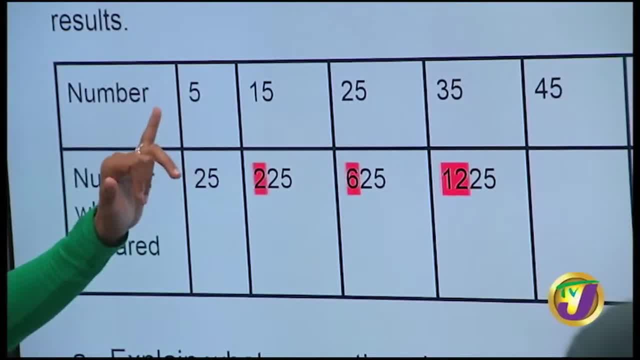 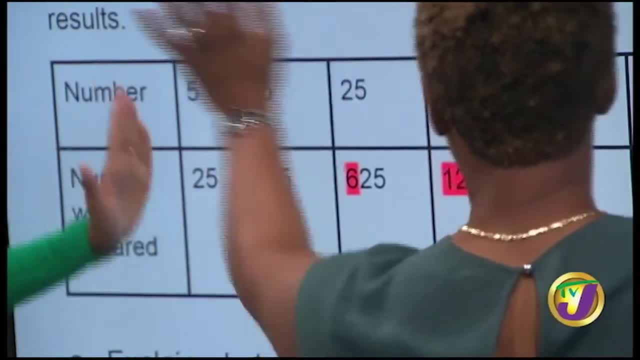 What you realize about the digit in the tens column. Look and tell me: Sure, I'm giving you a hint. Okay, So you have 1.. Ignore, Ignore this one. So you have 1.. Uh-huh, Then you have 2.. 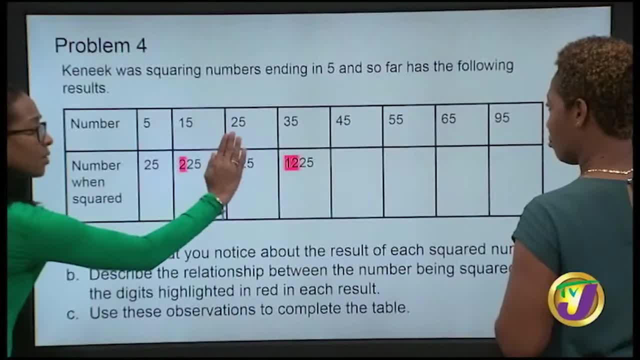 All right, Then you have And look at the relationship, Hold on. So just look at the 15. The 25. And look at the 225.. So you would have already told me how you arrive at the 25. The 25.. 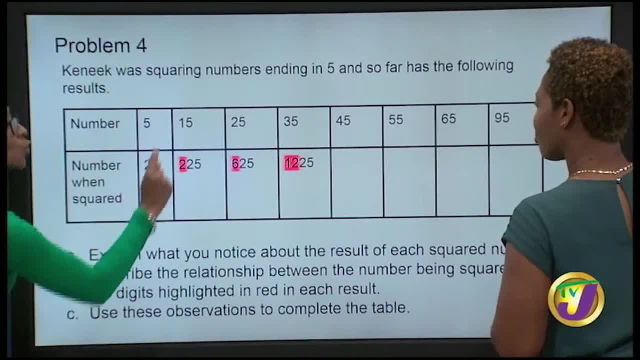 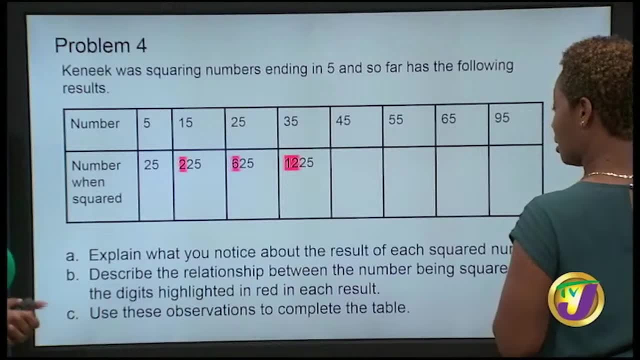 Right, Right, But I highlighted 2.. So I want you to look at: 1. What is in the tens column Great In 15 and 25.. And tell me how you can get 2.. 1. 1 times. 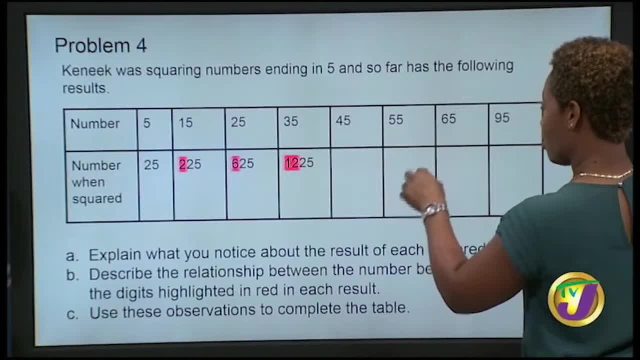 1 times 2 is 2.. All right, But watch it again. Do it now for 25 and 35. And tell me if it works. Um 3 times 2 is 6.. All right, And there's a third number there. 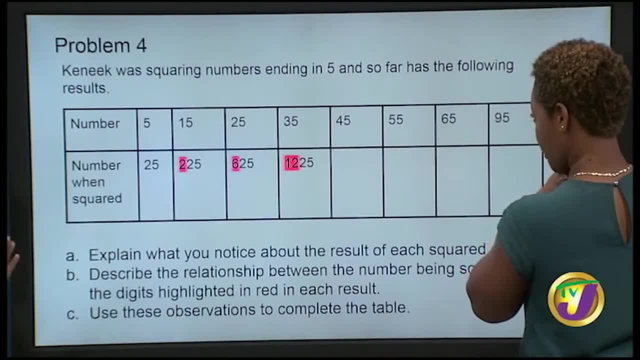 All right. So that must be: 3 times 4 is 12.. Great, So 5 times 4 is 5 times 4 is 20.. Good, But hold on. And then the 25. Hold on, Hold on, man. 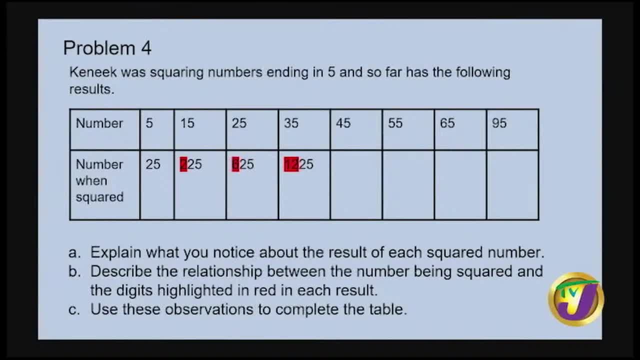 So you're getting it, But what you realize is: How, How, How, How, How, How. What you realize is happening with those numbers too. So you would have had 1. The numbers: It's increasing by one. 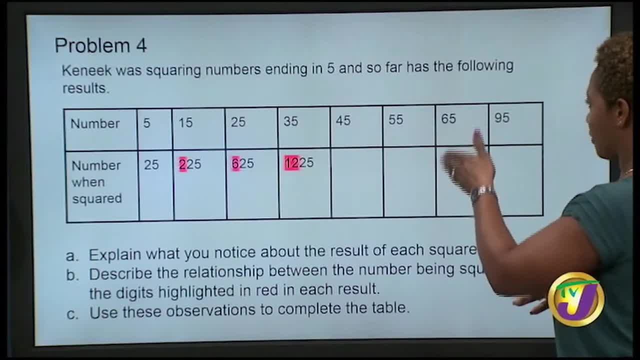 Great, Good job. Okay, So you realize that it's increasing. So you have 15.. So you have 10.. Then you have 20.. Pretty much I'm just looking at the tens place Yes, 1,, 2,, 3,, 4,, 5,, 6.. 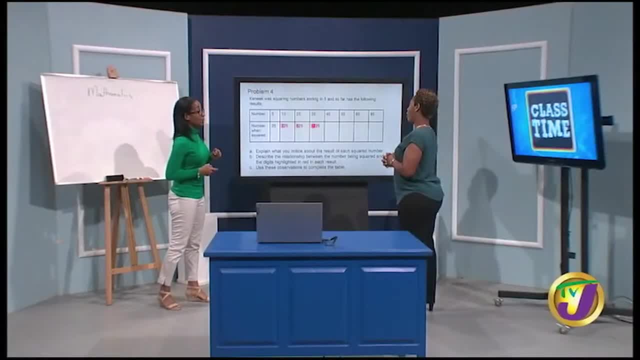 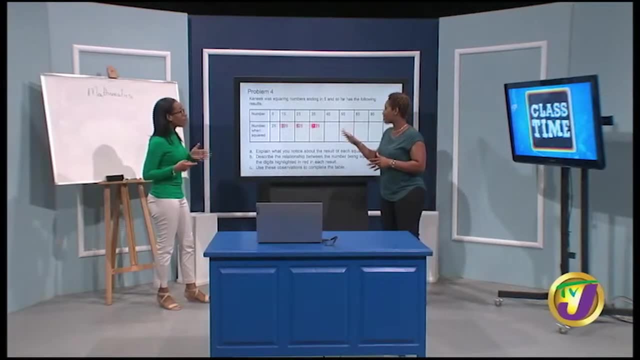 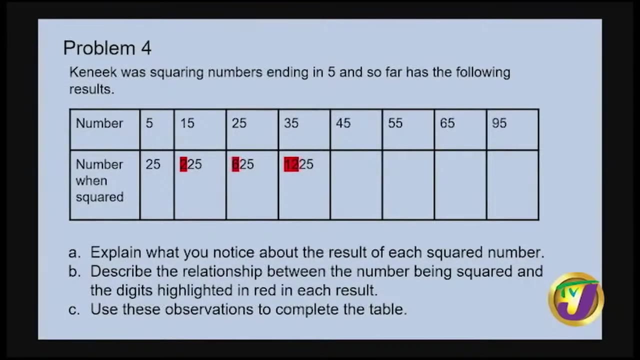 Yes, Great, Can you skip us some? Yeah, man, And that is why I needed you to complete the table. So, based on the relationship and the observations Okay That you would have, I can get this All right times. four is twelve, so this is the three four. oh, it says four, fours, four, fours, where you get. 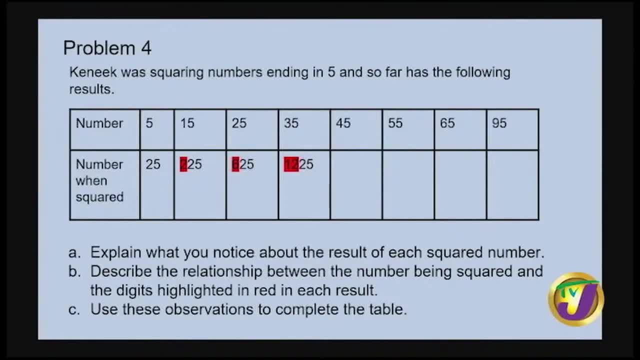 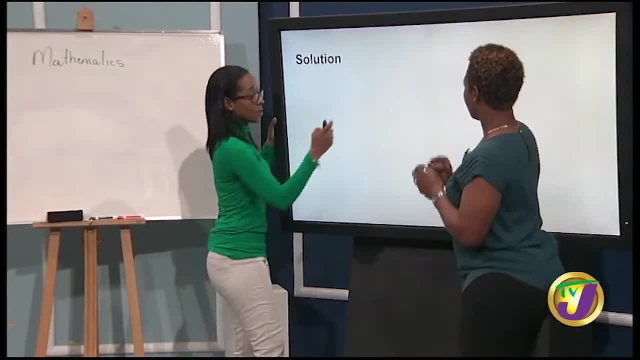 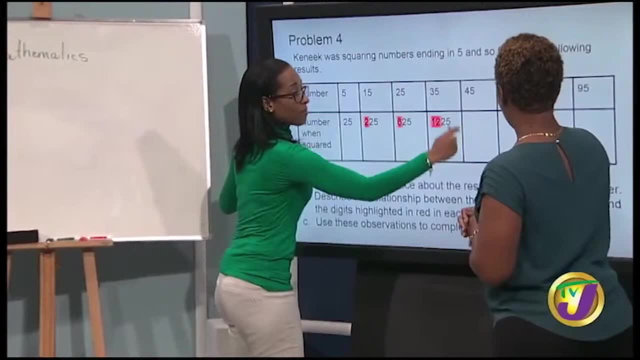 four, fours, that's three. yes, man. so this is one times two, one times. so. one times two give you two, good, right, okay. two times three gives me six, right. three times four gives me twelve. so how would you arrive right here now, instead of you running ahead, if you don't have a calculator? 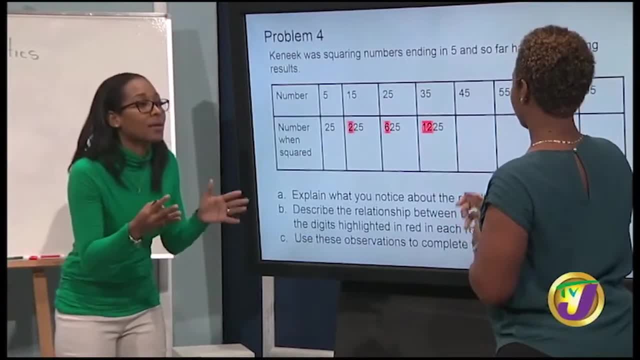 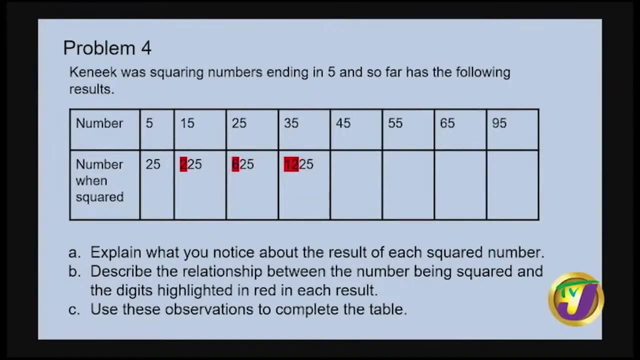 and you. you have to work this question out without a calculator. figure it out all right. so you go two times, i'll give you that that time. so three times four is twelve, says five times four times five gives me twenty. great, and what would be your last, remember you have to great. so 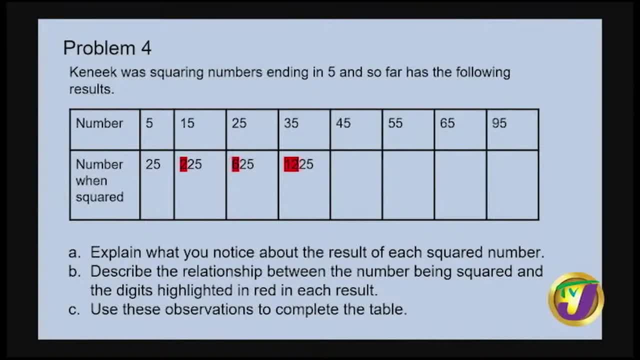 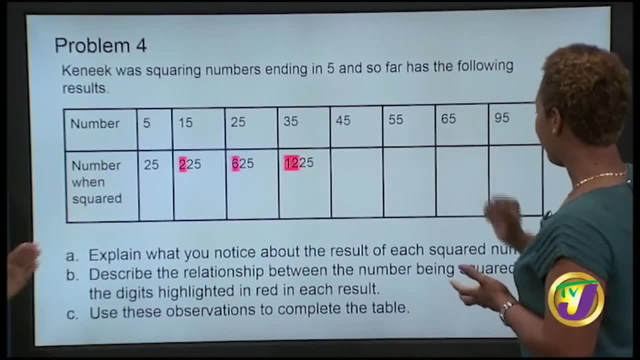 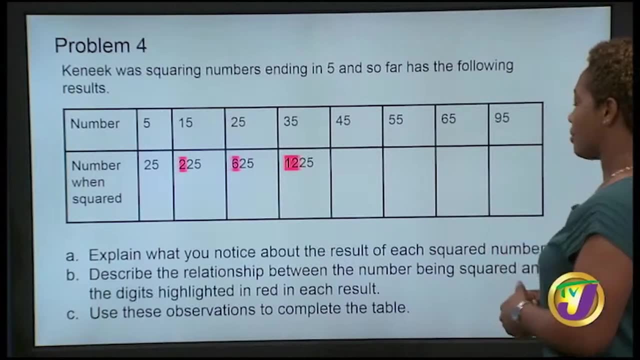 it's two thousand twenty five. good girl, what would be the next one? so two thousand twenty five. so when forty five is squared, five is thirty, right, and then you add the twenty five, so it's three thousand twenty five. all right, let me show you're going to do the next one now. 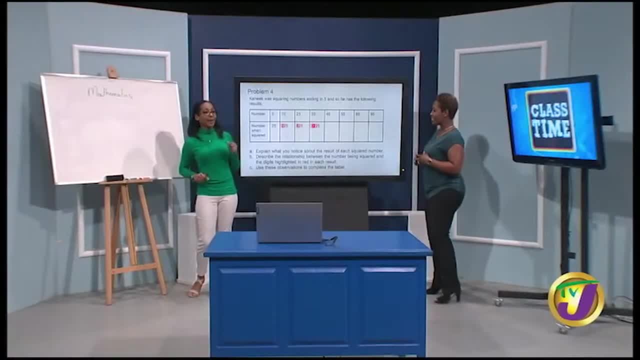 problem is there, but guess what? yeah, try to trick me, you know, guess what? so six would sixty, five would not be before ninety five. well man, five would be before it. i give in your head a little break. yeah, man, work it out yourself. i give you in your head a little break. oh geez, all right. 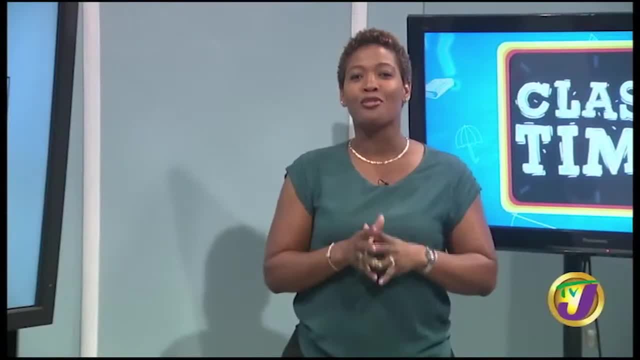 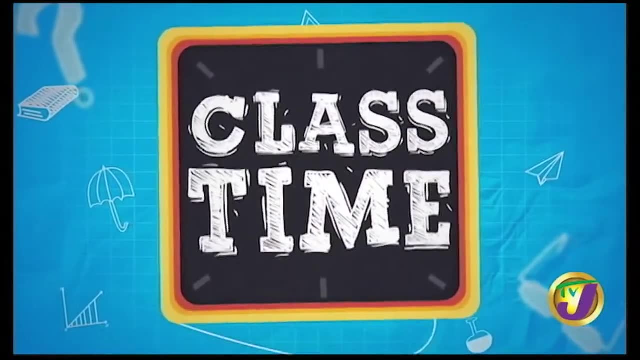 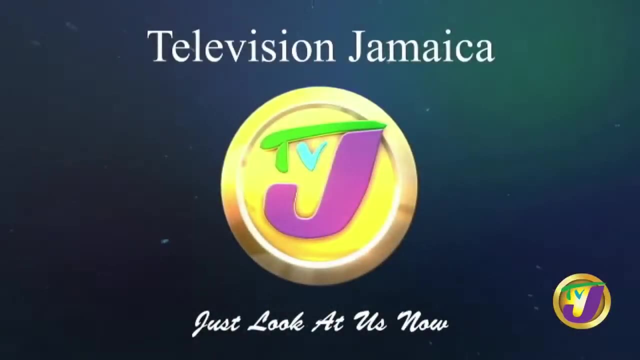 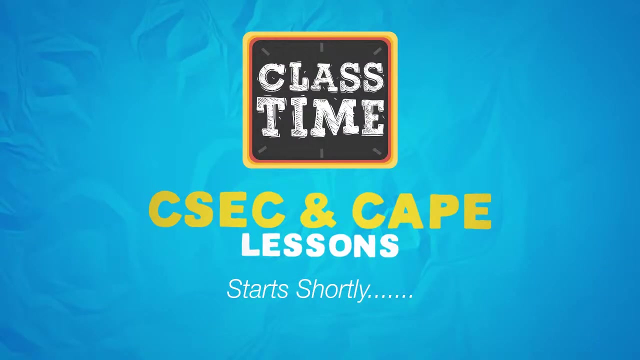 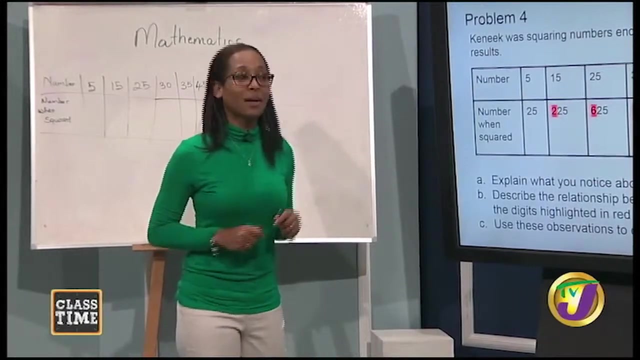 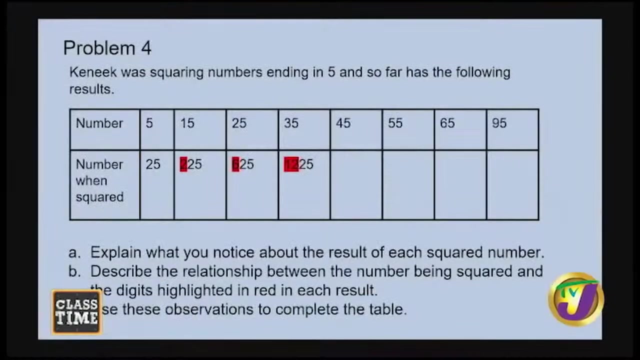 our second break is upon us. we'll be back to wrap things up after this. we'll see you next time. welcome back. let's pick up where we left off. so here we were. at kenny squared numbers ending in five, and so far he has the following results: now, tamika was trying to figure out, so she would have. 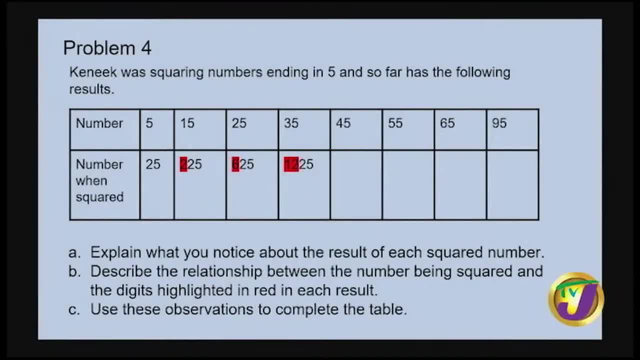 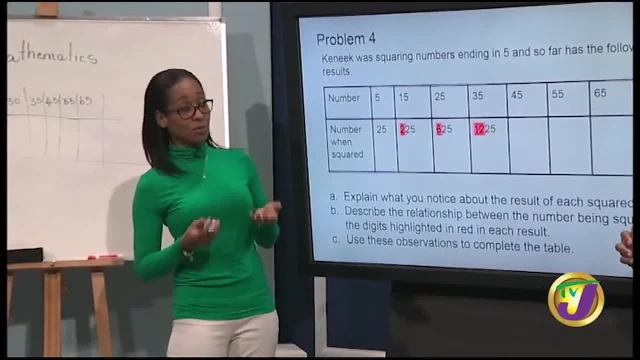 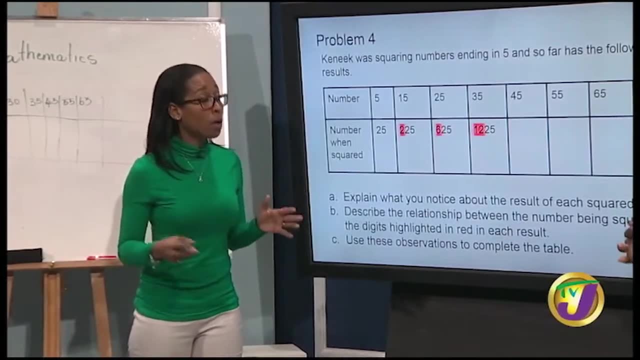 she would have figured out 45 when squared. but guess what? in the event, as i was reminding her and reminding our viewers before we left and we took the break, in the event, we don't have a calculator, okay, and we are squaring number, we need to figure out this table. so you worked out 45, you. 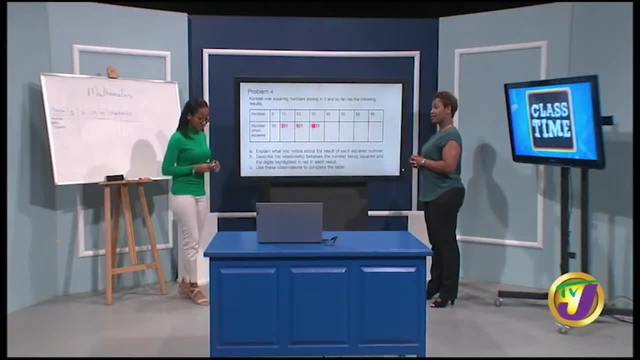 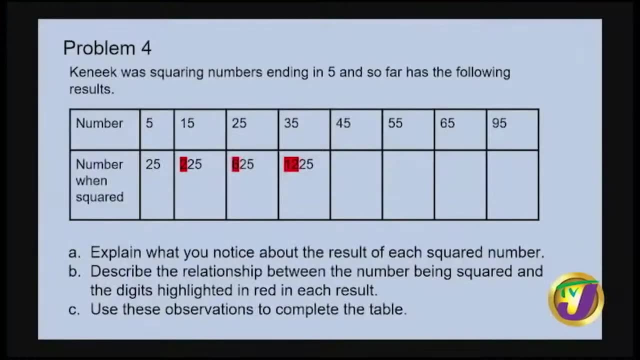 worked out 55. i did 65 too. all right, you did 65 as well. what did you get for 65? when squared, or looking at what you have here? never do it. so tell me no, man, tell me no. oh, so the next one would be. 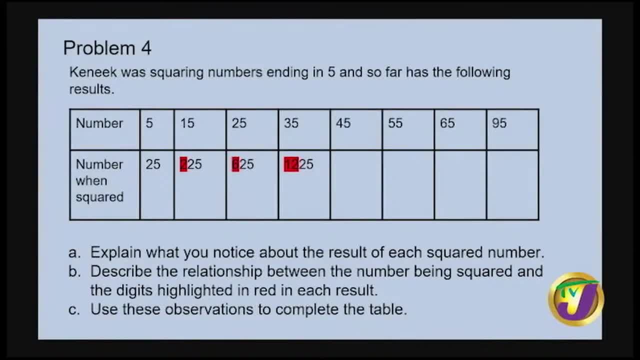 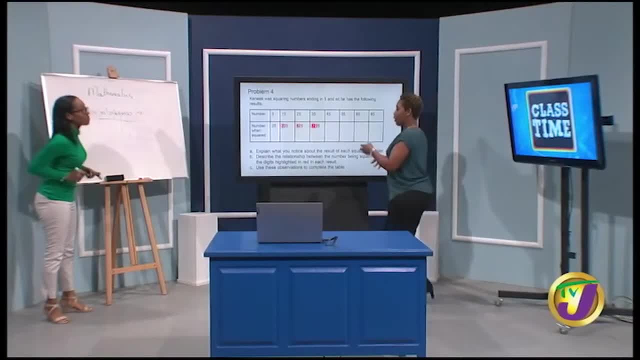 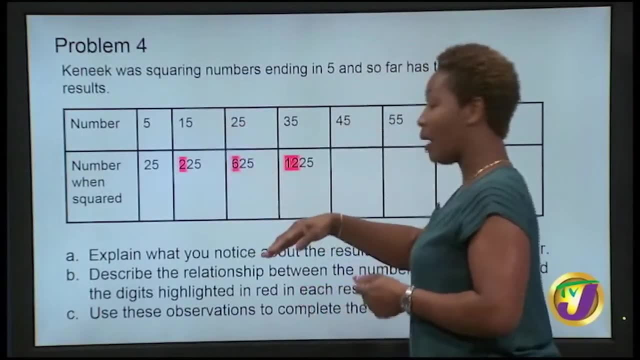 75.. so it would be 7. by how do you know that it would be 75.. i don't have 75 in my table. i want to answer for 65.. paying attention to the table, you would have added five to get 50. i mean 10.. okay then. 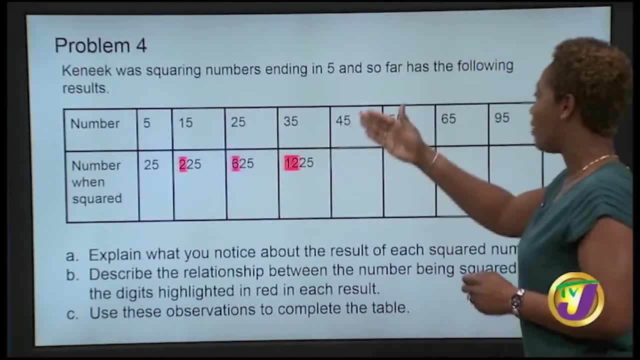 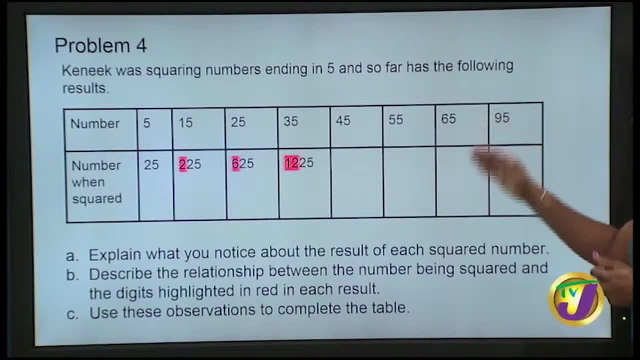 time to get 15, 10 to get 25.. anna, you keep on adding 10.. but you're trying to treat me and skip out some right. so the next one: if i added 10 to 65, i would get 75.. great, so we have so. 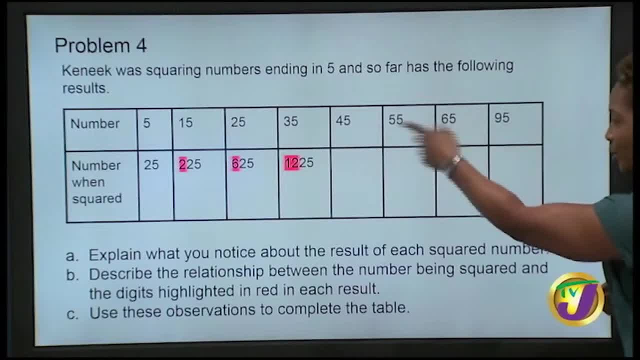 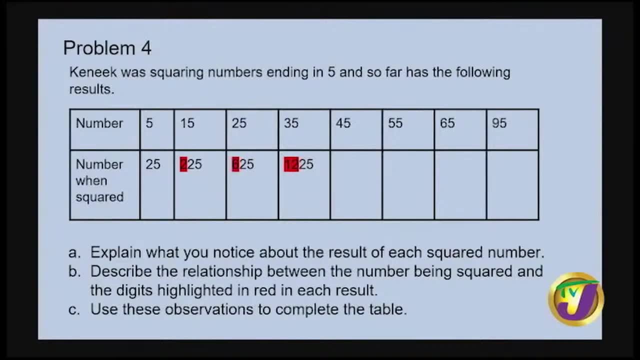 Some numbers missing from- And I have to make sure I'm paying attention- to continue what I did before. All right, So we know that that answer for 65 then Would be 7 multiplied by 6.. So I'm multiplying the digits in the 10th place. 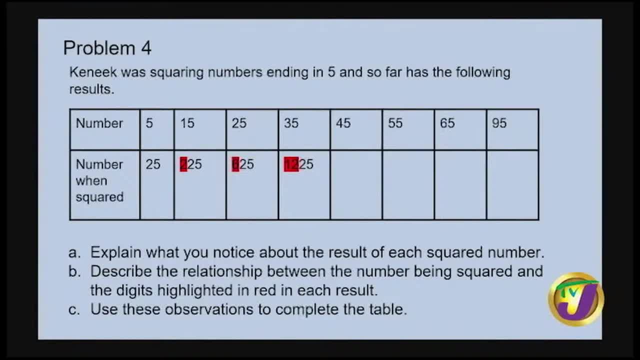 All right. So 7 times 6 is 42.. And then I put on the 25.. All right, So 4,225.. You're not tricking me. All right, We're going to see. The next one is 95.. 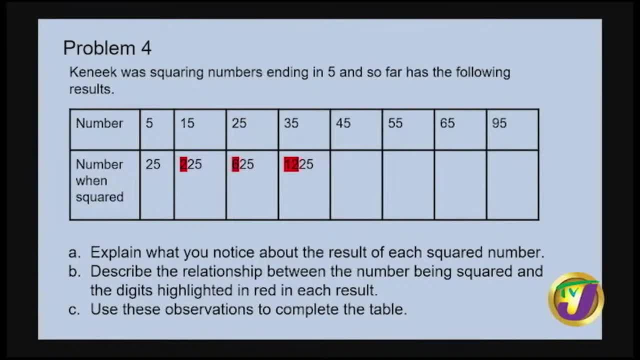 So figure it out, Let's see if you get it. So what would What is, What would you do? Hmm, You see, I can't trick you. All right, What? is a pity they can't see your face, you know. 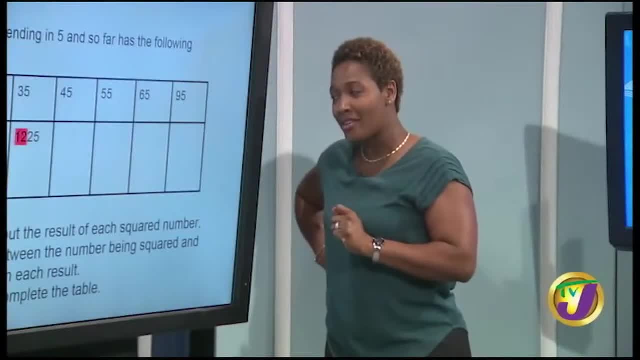 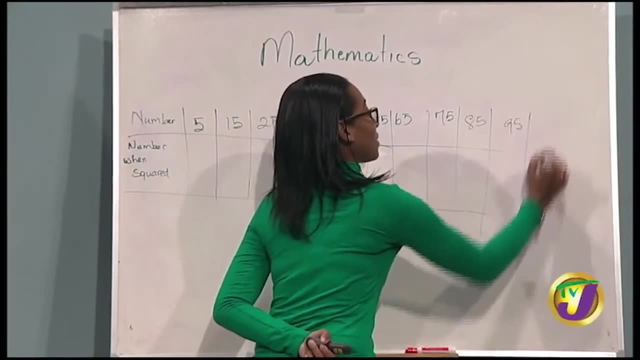 Well, the next one: if I added 10 to 95, that would be 105.. Okay, You're paying attention, 105.. So we would have had 85 missing, 95 missing and we would have had 105.. 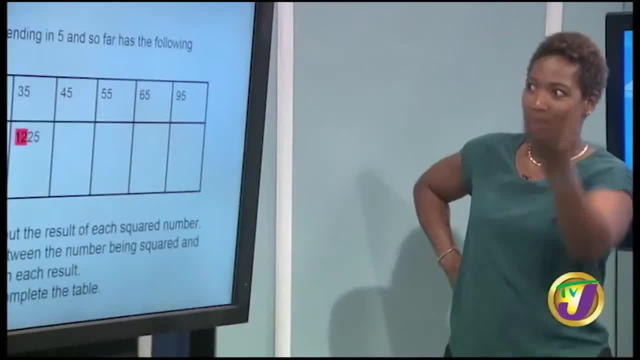 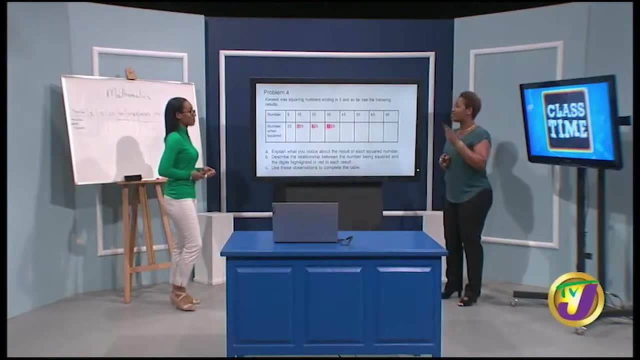 So I definitely need the number that comes after to work out the previous. Oh jeez, Correct. Okay, All right, So it would be 10 multiplied by 9.. All right, Which is 95.. 90.. 90.. 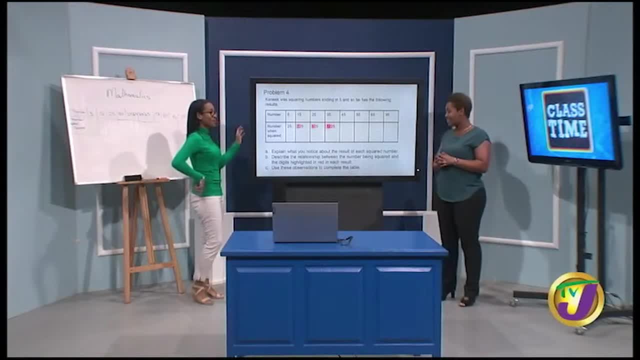 You're sure You're sure it's 90? 90. It's 90. I'm sure You're sure it's 90. So the answer is just 90. 90. And then I add on a 25,. 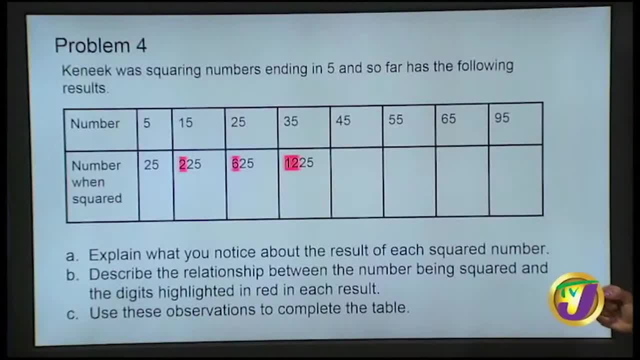 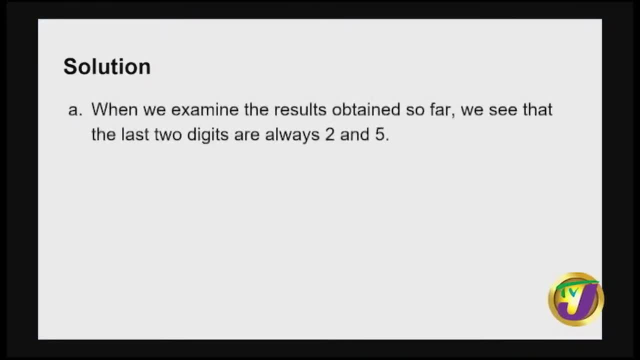 so it's 9,025.. All right, I got this. You got this, So let's check. if you are indeed correct, So you would have answered A. when we examined the results so far, We see that the last two digits are always 2 and 5, 25.. 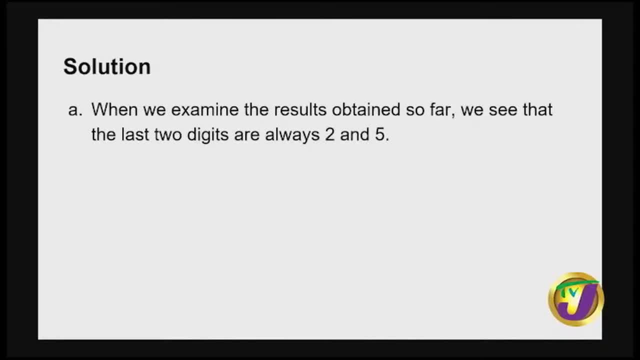 And remember we were squaring the numbers and we were looking at numbers ending in 5. Right, Right, So you would have also looked when you looked at the table, for each of the numbers being squared, the first digit is multiplied by that. 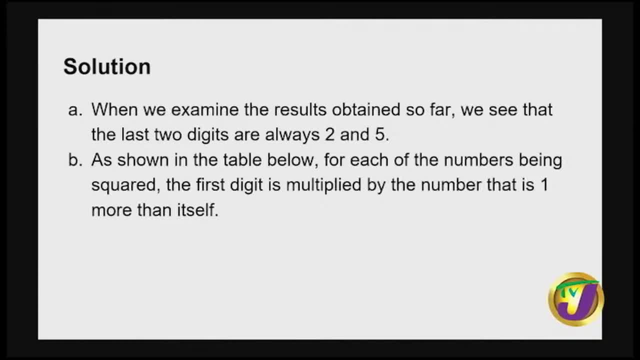 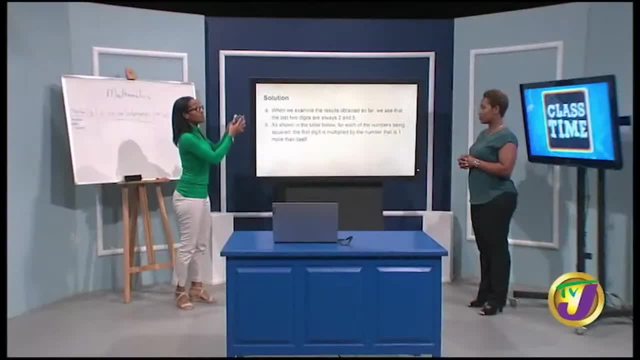 That is one more. So when you would have multiplied 1 times 2, you would have looked at your tens column there. yes, But it would have still been one more, because when you realize that, hey, you have 65, and I jumped to 95.. 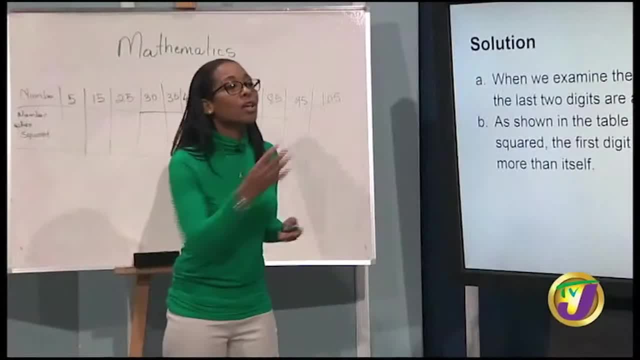 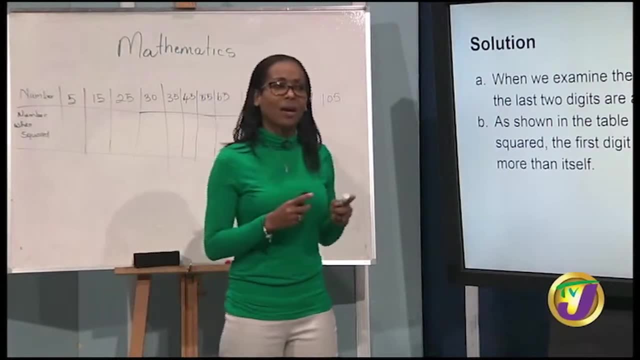 Can't work it. you realize what took place, But you didn't tell me what you used to figure this one out. So after a while, it took you a while to understand the problem. Oh, of course it did. I hope you understand the problem now. 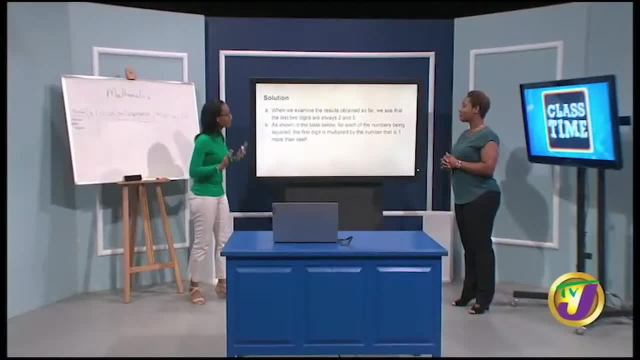 And it's fine. It's fine. I understood. in the end, You understood Great. So, in understanding, what did you do to understand it? now I looked for the pattern because you were trying to trick me. No, I wasn't trying to trick you. 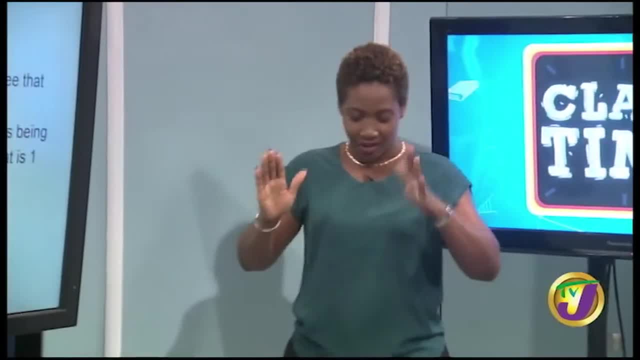 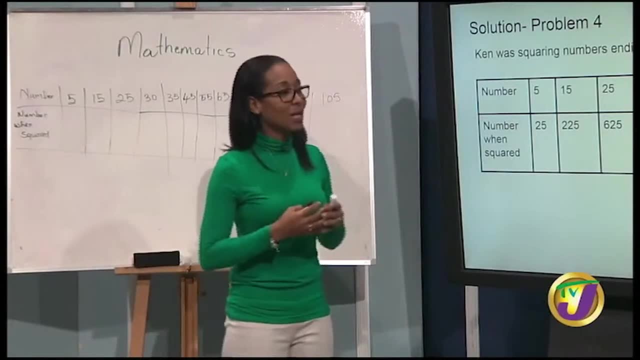 I looked for the pattern, There was a pattern, There was a pattern and I saw it. All right, You saw it. You looked at the observations that were taking place and you would have looked at the relationship. So this would have been your solution. 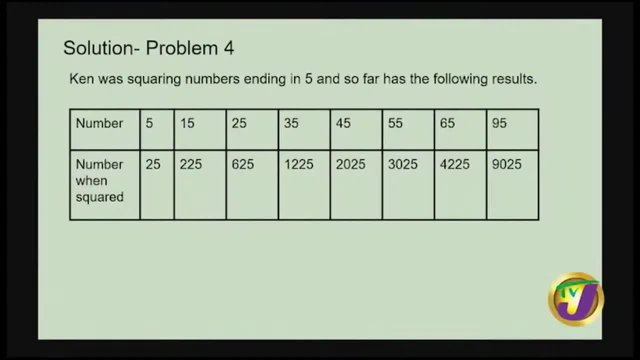 So you are indeed correct, I got it, And you would have helped connect the square, the numbers ending in five. So good job, You get it. So we are hoping that our viewers at home have gotten it as well. Yes, let me see. 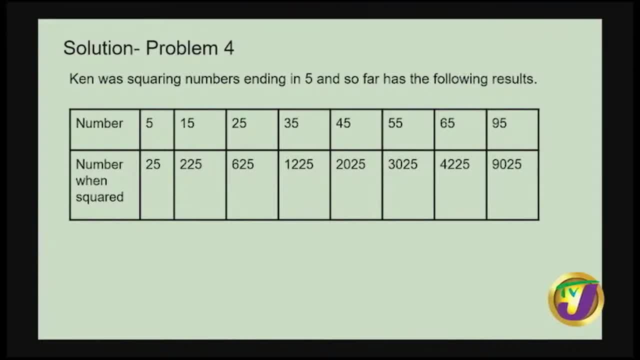 All of them end with two, five. Yep, I did it, See, So we're proving it now. So, all of them ending with over two, five, over 25, we're realizing And in getting the first digit here, 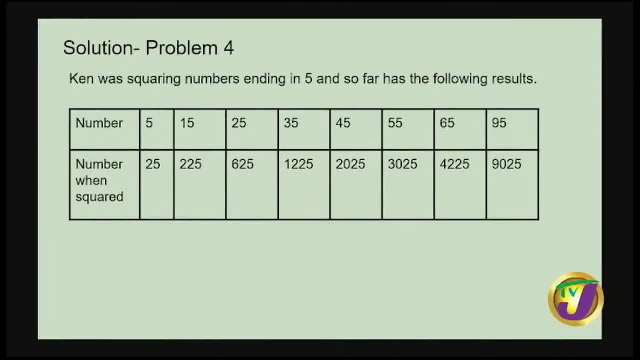 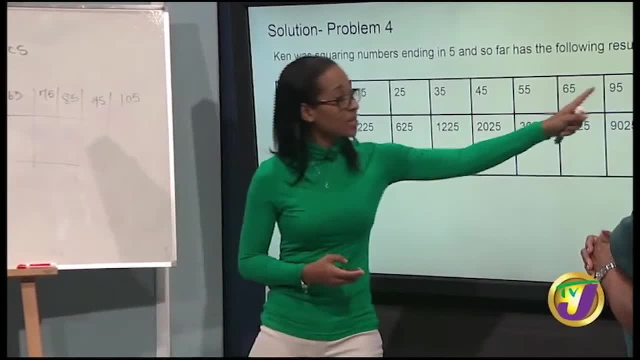 no, so it's one times two, two, Two times three, six, Three times Three times Five, Four, Four or 12.. So three times four is 12.. But watch me, you know, six times nine. 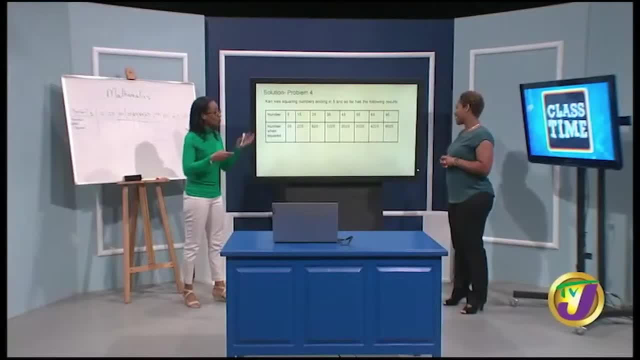 Six times seven, Okay, Okay. So those two numbers there, the 75, 85, would have been missing, as well as over 100.. So key point note: pay attention to the progression, Even when you do identify a person if they're missing values. 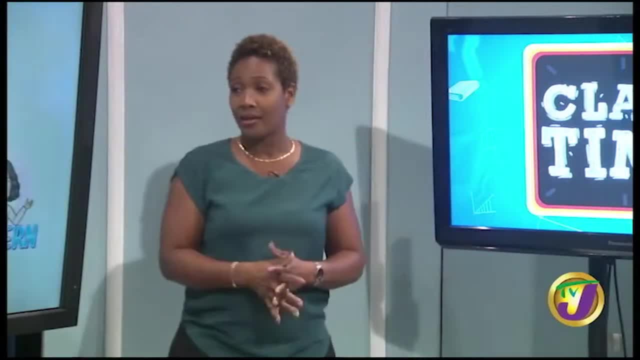 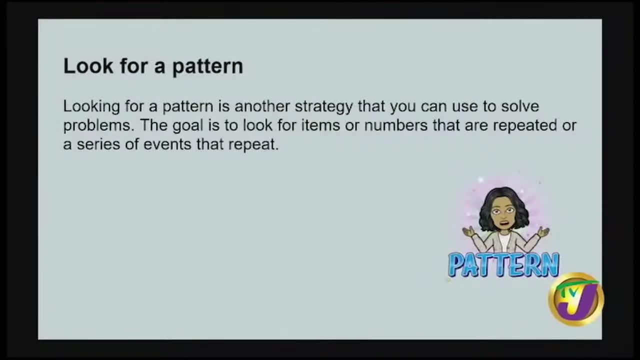 you can get one that's not correct, All right. So we did look at a pattern, and it's another strategy that you can use to solve problems. The goal is to look for items or numbers that are repeated, or a series of events that repeat. 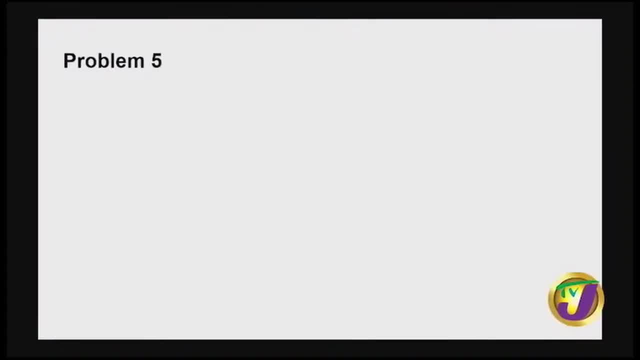 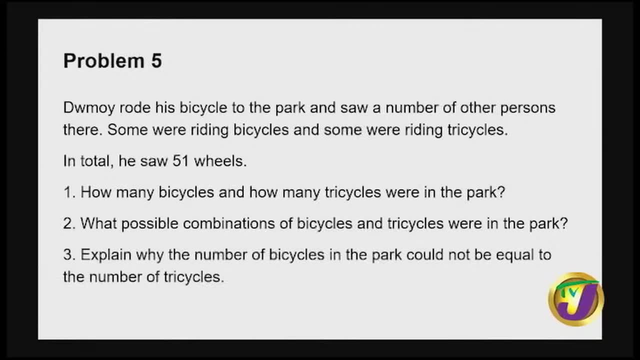 And guess what? We need them to try this one at home. So we're just reading it for them And we want them to try it at home, to screenshot it now and try it at home. So Dumoy rode his bicycle to the park. 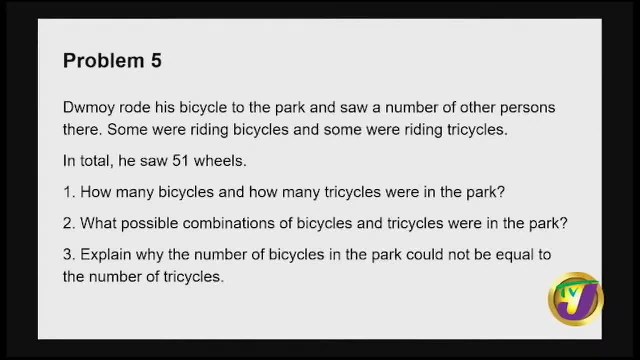 and he saw a number of other persons there. Some were riding bicycles and some were riding tricycles. In total, he saw 51 wheels. One: How many bicycles and how many tricycles were in the park? Two: What possible combinations of bicycles? 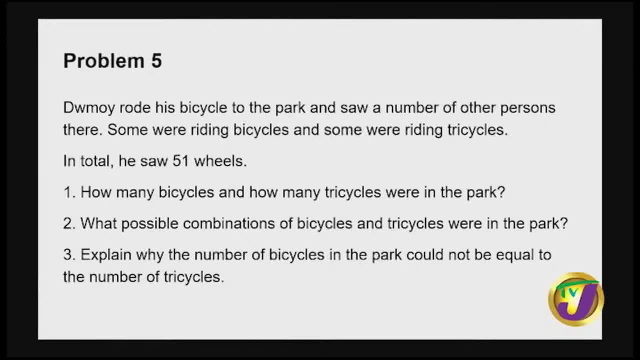 and tricycles were in the park, And three Explain why the number of bicycles in the park could not be equal to the number of tricycles. So it's important here for Dumoy to know that 51 wheels and what we know about a bicycle. 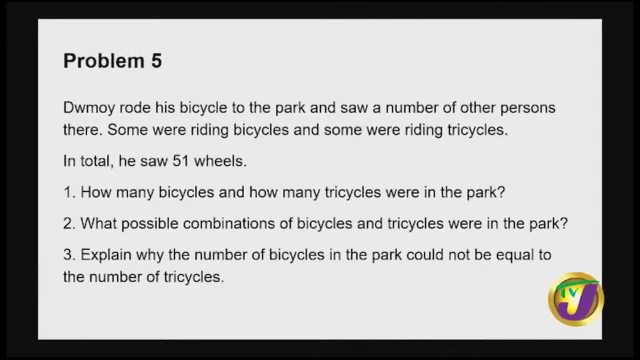 Two wheels- Great. What we know about a tricycle: Usually three wheels, Usually three, Three wheels- good. So three wheels for a tricycle and two wheels for a bicycle. So those are important information And you have to account for both tricycle and bicycle. 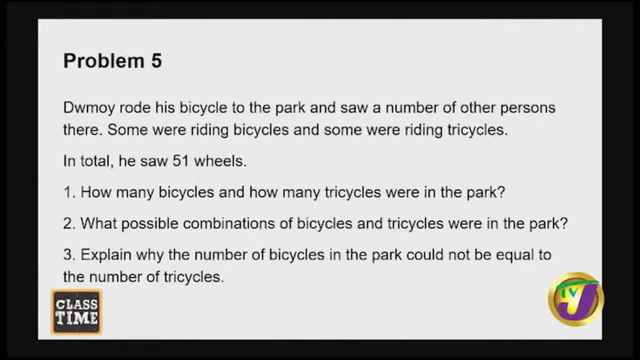 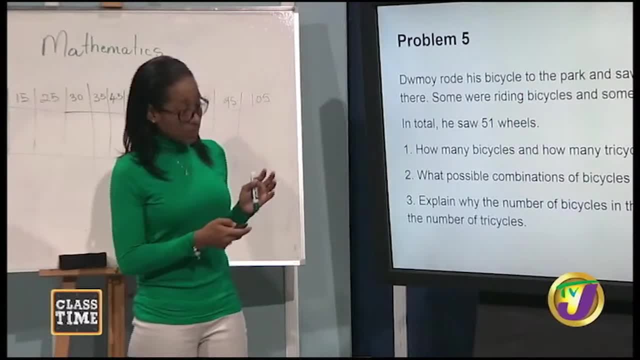 Great, So he needs to figure this out And we're hoping that you would have screenshot this for you to try at home. Yes, All right Now. we would have looked at some strategies so far, So we're just recapping our strategies here. 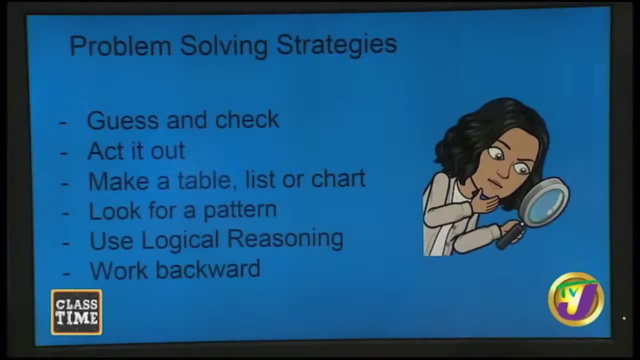 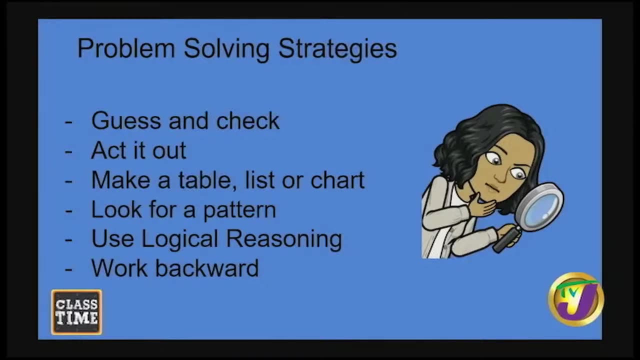 Guess and check was one of them we looked at. We didn't get a chance to look at Actito, but that's another problem-solving strategy We looked at. make a table list or chart, look for a pattern, use logical reasoning. 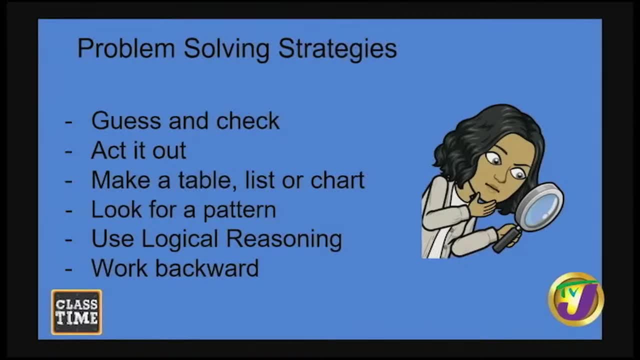 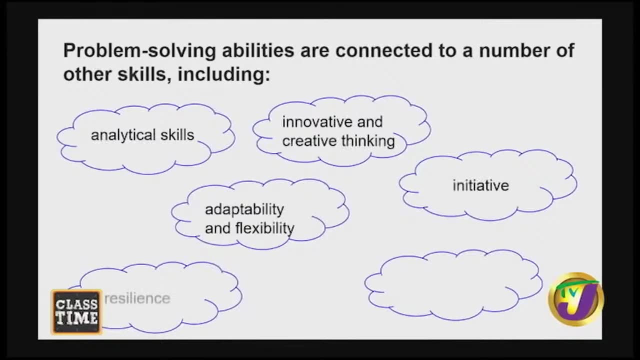 and we work backwards. So these are problem-solving strategies, And problem-solving abilities are connected to a number of other skills, including analytical skills, innovative and creative thinking, adaptability and flexibility, initiative, a lateral mindset and resilience. All right,